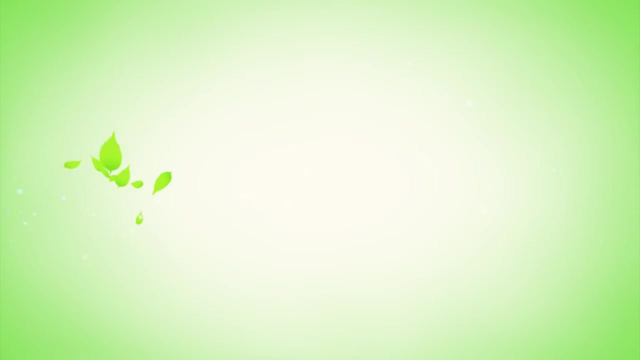 Today we're going to talk about methods for measuring hydraulic conductivity. So here's a brief outline of our presentation. First, we're going to talk about what is hydraulic conductivity and why is it important. We're going to go into some different measurement methods for saturated and unsaturated hydraulic conductivity. We'll cover both field and 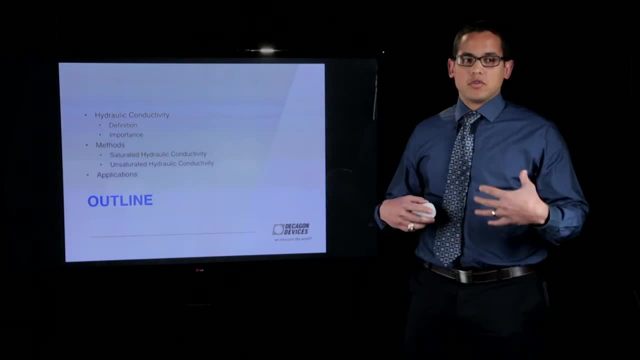 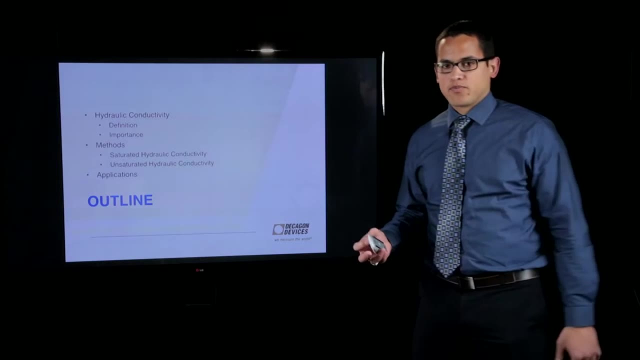 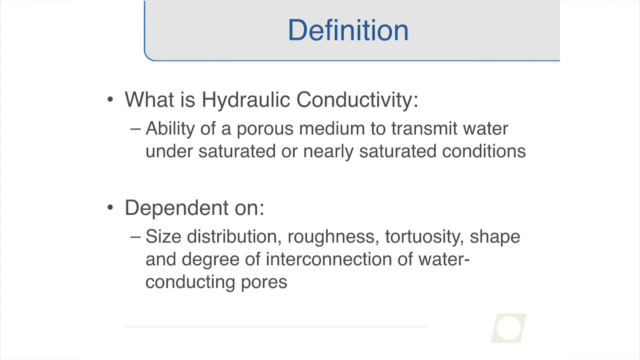 laboratory techniques. We will also then go into a couple of applications of hydraulic conductivity and show how it's been used and how it's been helpful. So, first off, what is hydraulic conductivity? Hydraulic conductivity is the ability of a porous medium, for example. 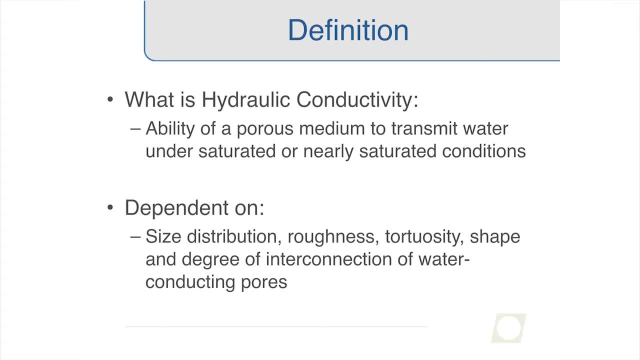 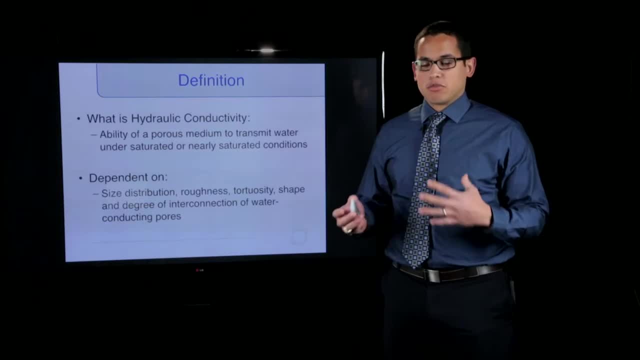 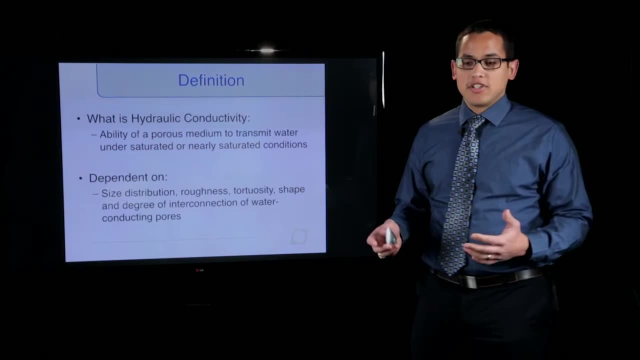 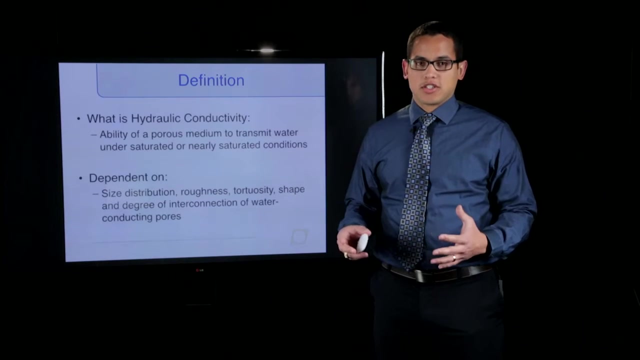 soil to transmit water under saturated or nearly saturated conditions. Now, hydraulic conductivity is dependent on some different factors. Some of those factors are size, distribution, roughness, tortuosity, shape and degree of interconnection of water conducting pores. Now, one of those things that can often affect hydraulic conductivity is soil structure and 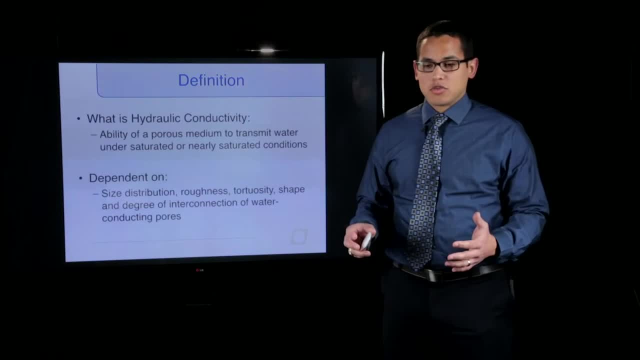 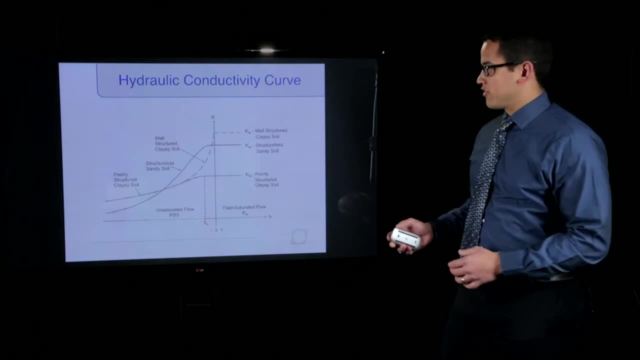 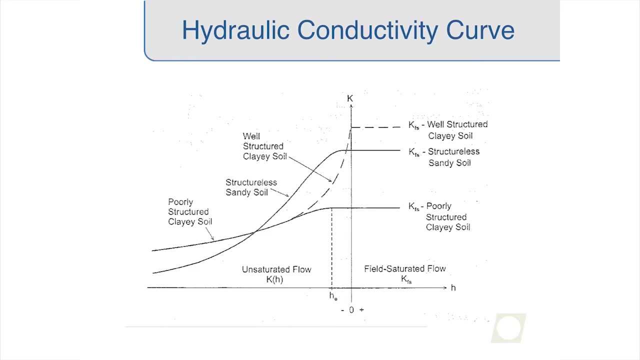 how strong the structure is in that soil you're measuring. So here's an example of a hydraulic conductivity curve for three different soil types. One is a well-structured clayey soil, the other is a structureless sandy soil and the third one is a poorly structured clayey. 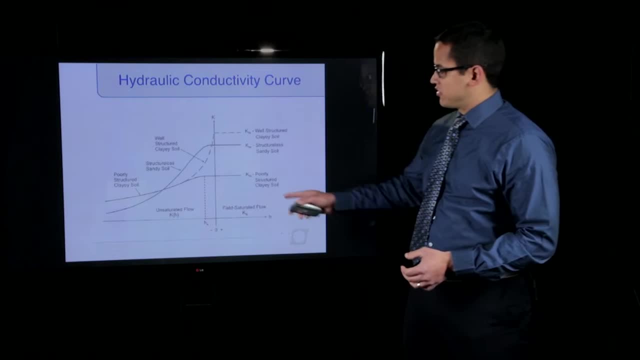 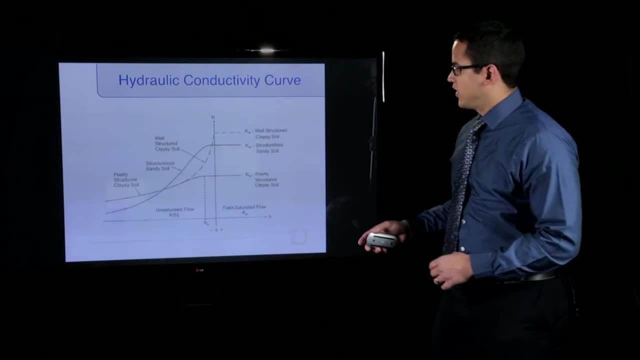 soil. So here's some interesting things to point out. This is the curve starting from field saturation and going into the unsaturated hydraulic conductivity portion of the curve, And I think the most important thing here is the difference that you get from a well-structured 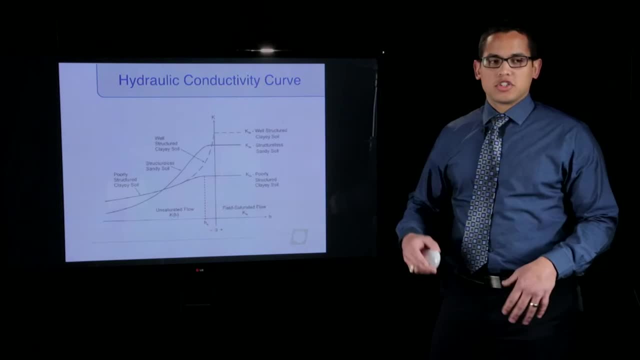 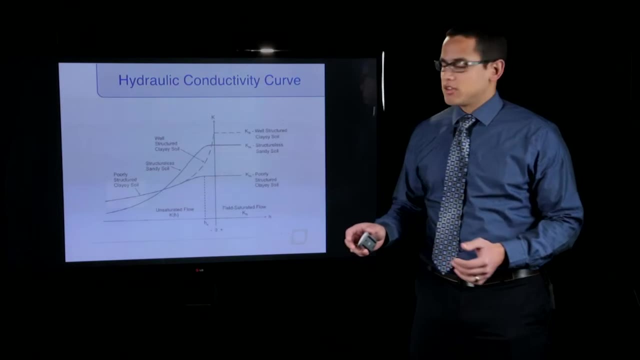 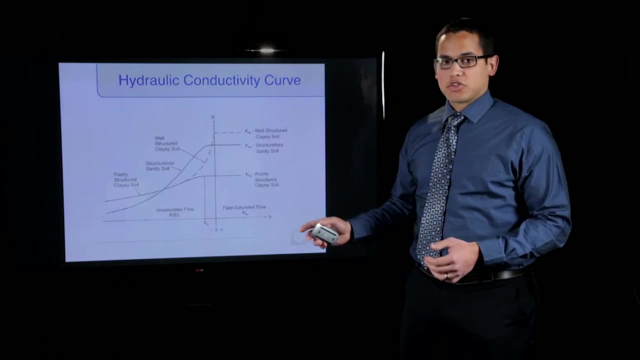 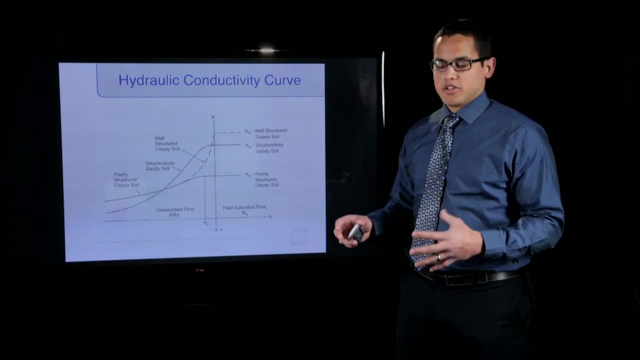 clayey soil to a poorly structured clayey soil And what this shows is the importance of structure in hydraulic conductivity, especially at or near saturation. And you can see that this well-structured clayey soil actually has a higher saturated or field saturated- hydraulic conductivity than the structureless sandy soil. And that is in part due to the 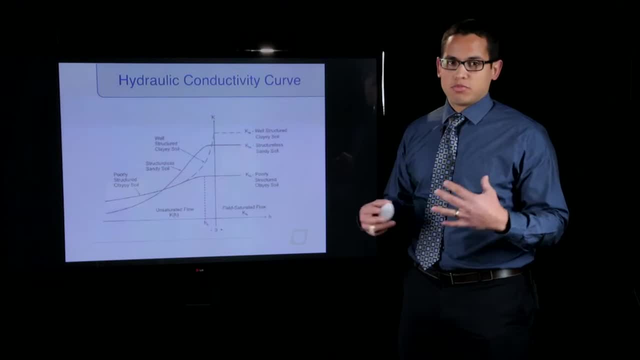 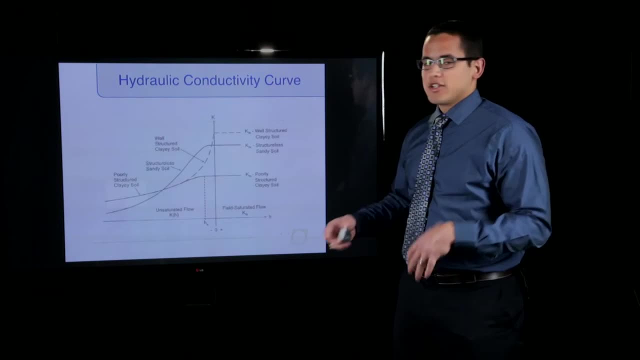 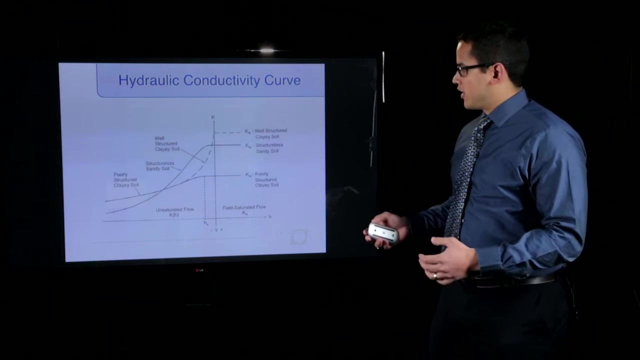 strong structure which creates larger macros, The macropores, and just better flow paths for water and soil. And then when you go, look at this poorly structured clayey soil, it has very low hydraulic conductivity, mostly small pores that are transmitting water and more restricted. 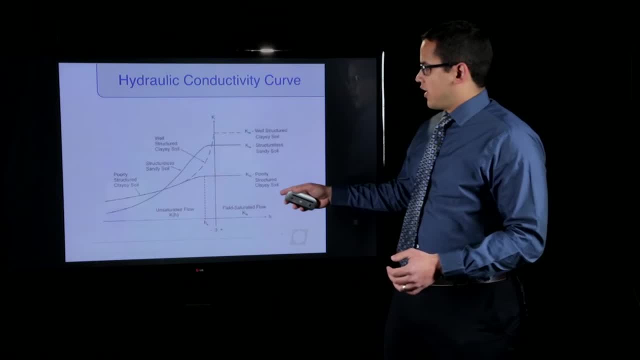 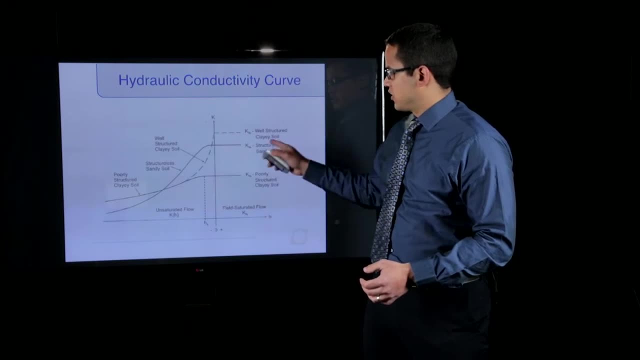 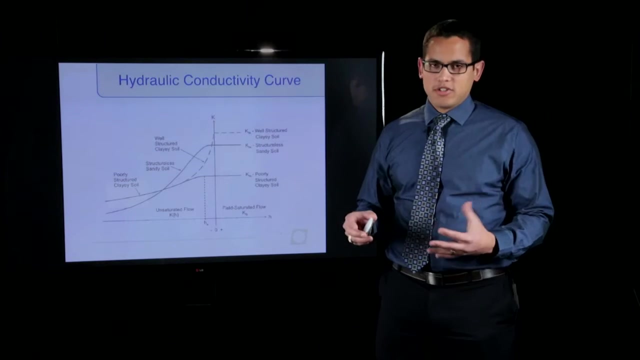 The other important thing to point out in this is: eventually the unsaturated hydraulic conductivity for the poorly structured clayey soil and the well-structured clayey soil eventually meet up, And what this is showing is that at a certain point, the macropores stop contributing to. 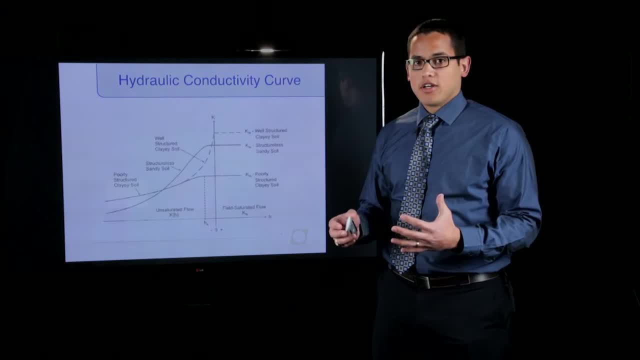 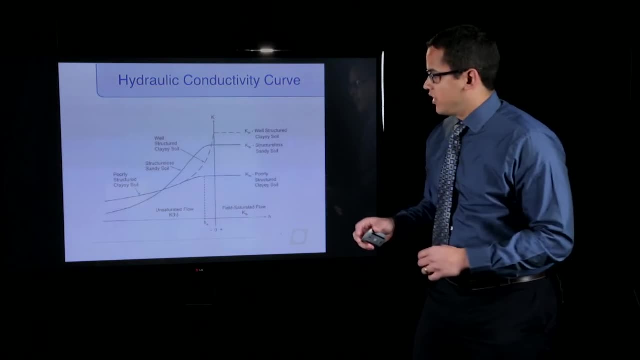 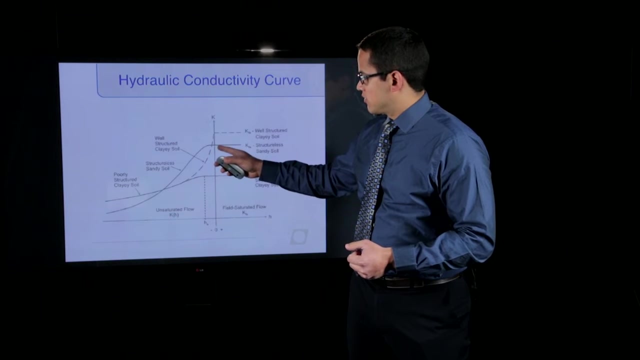 the flow and then it's purely back within the mesopores of the soil and actually just the fine pores between the soil particles. And I think another interesting thing to point out is the unsaturated hydraulic conductivity curve, for the structureless sandy soil starts out higher than the highly structured clayey. 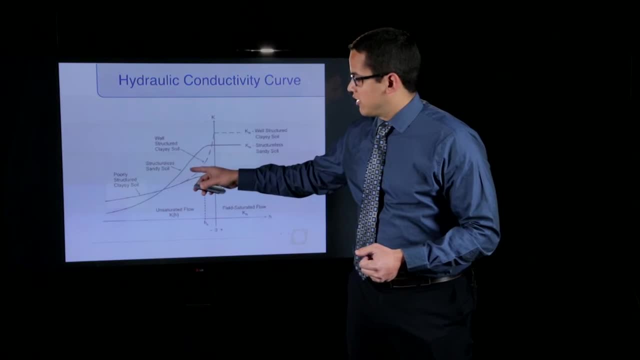 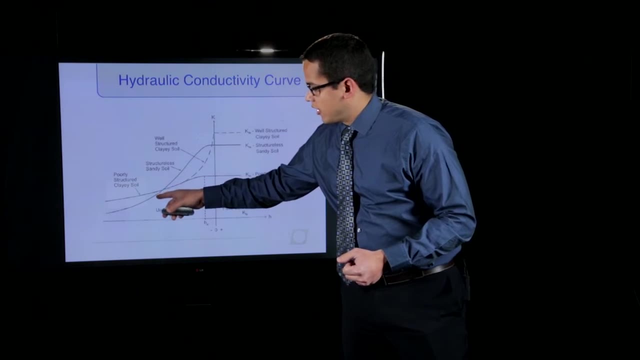 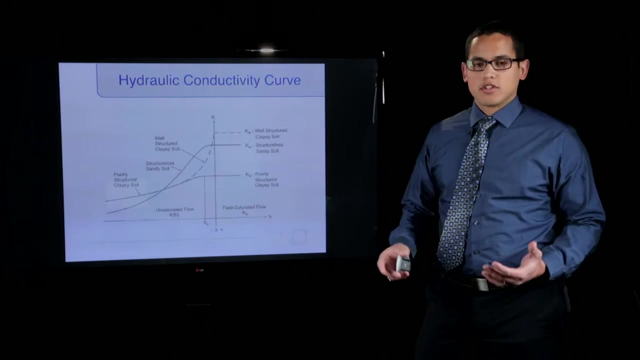 soil, the clay soil. but as the water potential decreases or as the soil gets drier, the unsaturated hydraulic conductivity actually goes lower than the hydraulic conductivity of the clay soils. So why do we even care about hydraulic conductivity? What do we use it for and why is? 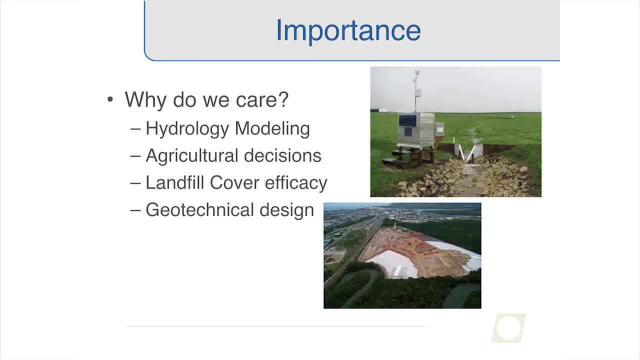 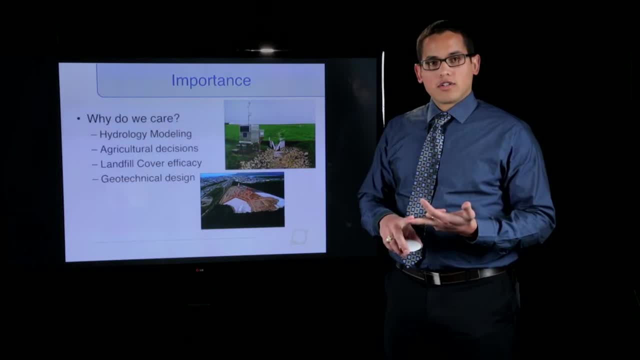 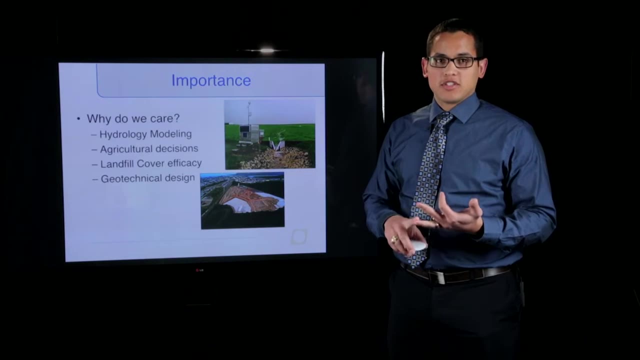 it important. Well, one of the common applications of hydraulic conductivity and those values is for hydrology modeling. So people are modeling runoff, modeling water tables and groundwater flow and also just modeling water flow in the unsaturated zone or in the beta zone. 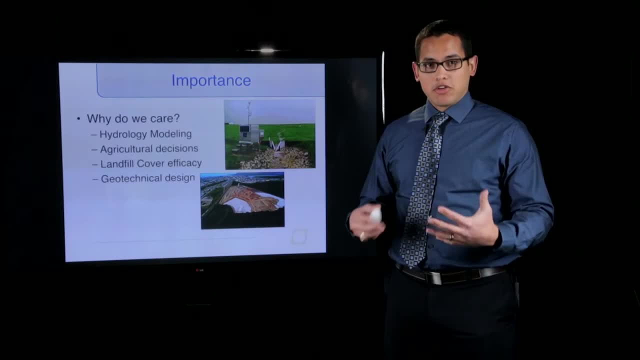 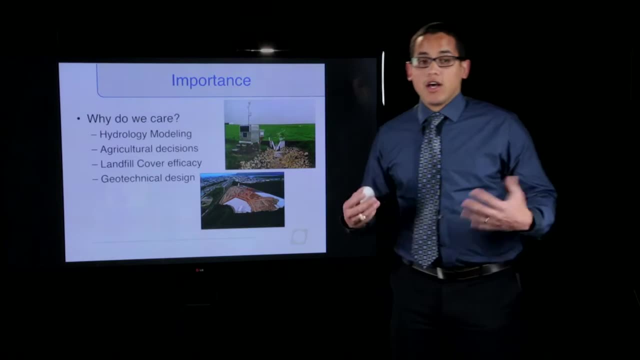 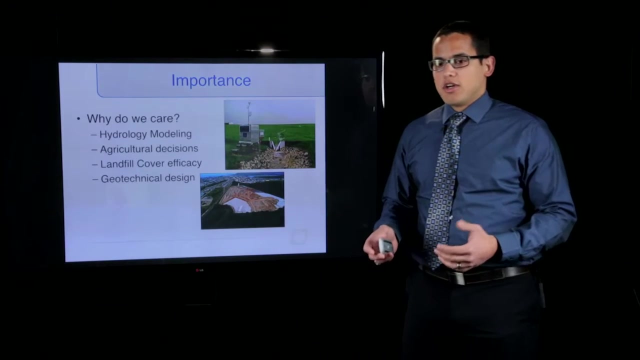 We need these hydraulic conductivity values to be able to accurately model how water is going to flow through soil and in different field sites. So another important factor for why we need hydraulic conductivity is basing agricultural decisions, whether we're doing trying to determine irrigation rates. 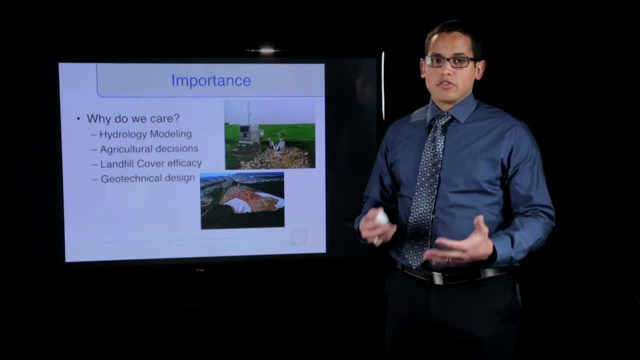 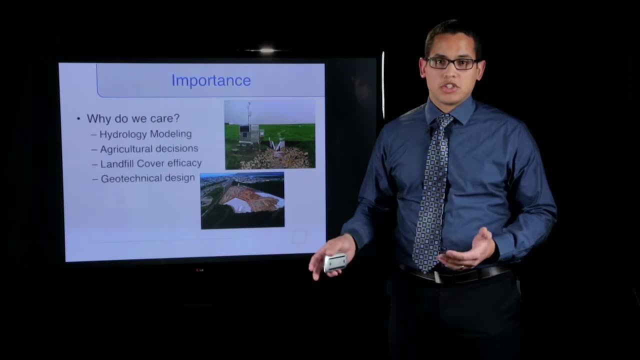 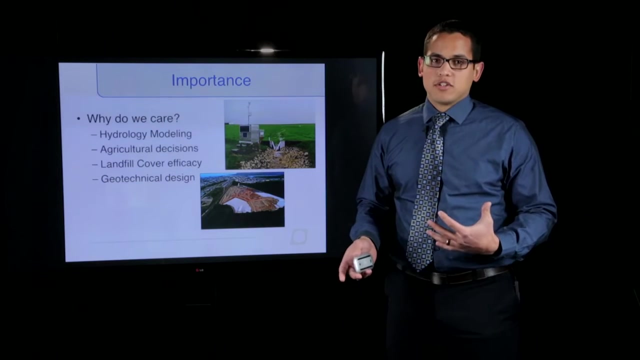 potential for leaching those types of things. We don't want to over irrigate soil and cause water to pond and potentially runoff because one that's a waste. It's also a potential for erosion, which could cause loss of fertilizers and those types of things, So it's important. 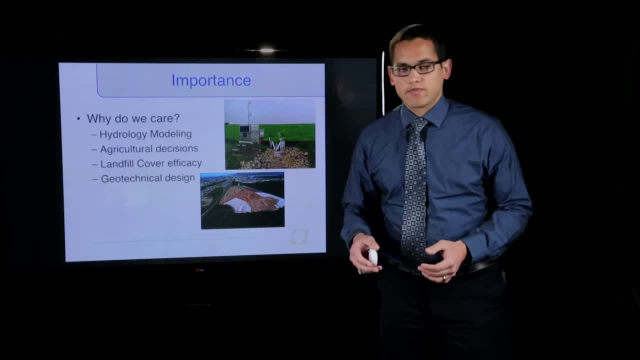 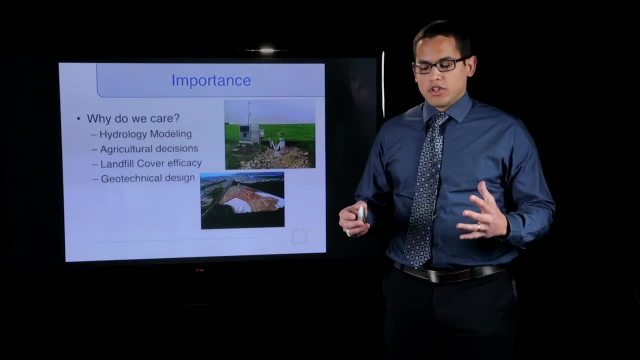 that we understand the actual ability of the soil to transmit water. A third thing is landfill cover efficacy. When people are, when designers are designing landfill covers and wanting to make sure that they're actually doing what they're supposed to do, typically, the goal is that they have a very low hydraulic conductivity. 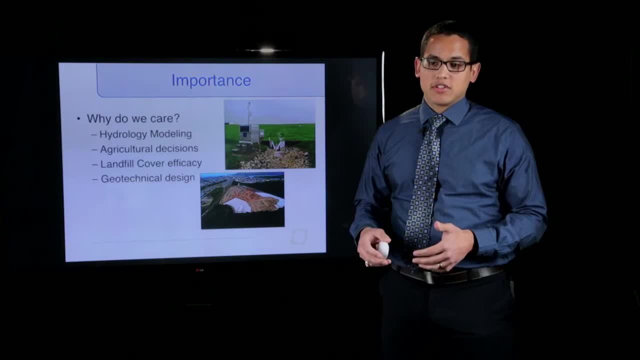 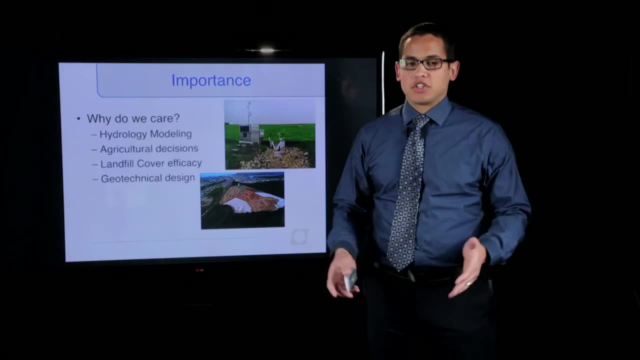 And that is to prevent water from infiltrating into the landfills, potentially then carrying the contaminants from the landfill deeper and potentially into the landfill. So that's a big thing, So that's a big thing. So they're also very concerned about the possibility of water coming into the ground water and causing those types of issues. 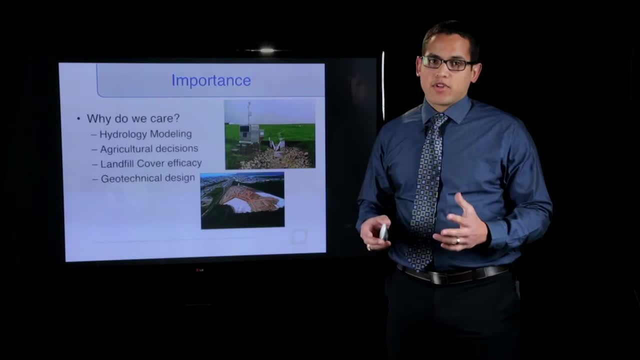 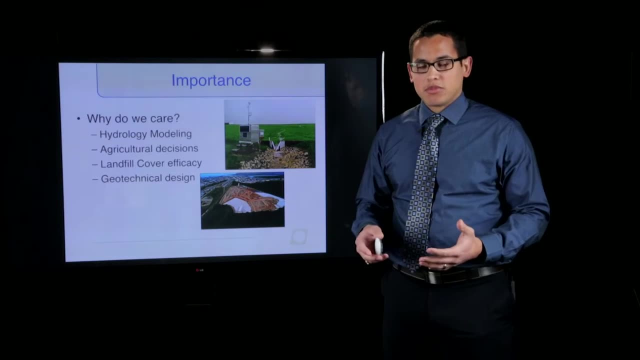 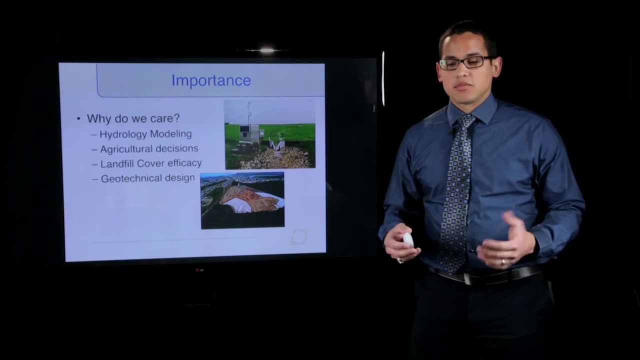 So they are often measuring landfill covers, whether it be clay caps or alternative covers, to make sure that they're actually transmitting water how they would want them to. And a fourth thing is in geotechnical design, Whether we're designing retention ponds or or road beds or other other systems. 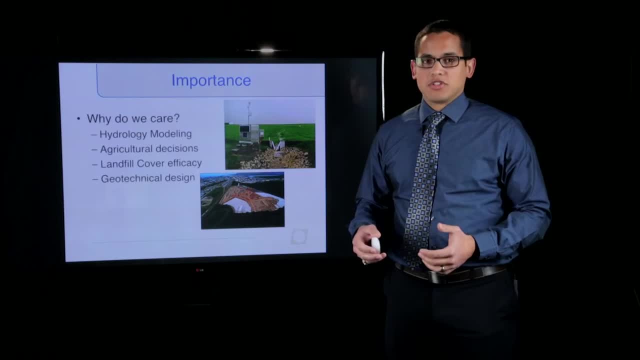 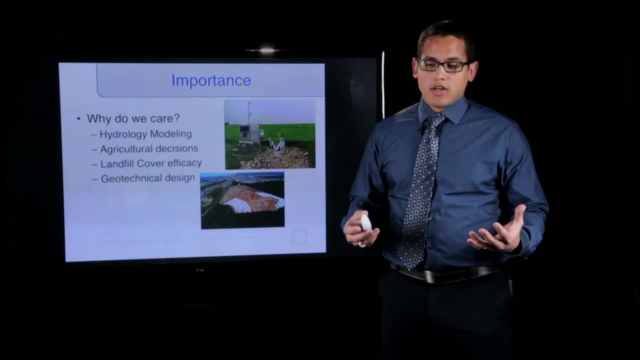 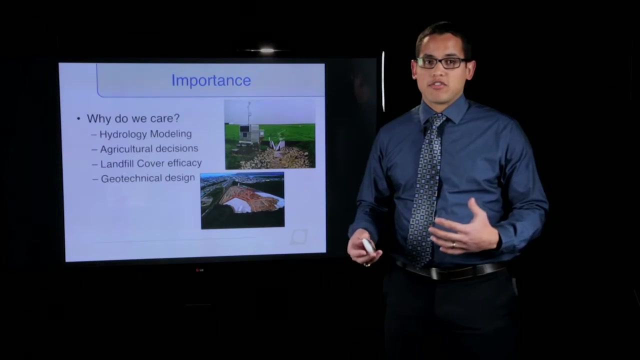 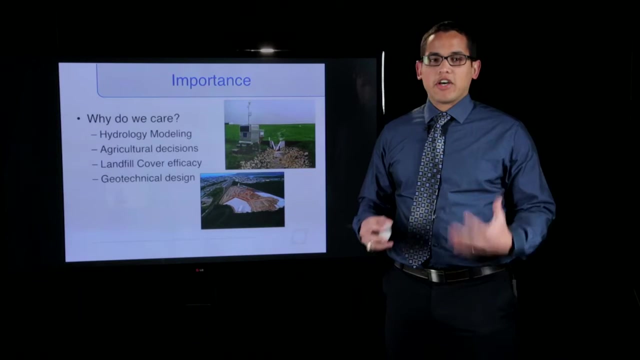 geotechnical engineers also need a lot of ground water measurements of hydraulic conductivity to base their decisions, whether it be sizing a retention pond or designing rain gardens- those types of things that are designed to capture runoff from parking lots and other impervious services- So it's a value that's important in all of these. 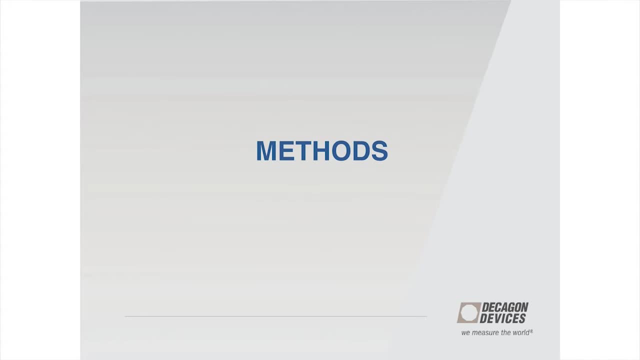 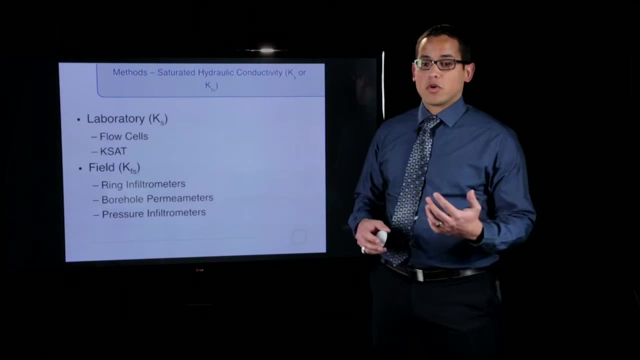 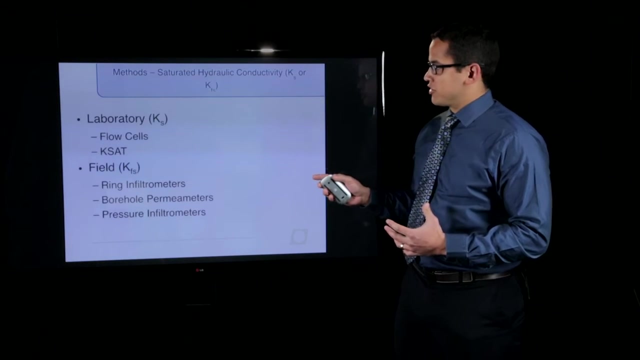 areas. So next we'll go into some methods for measuring hydraulic conductivity. So first let's focus on measuring saturated hydraulic conductivity- KS or KFS- And the reason we have two different designations, KS and KFS, is in the lab, when we're measuring saturated hydraulic. 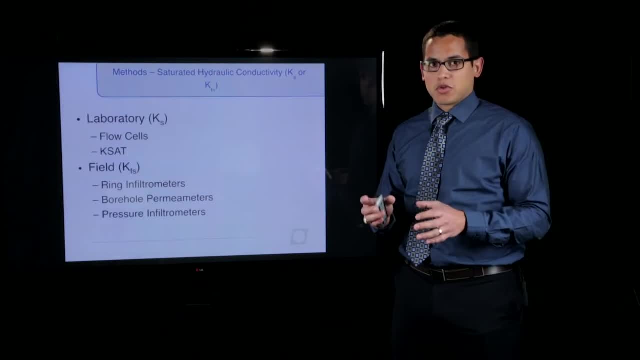 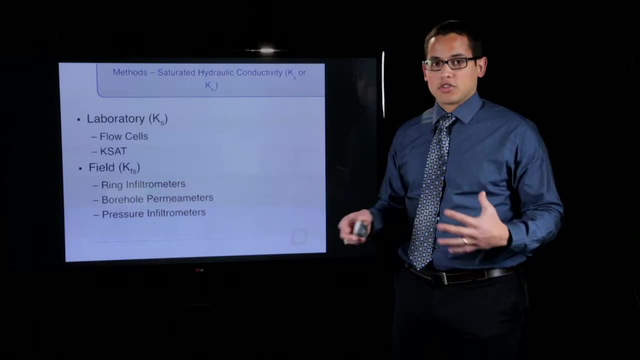 conductivity, we can bring the soil cores to complete saturation, whereas in the field it's fairly difficult to bring the soil to complete saturation. Typically you wind up with entrapped air because we're infiltrating from the top and oftentimes there's not a point. 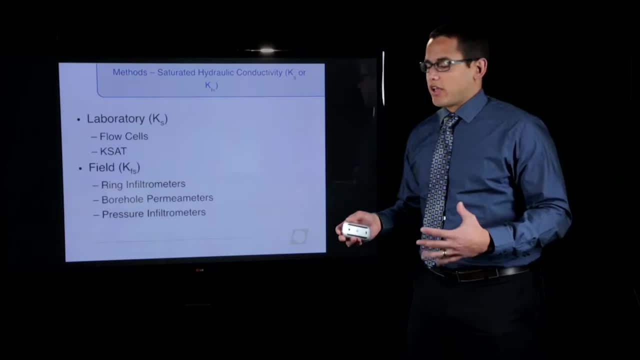 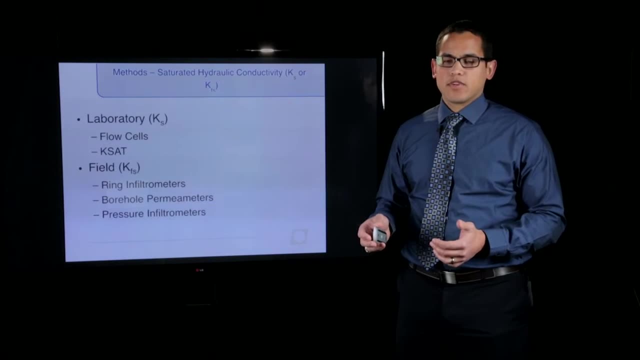 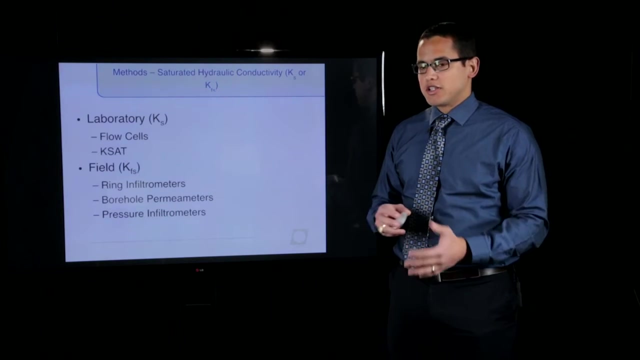 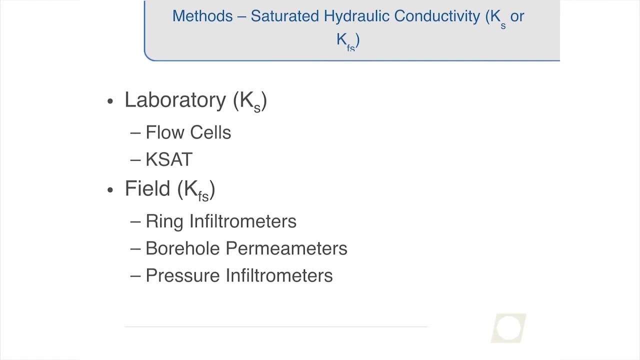 There's not a place for the air to escape, And so that results in not a completely saturated situation, so we call it field saturated hydraulic conductivity, And KFS is typically a little lower than KS just due to the entrapped air actually slowing down water movement. So with laboratory 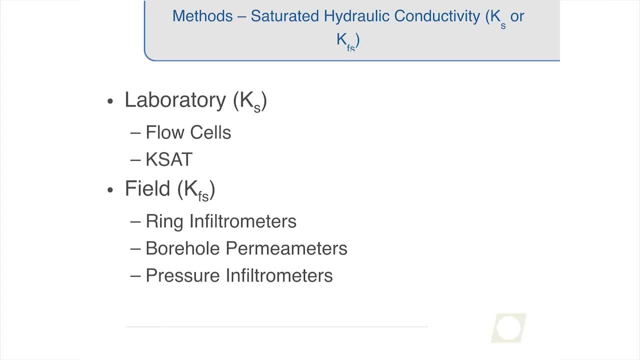 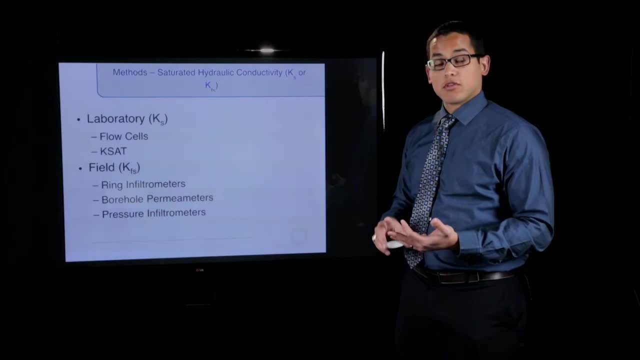 methods for measuring KS. we're going to focus on flow cells and a new instrument called the D-SAT from UMS, and we'll talk about both of those, And then, in the field techniques, we'll focus on ring infiltrometers, borehole permeometers and pressure infiltrometers. 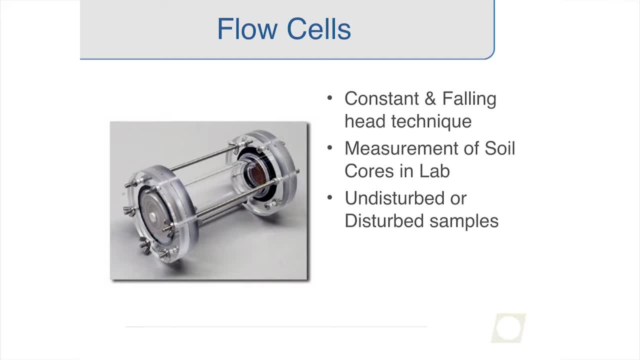 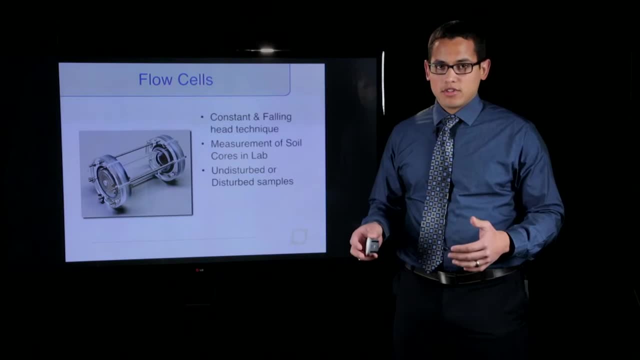 All right, so first let's focus on the flow cells. With a flow cell you can do both the constant and falling head technique. These measurements are typically made on soil cores that are brought back into the lab. You can do undisturbed or disturbed soil samples. 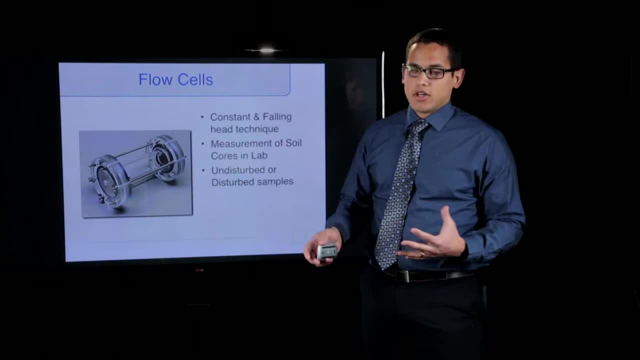 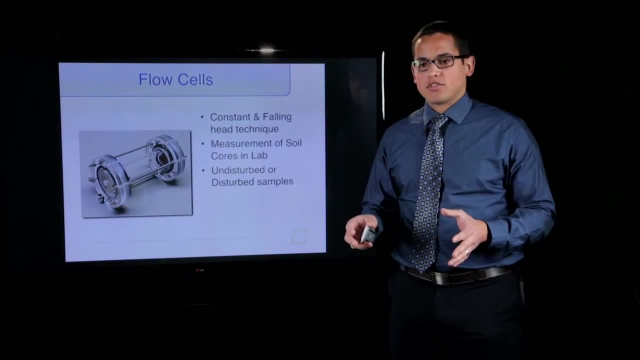 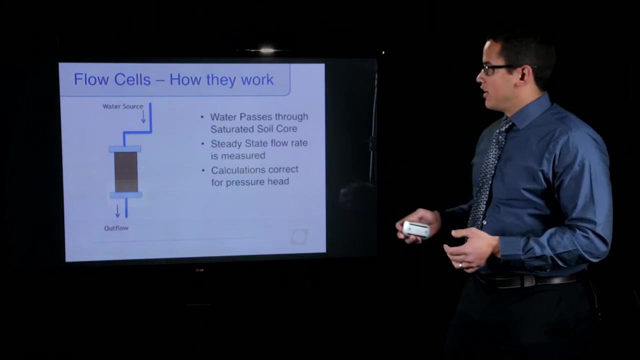 but the size is going to be dependent on the flow cell design, so you are going to be kind of limited to that. So here's kind of an example of how a flow cell works. So you have a soil core that you've brought back to the lab. You can usually typically saturate the soil core before. 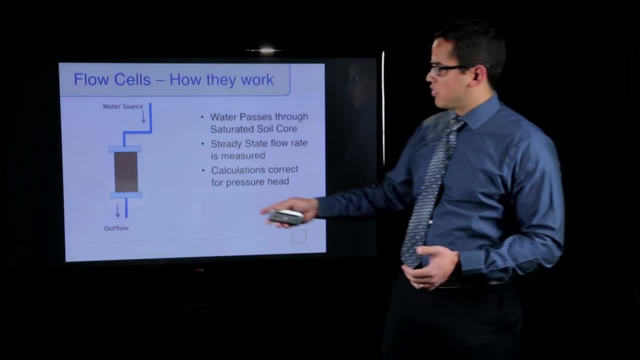 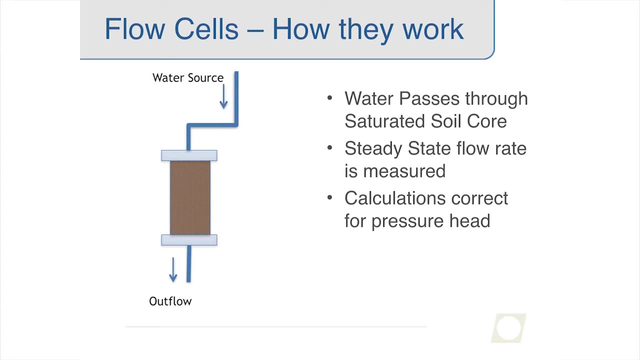 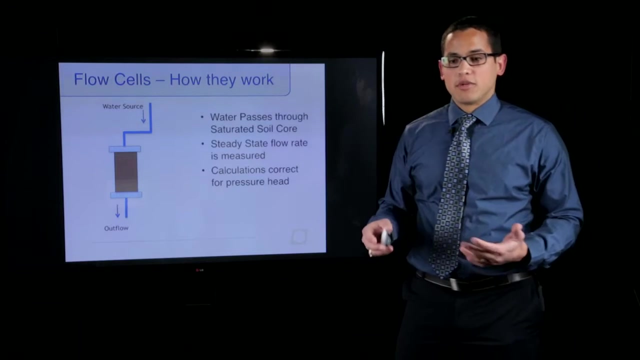 putting it into the flow cell, And what happens is you have this soil core inside of the flow cell. you have a water source that's coming in through the top, or there are other designs, but the water passes through the saturated soil core and the steady state flow rate is then. 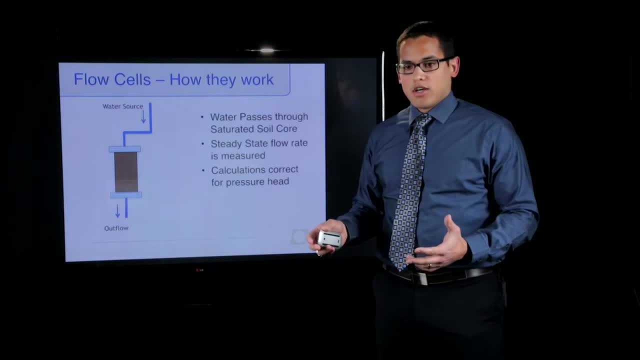 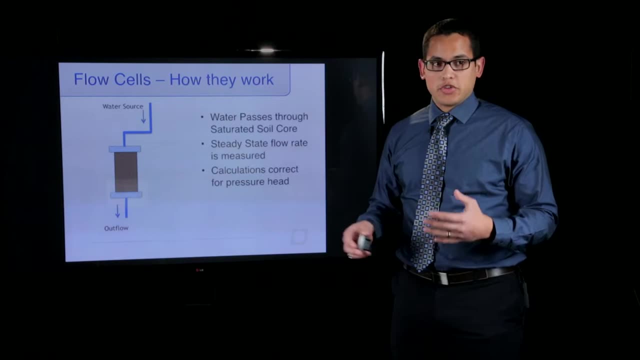 measured And we use that to determine the infiltration rate. and then we make calculations to correct for the pressure head. If we're doing a constant head, then we just correct for that pressure head from the constant head that we designate, whether it be. 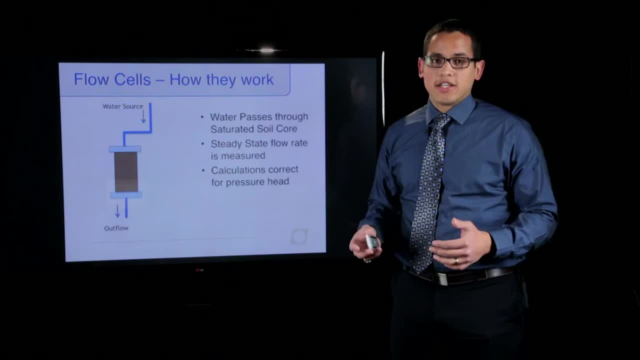 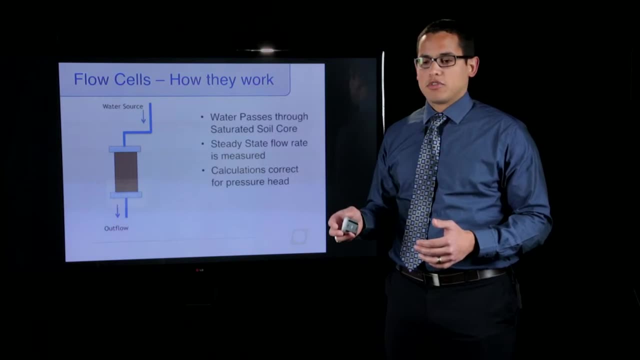 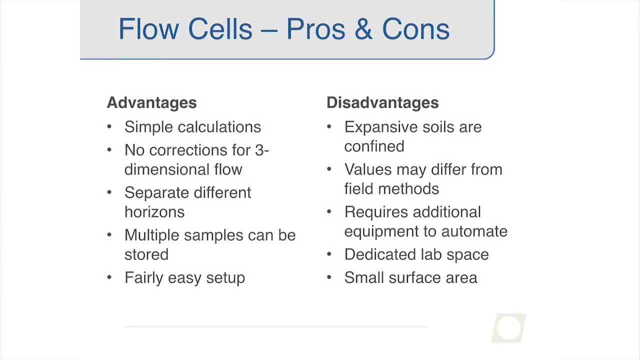 10 centimeters or 10 centimeters, Or if we're doing a falling head technique, then we would have to correct for the pressure head as it changes throughout the times of the measurement. Some of the advantages of the flow cells: the calculations are fairly simple because we're. 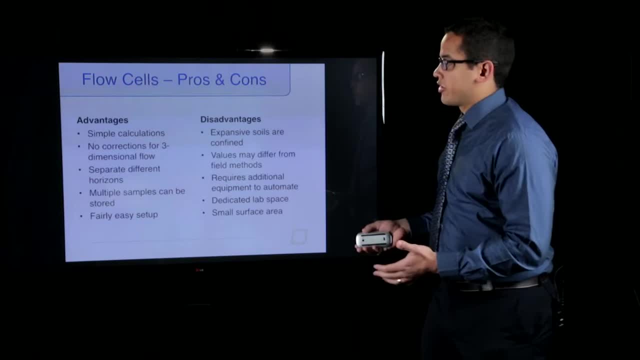 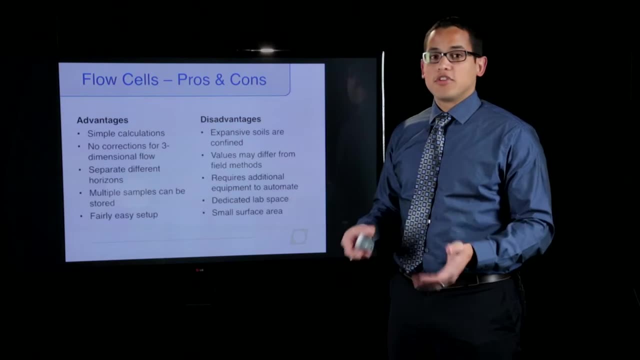 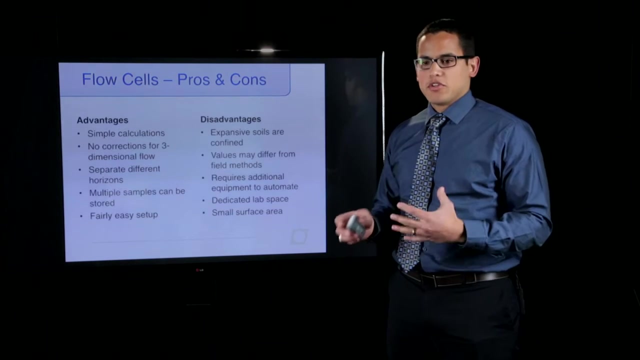 just infiltrating through a known specific area, We don't have to worry about three-dimensional flow because it's a confined soil core, so there's no chance for water escaping, Whereas in the field we have three-dimensional flow that we have to correct for, and we'll talk about that in a little bit. Another kind of cool advantage of 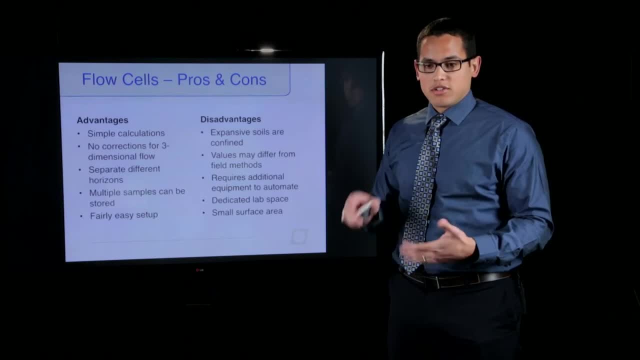 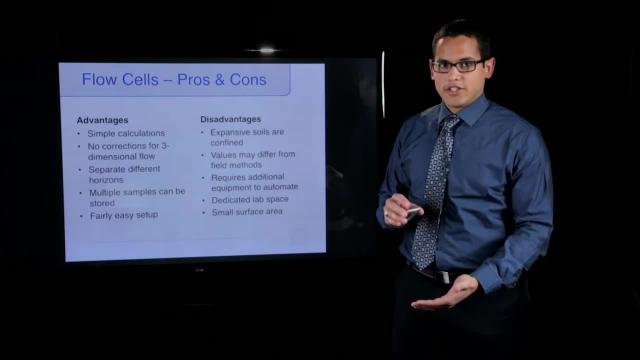 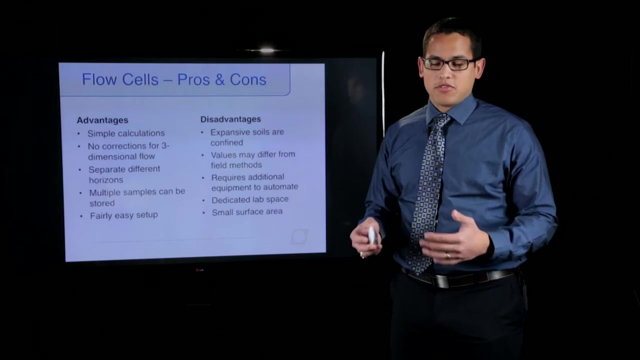 flow cells is we can separate different horizons, So we can take cores from different soil layers and bring them back to the lab and actually measure the hydraulic conductivity of these different layers to understand what maybe is more limiting factor and those types of things. So it's. 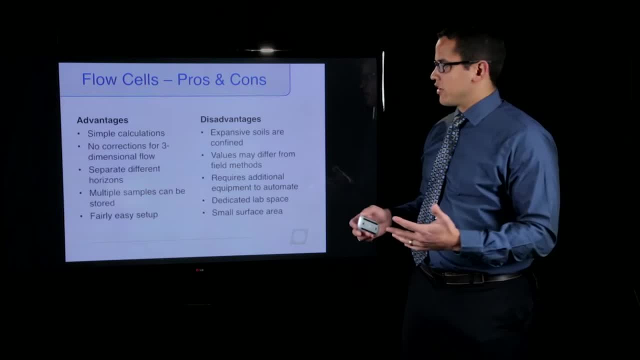 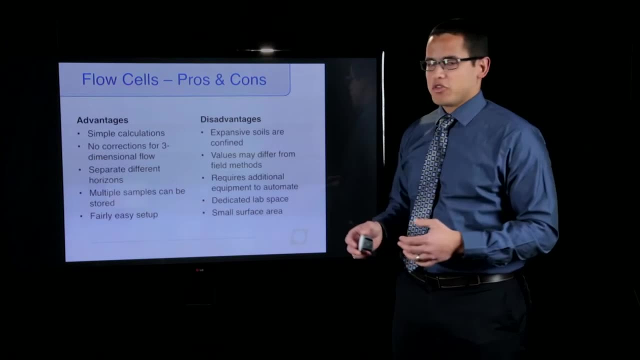 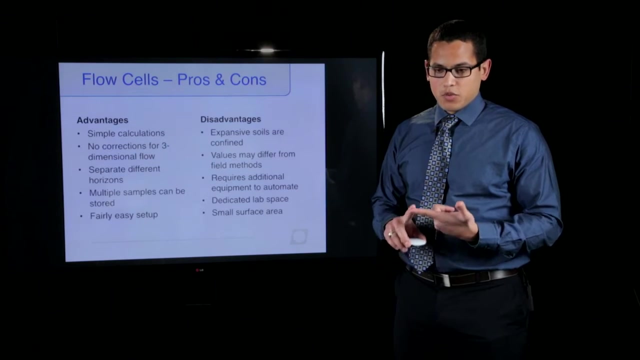 kind of a nice advantage. The other thing is it is a fairly easy setup. There are some complexities to it that mostly is associated with actually getting the system set up and ready. If you want to automate the device, you will need something to control the flow into the cores and something. 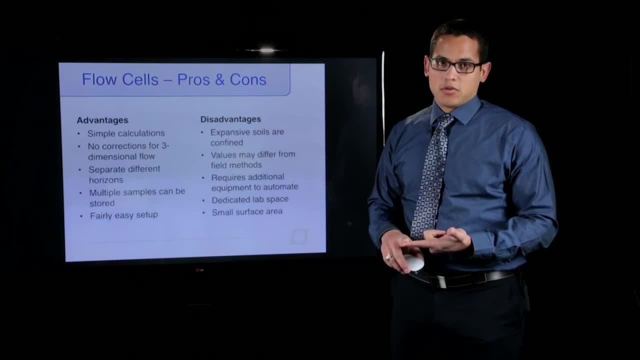 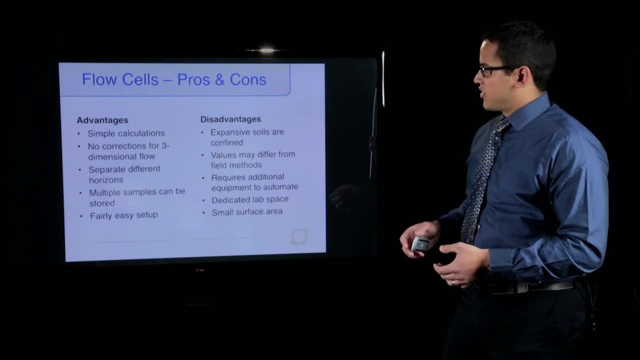 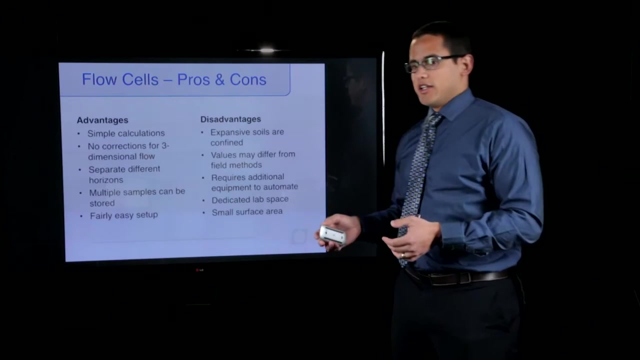 to measure either the flow rate or the outflow rate. So those are some things that you'll have to consider. Some of the disadvantages of flow cells- that's primarily associated with laboratory techniques where you're bringing back soil cores- is expansive soils are confined in. 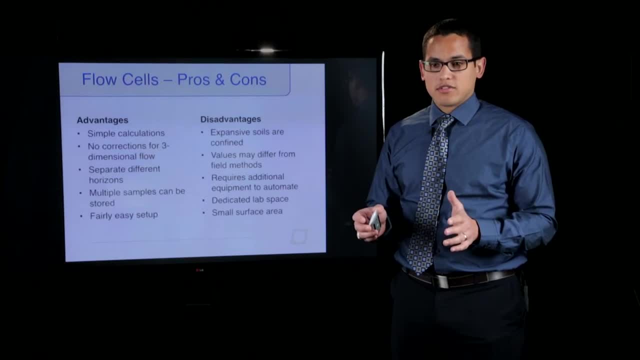 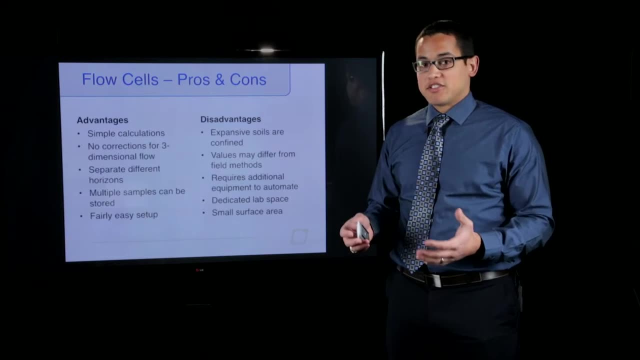 this soil core. So if you start with a soil core that's drier, as it's wetted it begins to expand, and when it expands inside of a core, it actually is confined, and so you can actually start compressing pores and actually change the flow. So that's one of the things that we're going to. 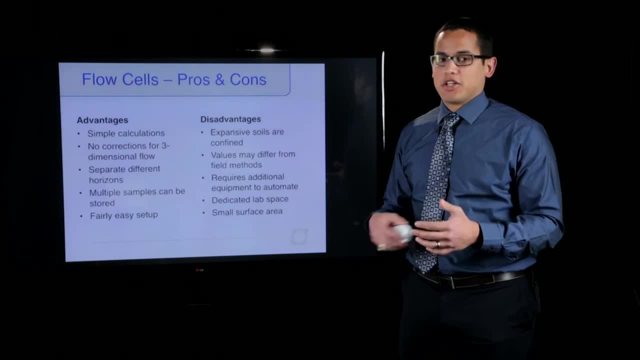 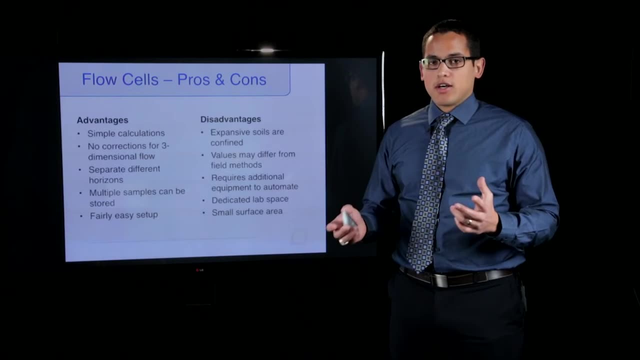 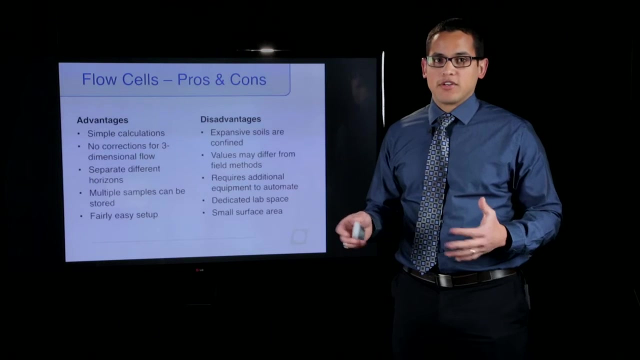 be looking at is changing the properties of that soil, which could actually then cause you to underestimate hydraulic conductivity. One of the ways to overcome that is to sample when the soil is wet or near saturation. That way it's fully expanded and you don't have to worry about it. 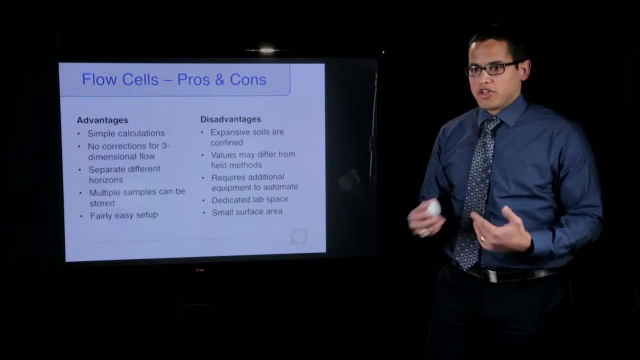 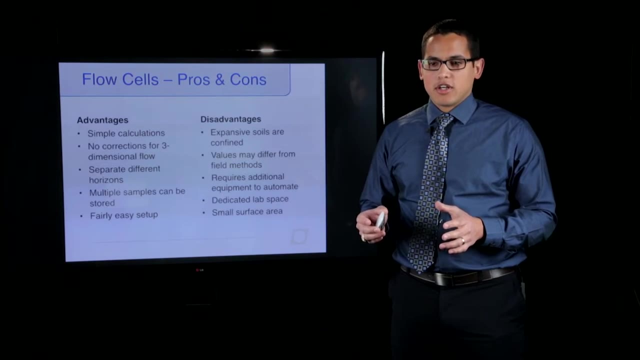 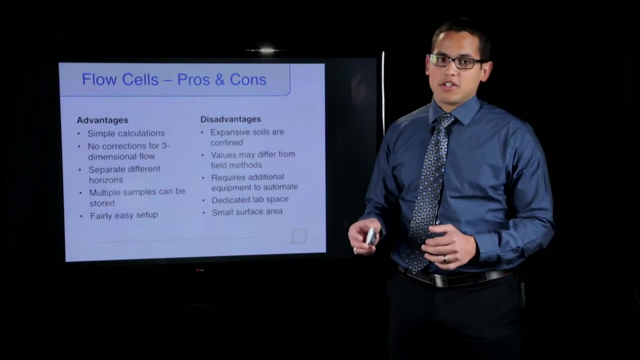 expanding inside of the core. Some of the other disadvantages of the flow cell technique and the laboratory techniques in general is values may differ from field methods and typically you actually tend to overestimate hydraulic conductivity with this technique. One of the reasons for this is you could have 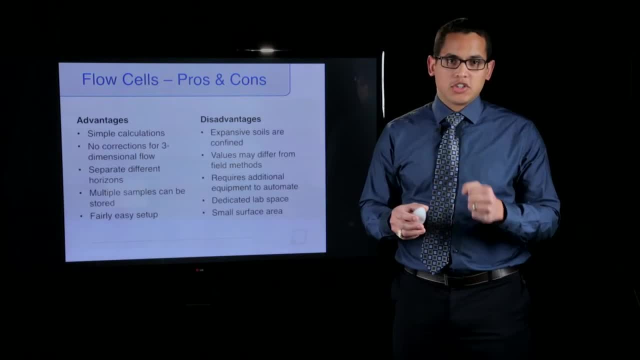 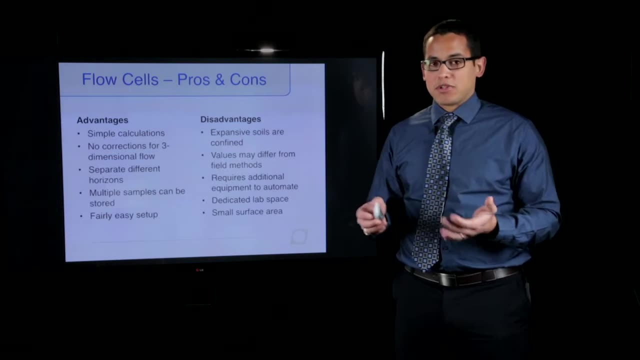 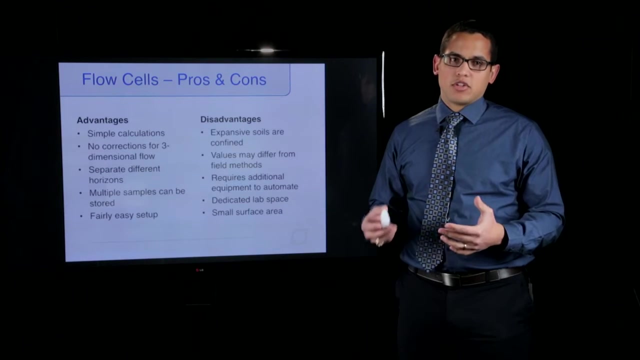 for example, a macro pour that in the field is actually closed off. but if you take a core sample and bring it back into the lab, then you wind up with that macro pour potentially being opened and being an open-ended pour and water can easily flow through that and so you'll get an. 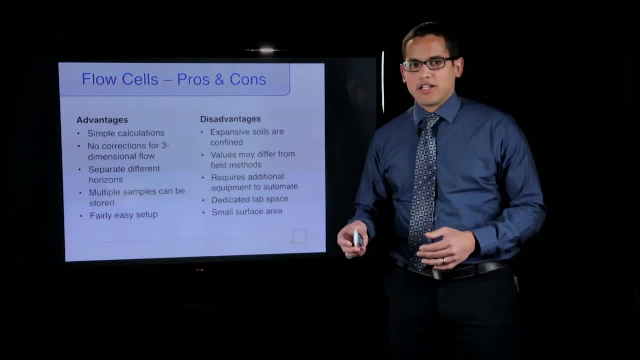 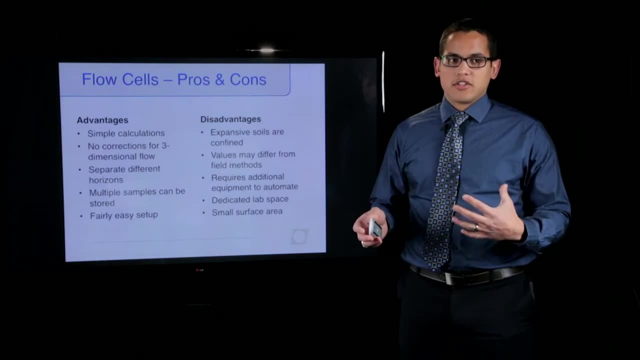 overestimation of how much water is in the field. So that's one of the things that we're going to look at in terms of hydraulic conductivity and that's typical with the laboratory techniques for measuring KSAT With flow cells. there's not really a simple system to set up and put in your 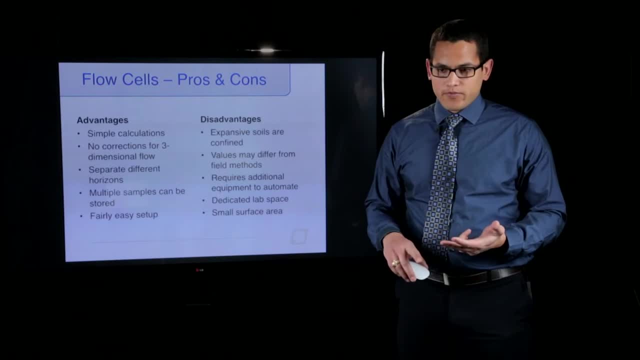 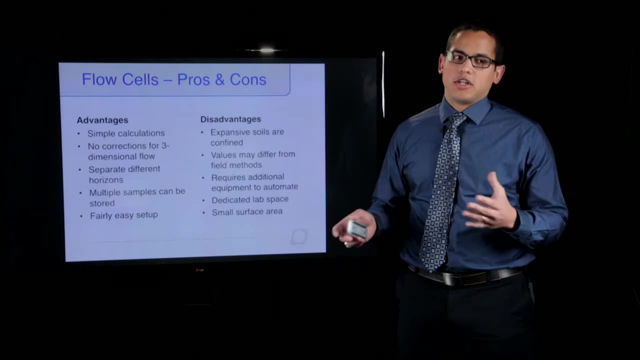 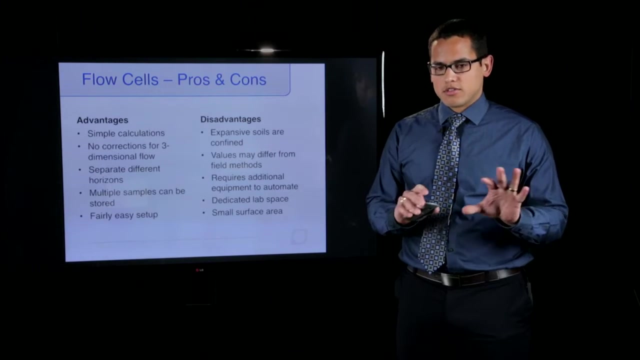 lab. It typically requires additional equipment to automate, and one of the other disadvantages is they typically require dedicated lab space because some of the equipment to automate it and get everything set up can be fairly large and needs to stay set up, just due to the complexity of actually getting these systems put together. 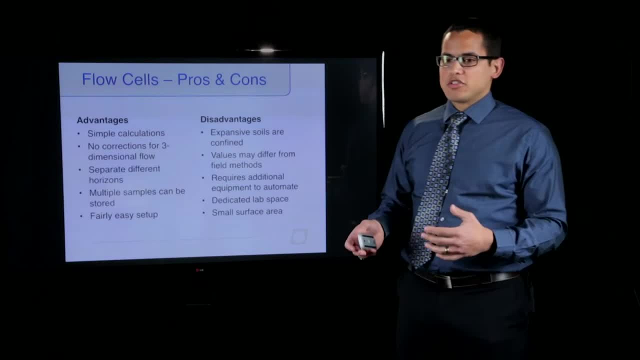 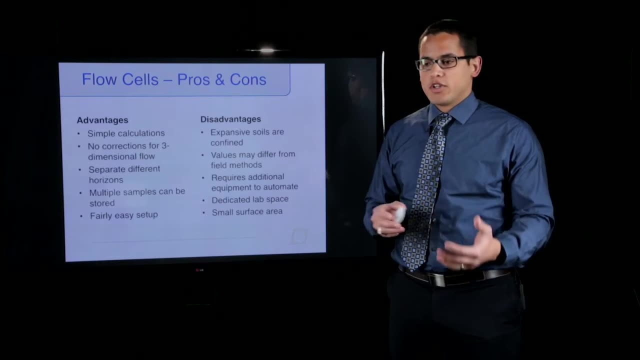 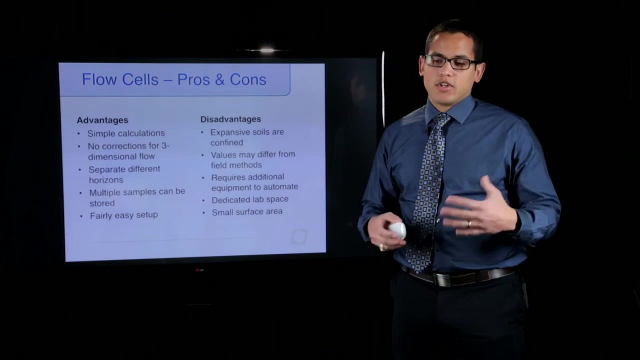 and making sure they work. One of the other disadvantages of flow cells is the small surface area. Due to the fact that you're taking kind of a small core, you don't always get a good estimate of the spatial variability of hydraulic conductivity, and so, to overcome this, 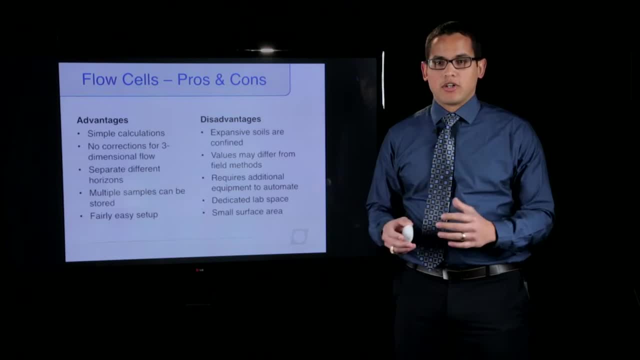 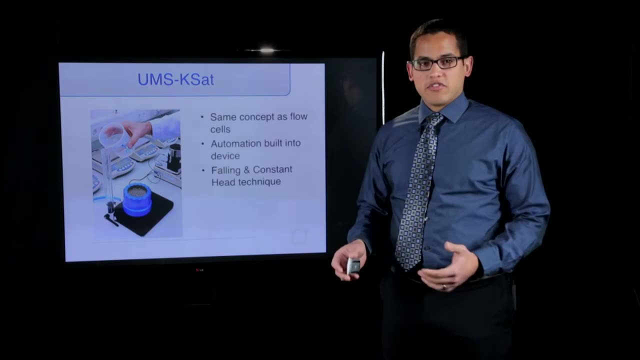 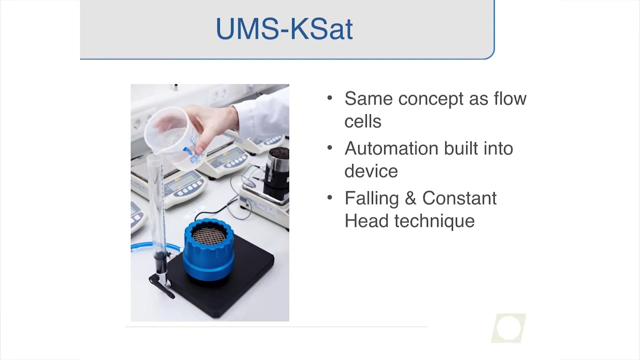 you have to usually take more samples just to get a better representation of the field that you're sampling from. So another tool that's available- it's very similar to the flow cell concept- is the KSAT from UMS, and the way this device kind of simplifies. 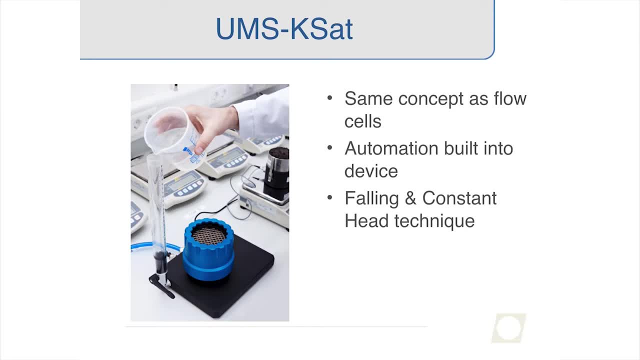 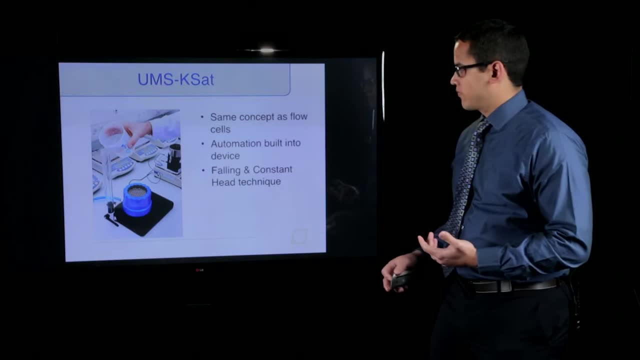 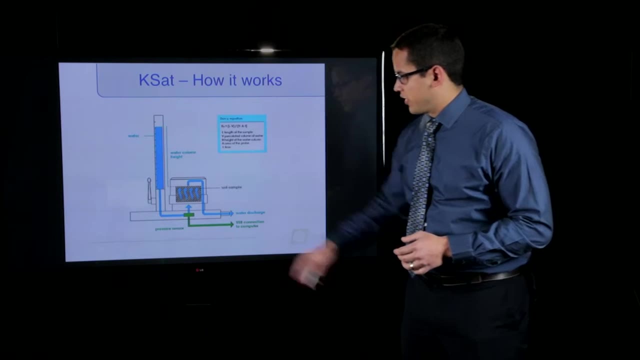 things is. the automation is built into the device. It's also capable of doing the following and constant head technique similar to flow cells. The way the KSAT works is: you'll have a small soil core which you can kind of see right here, and then you have a water column. 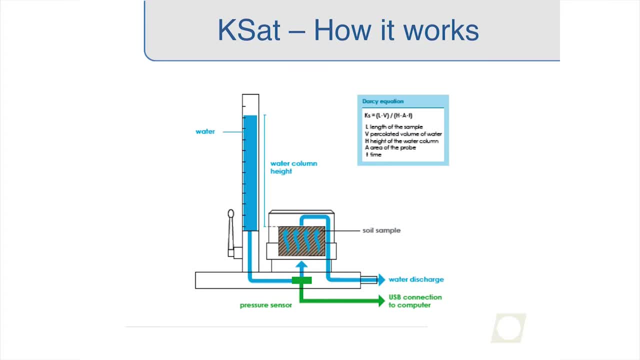 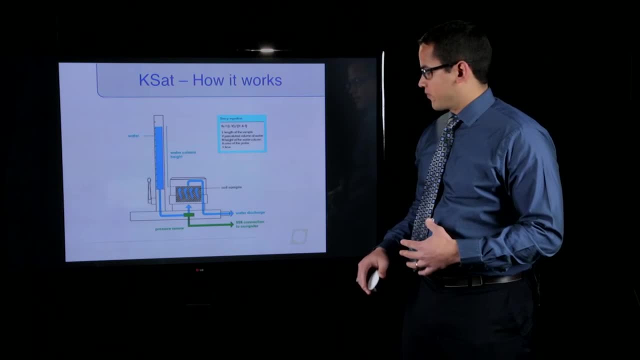 with a burette to control the water flow, and then you have a pressure sensor that's actually measuring the pressure head from the water column. The device is then connected to a computer through a USB connection and that is where all of the automation comes in. The computer measures the 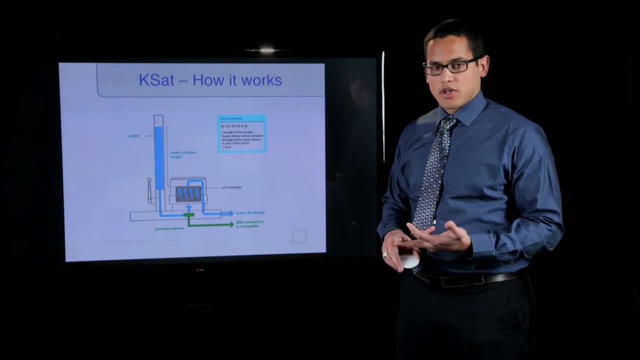 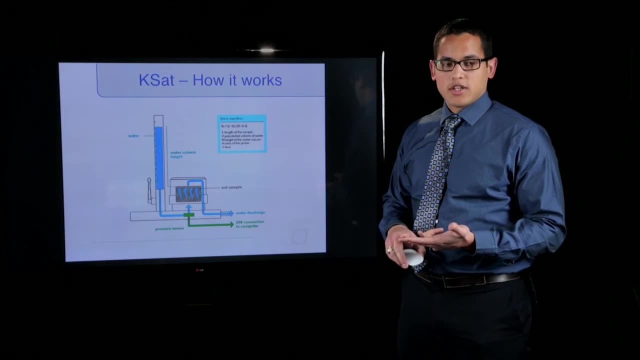 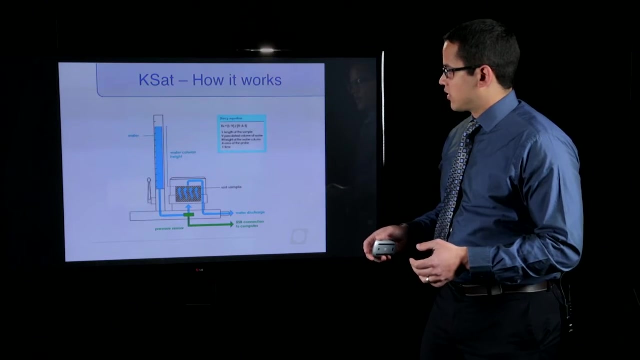 instrument and measures the readings from the pressure transducer. and then there's software which does all of the calculations and also does all the corrections for the viscosity of water changes at different temperatures, and so it's kind of a nice, a nice feature. So the water passes, comes through the burette. 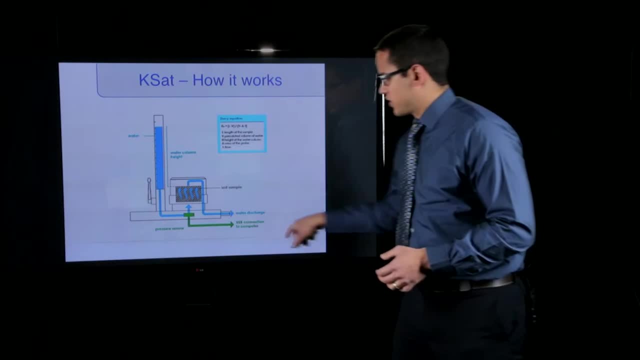 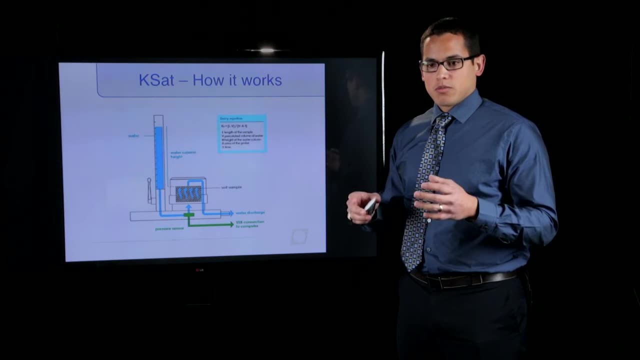 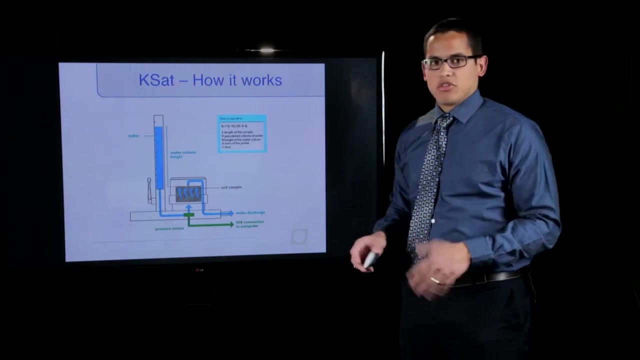 and then through the bottom of the sample and then outflows over the top of the sample And when doing the falling head technique, the pressure transducer measures the change in the water column and then, And through that, we're able to calculate the flow rate and very easily calculate the. 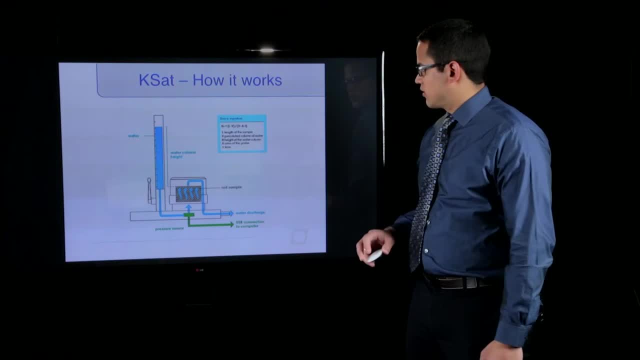 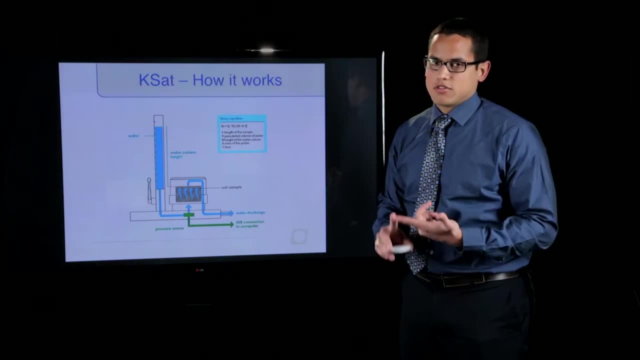 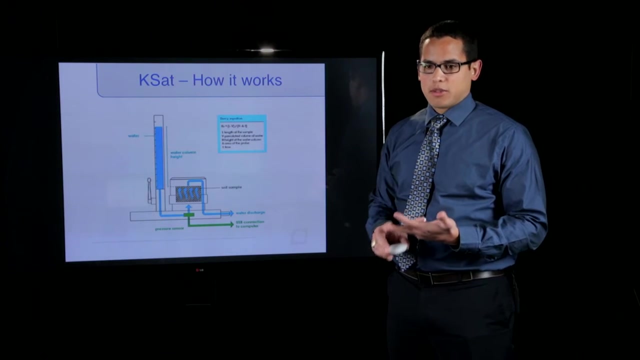 hydraulic conductivity of that sample, Similar to flow cells. the KSAT has some of the same limitations due to such a small surface area and the fact that it's a confined sample, So you'll want to make the same considerations when sampling for this device as well. 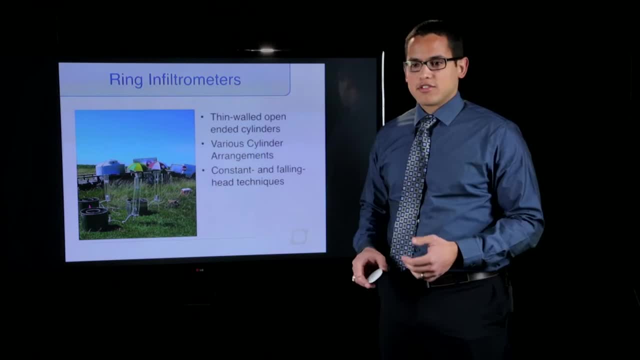 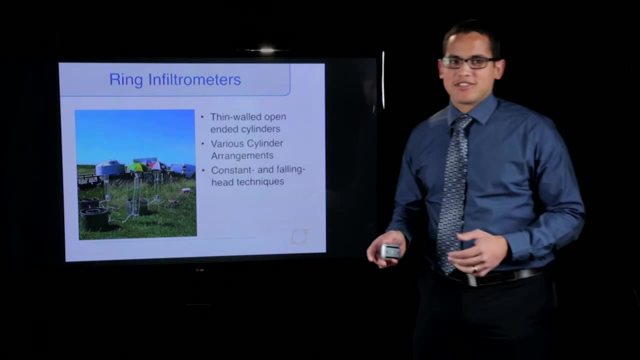 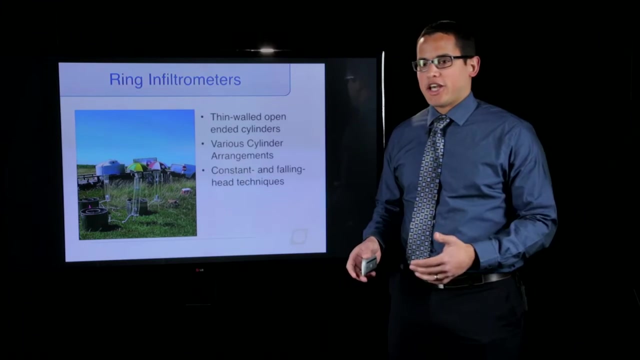 Alright, now let's get into field techniques. These are probably my more favorite techniques One because you actually get to get outside and make measurements And typically what I've found is that some field techniques tend to represent- or better represent- what's actually going to happen in the field. 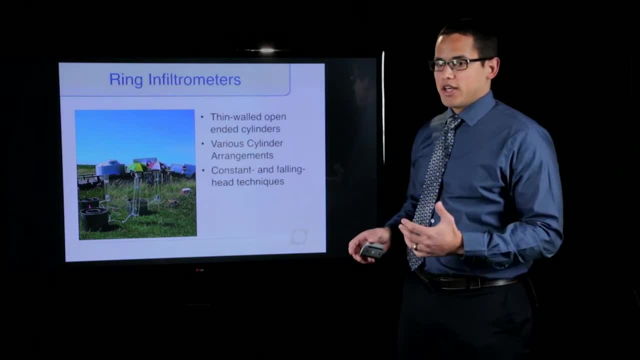 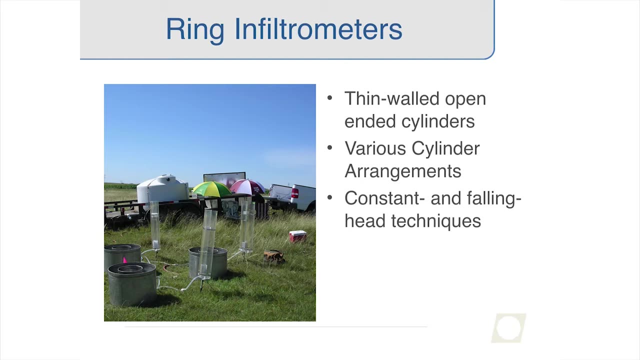 So one of these techniques is ring infiltrometers, And essentially what a ring infiltrometer is is a thin walled, open-ended cylinder that you would insert into the soil So specific depth, typically around five centimeters, And then you'll infiltrate water through these rings, using either the constant or falling. 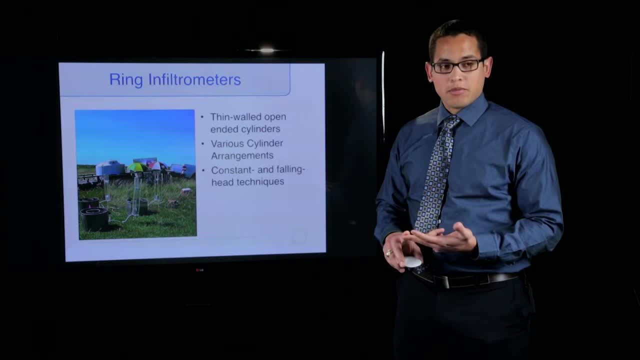 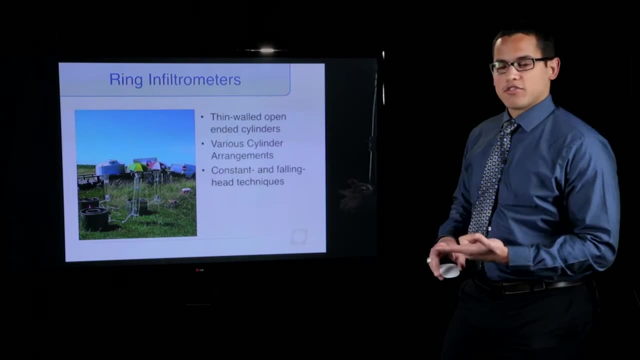 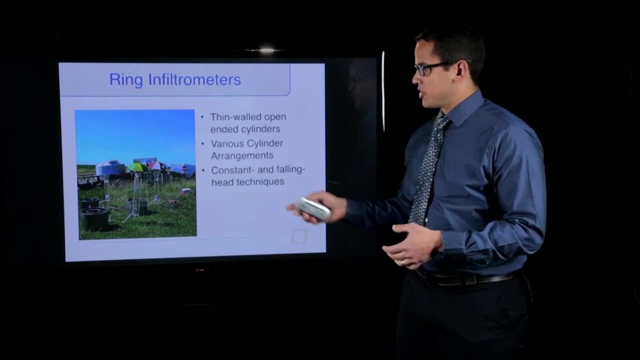 head techniques, And you can do this either manually or you can automate the system to get automated measurements of field saturated hydraulic conductivity. When you are trying to automate this system, the nice thing about it is it does allow you to make multiple measurements at the same time. 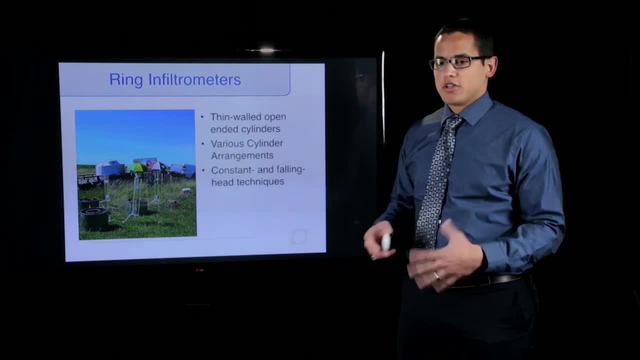 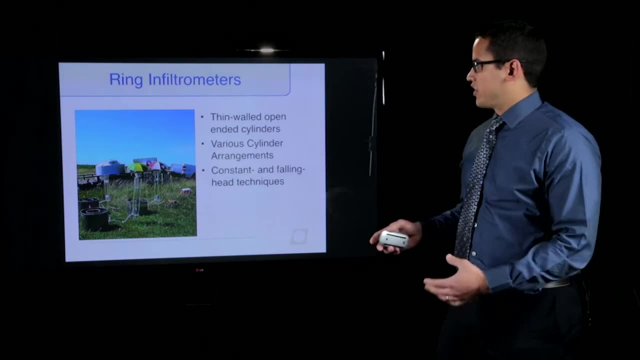 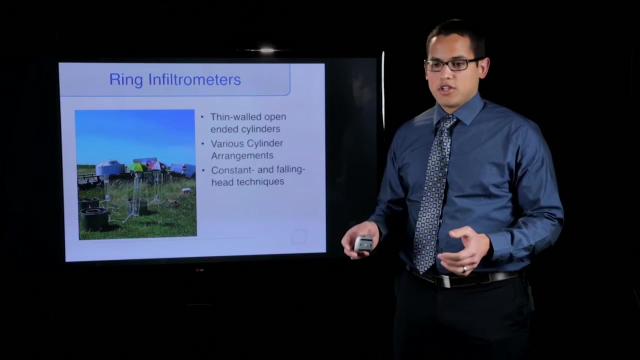 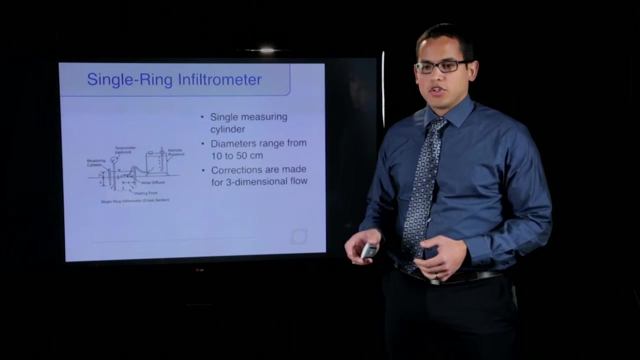 Which is useful when trying to, depending on your research or your research goals. There are various cylinder arrangements. You can have a single ring or double and concentric ring infiltrometers, Which we'll kind of talk about that right now. So with a single ring infiltrometer, you have a single measuring cylinder, which is depicted. 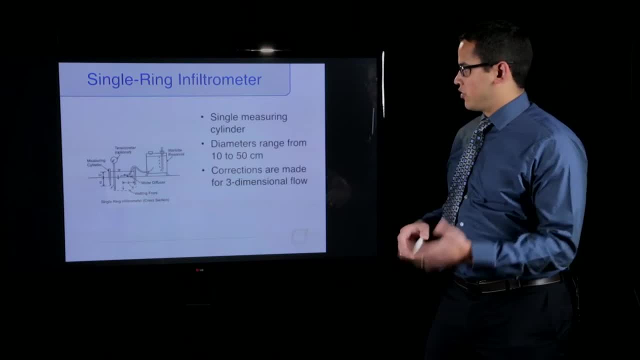 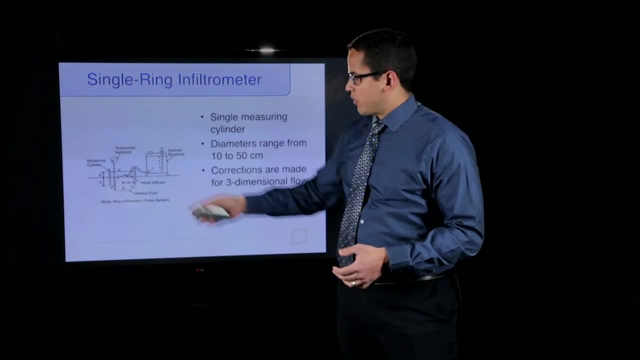 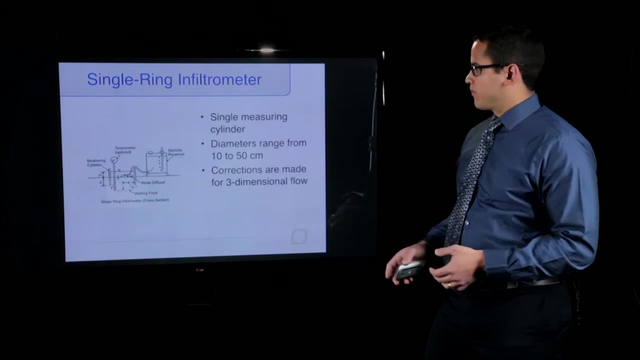 here And the water is infiltrated through the cylinder again using the constant head or falling head technique. When doing the constant head technique, you can usually use a reservoir with a Marriott bubbler to control the flow and control the water level inside of the ring. 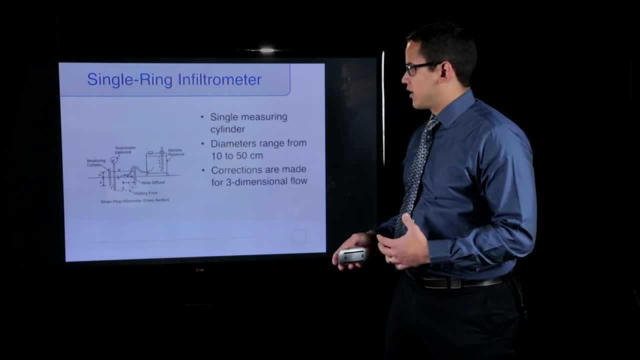 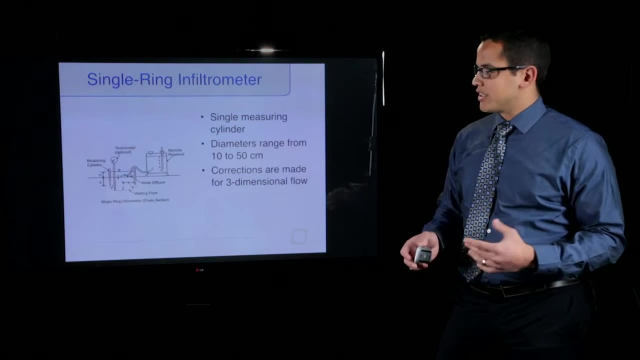 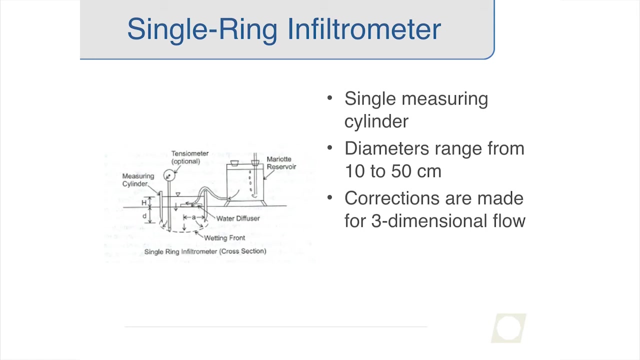 There are other ways to automate this as well that tend to work well, So it just kind of depends on what you would like to do there. Okay, So diameters for single ring infiltrometers range typically from 10 to 50 centimeters. 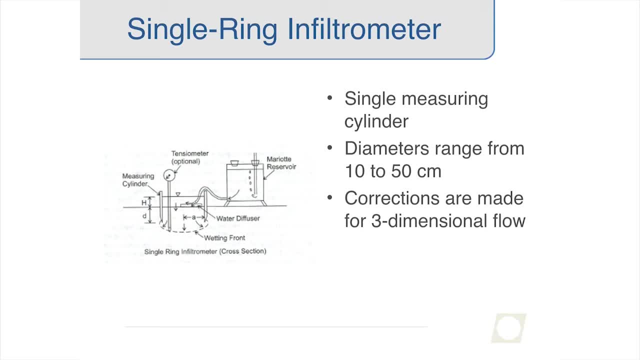 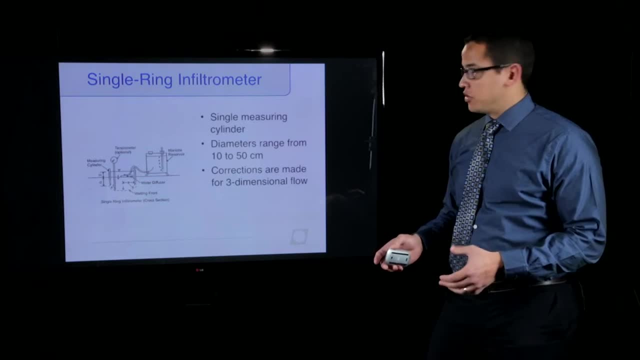 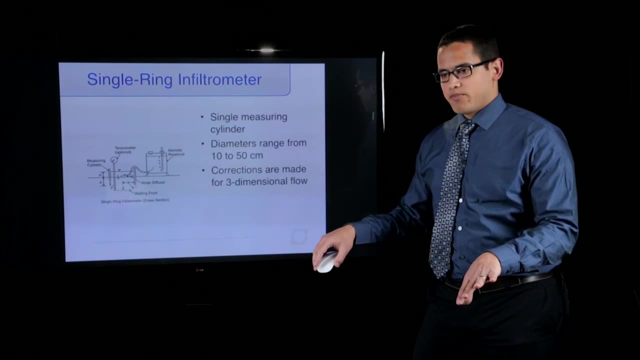 The bigger the diameter you can get, the more area you'll cover, which gives you a better representation of the spatial variability. With single ring infiltrometers you do get three-dimensional flow. As the water infiltrates from the ring, it does begin to go out horizontally as well. 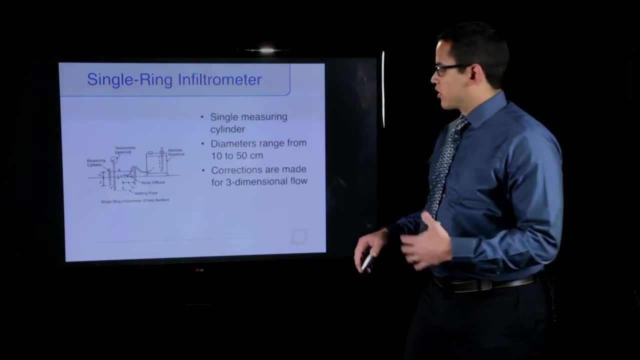 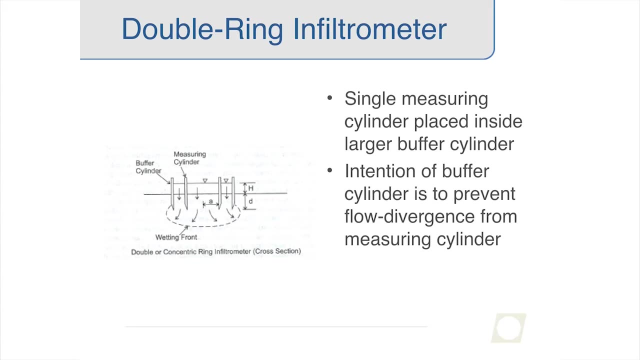 as down vertically into the soil. Okay, Okay, Okay, Okay, Okay, Okay, Okay. So corrections have to be made for three-dimensional flow. The next one is the double ring infiltrometer or concentric ring. With a double ring infiltrometer you have a single measuring cylinder. that is then placed. 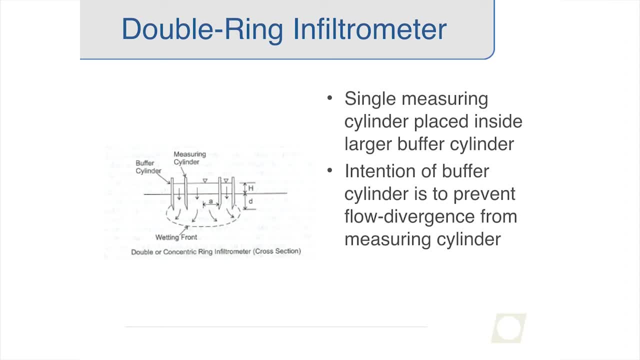 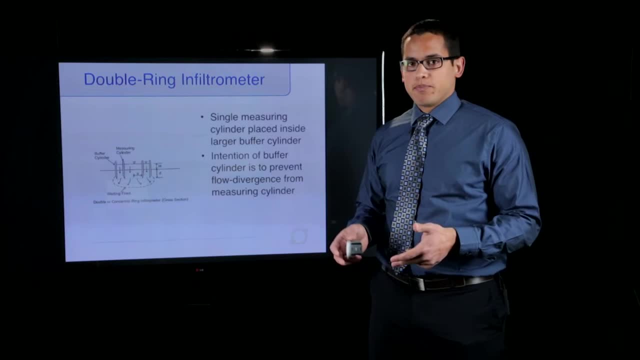 inside of a larger buffer cylinder And the intention of the buffer cylinder is to prevent flow divergence from the measuring cylinder. So in theory, in the measuring cylinder you're only measuring the volume, You're only measuring the vertical flow of water and there should be no lateral flow. 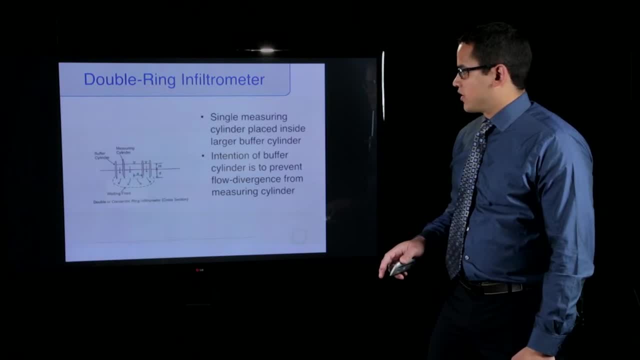 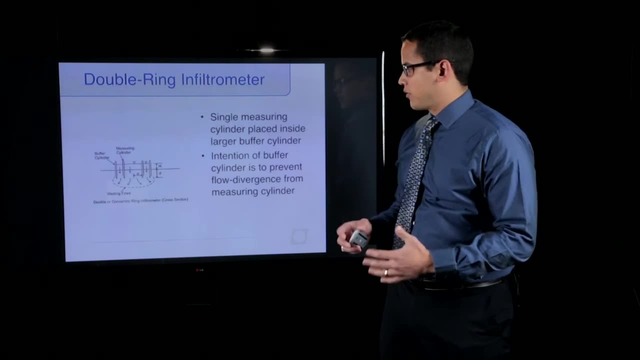 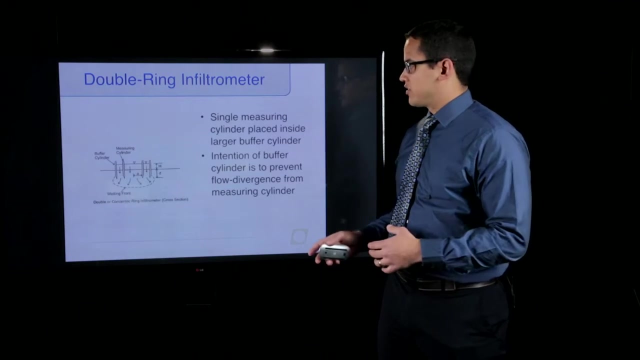 or horizontal flow. The goal of this is to help simplify the analysis, but we'll talk about some of the issues there. With this technique, again, you can do either the falling or constant head techniques. Typically, you'll want to maintain the same level in the buffer cylinder. 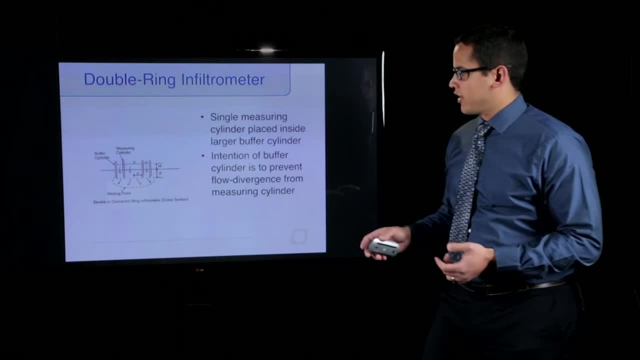 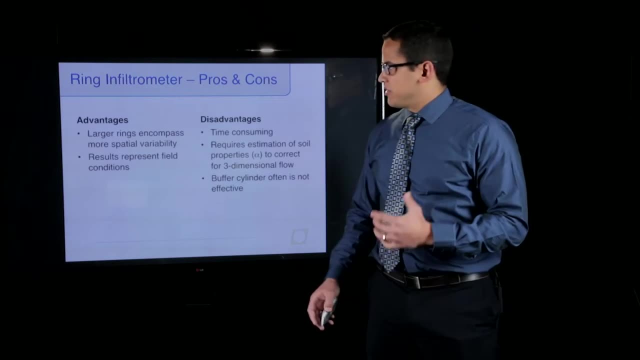 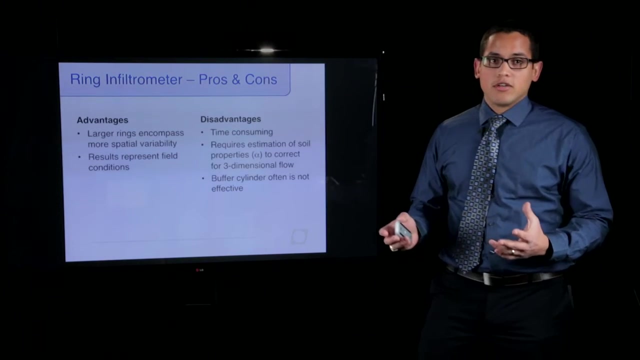 The buffer cylinder as what you have in the measuring cylinder just to get the same pressure gradients. So some of the advantages of ring infiltrometers is with larger rings you can encompass more spatial variability, which helps you better understand what type of hydraulic conductivities. 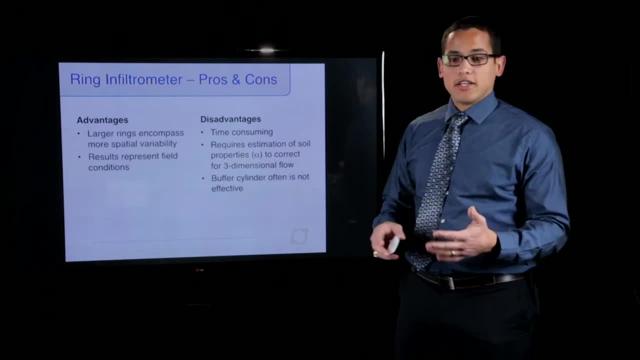 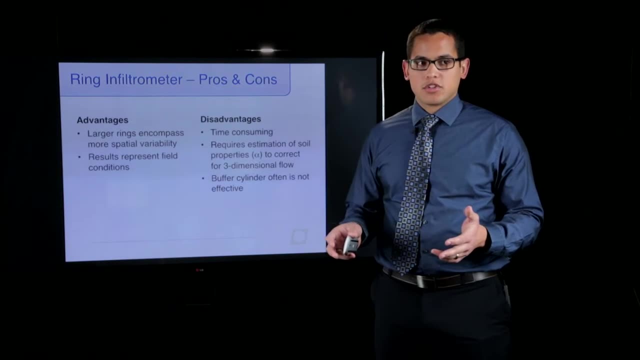 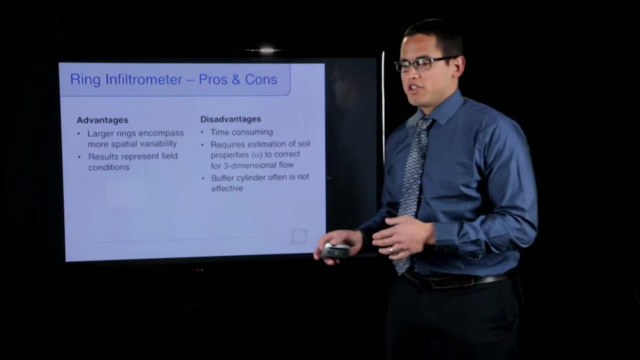 you would see in a field And again, like I said earlier, the results, I believe typically tend to represent field conditions better, which is more suited from a modeling perspective when you're trying to actually understand what's going to happen in a field. 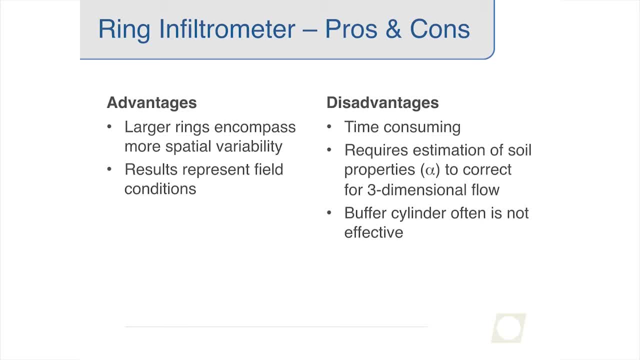 Some of the disadvantages of ring infiltrometers is the measurement is very time consuming. It can take upwards of two to three hours depending on the ring size. The smaller the ring, the less time it takes to reach steady state again. you want to go larger, typically to get more spatial variability, so you're. 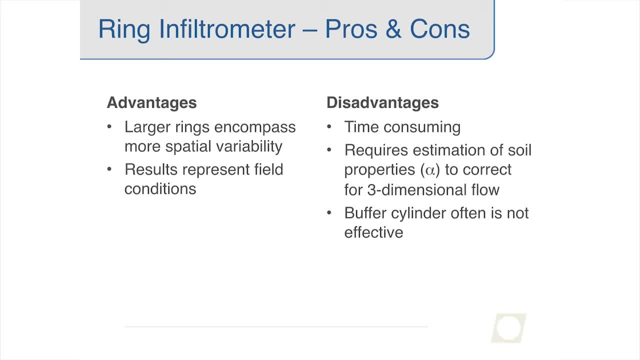 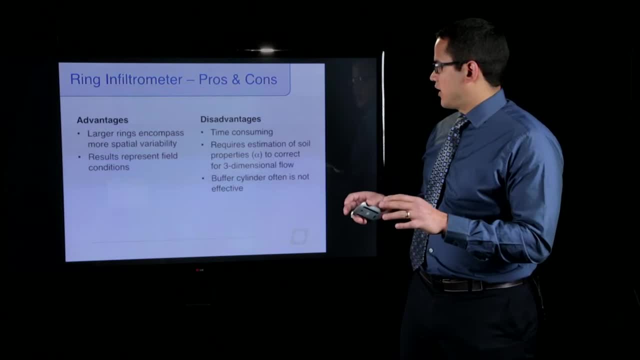 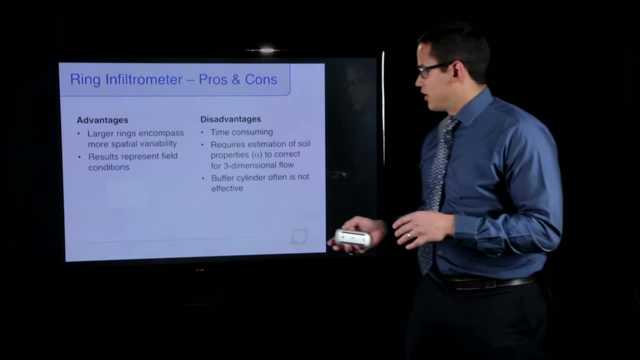 going to run into more time to actually make the measurement and to reach steady state. Another disadvantage is, with this technique, you have to estimate the soil properties, and one of those properties is the soil macroscopic capillary length factor, which is referred to as alpha. in order to correct 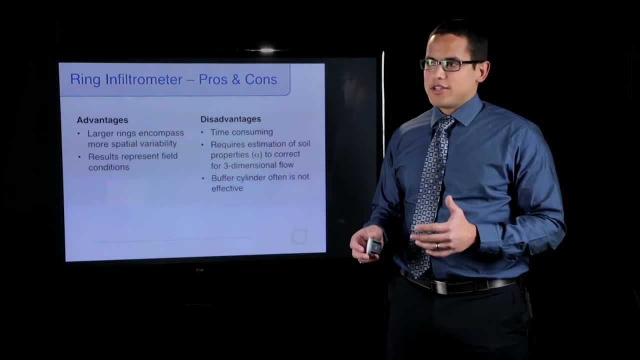 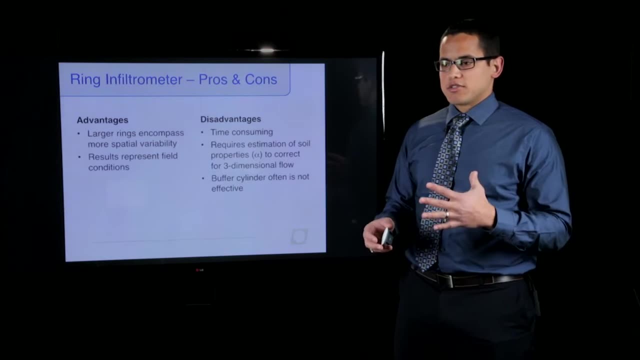 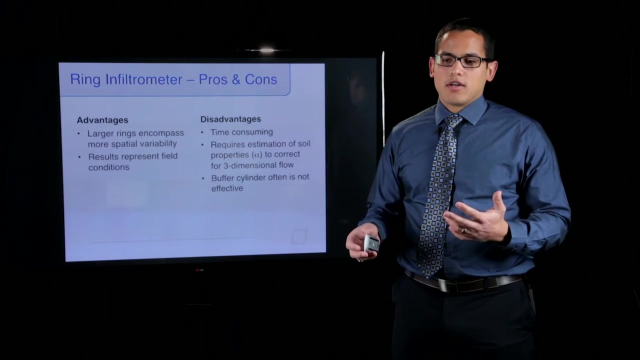 for three-dimensional flow, and so there are tables available to estimate this alpha parameter, but it is an estimation and if you're wrong it can affect your hydraulic conductivity values, which can result in inaccuracies in your estimates of hydraulic conductivity. And then one of the other. 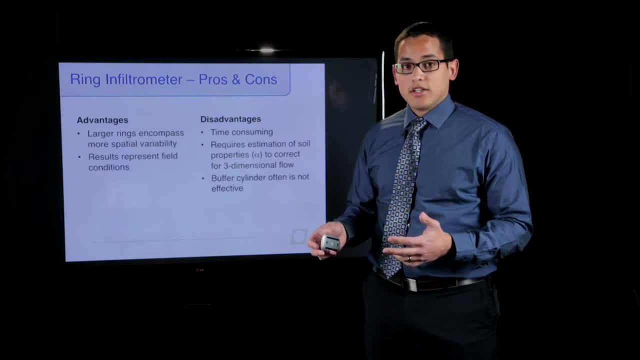 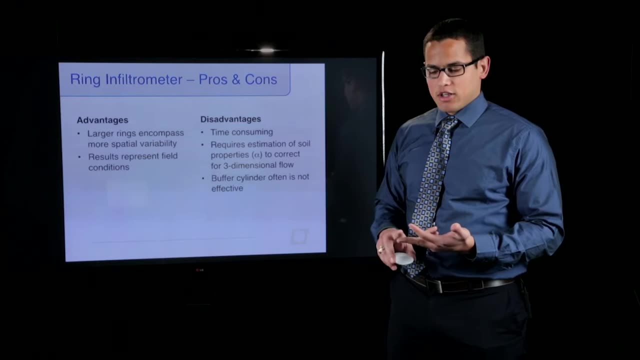 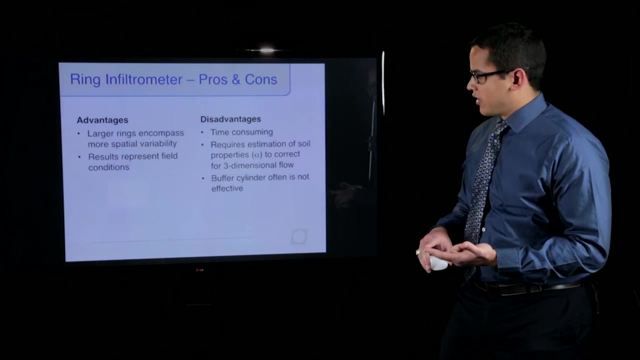 issues with ring infiltrometers is the buffer cylinder often is a little bit of a problem. It's a little bit of a problem because it's not effective and this has been shown through lab and and modeling analysis of this double ring infiltrometer technique. What they found is that you're still 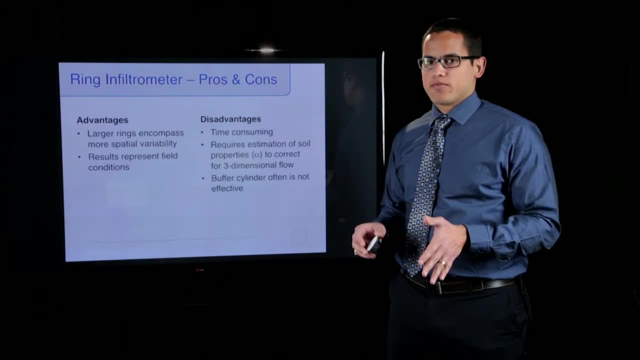 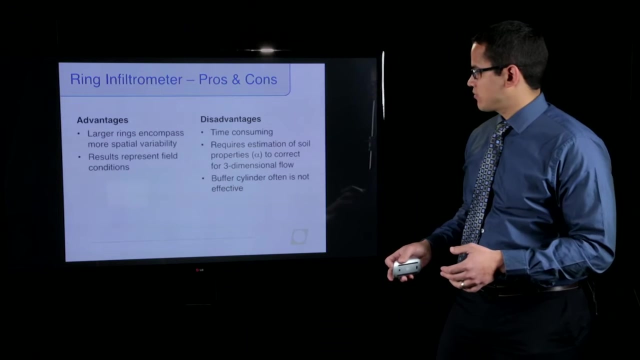 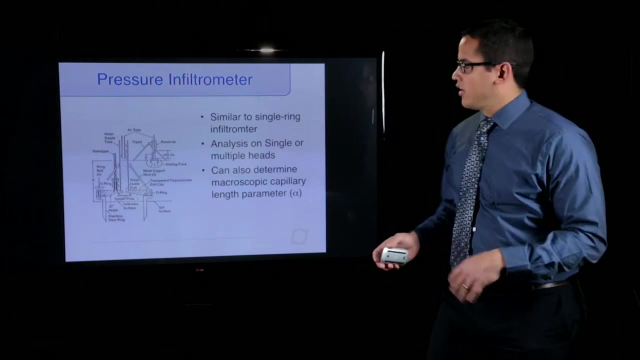 getting lateral flow in the measurement cylinder which, if you go based on the analysis that you're only getting vertical flow, you actually wind up overestimating hydraulic conductivity, which can be an issue. So one of the other techniques is the pressure infiltrometer and the pressure. 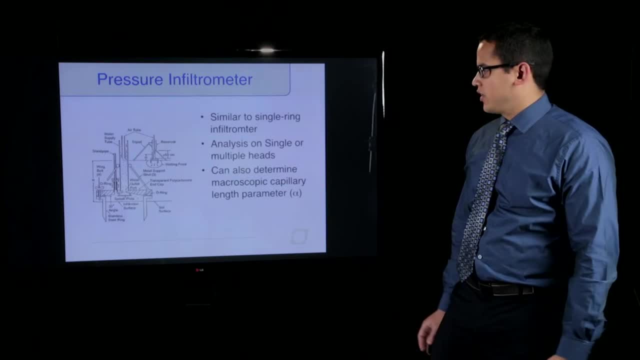 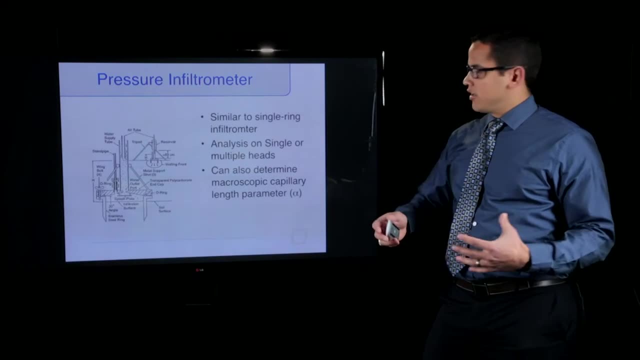 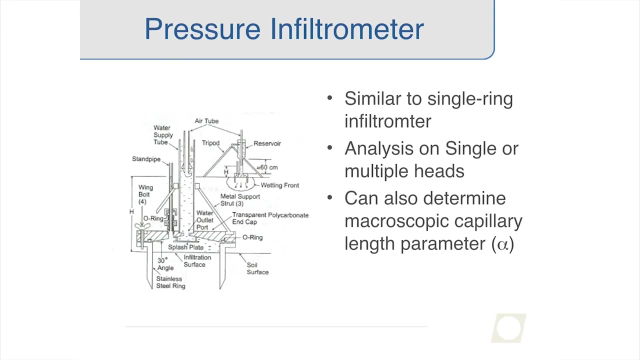 infiltrometer is actually fairly similar to a single ring infiltrometer. You have essentially a single ring inserted into the soil and and then, and then. one of the main differences is you then have an attachment that goes on top of that ring. that allows you to. 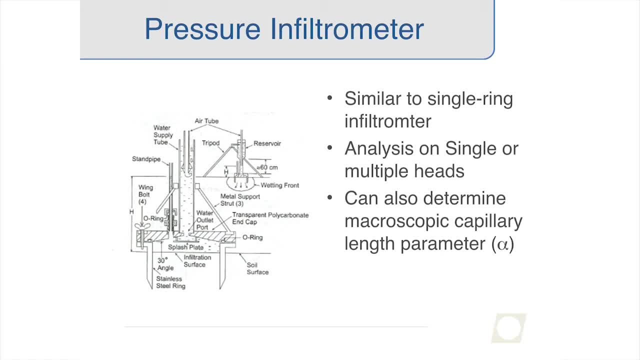 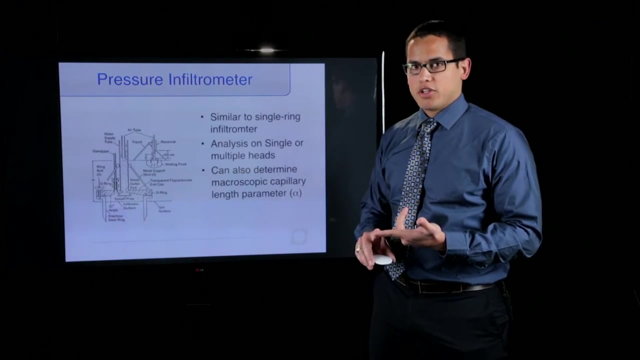 to actually control the pressure head of the pressure head that's being applied over the ring, which can be advantageous because if you can do, then do a multiple head analysis, so changing the pressure heads. this actually allows you to do other measurements, such as sorptivity, and you can also determine the 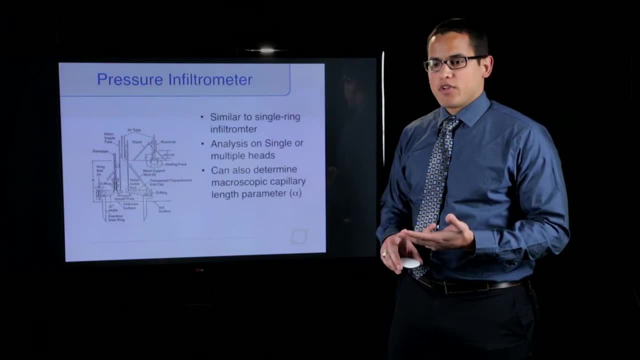 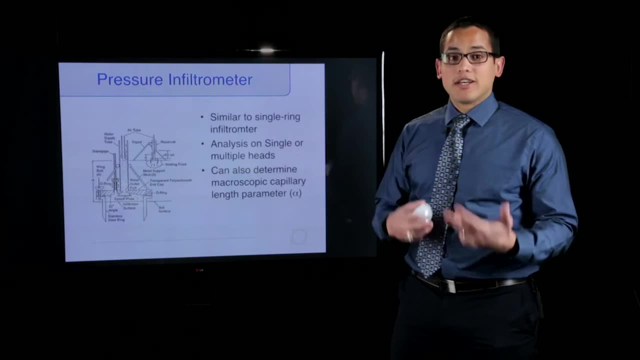 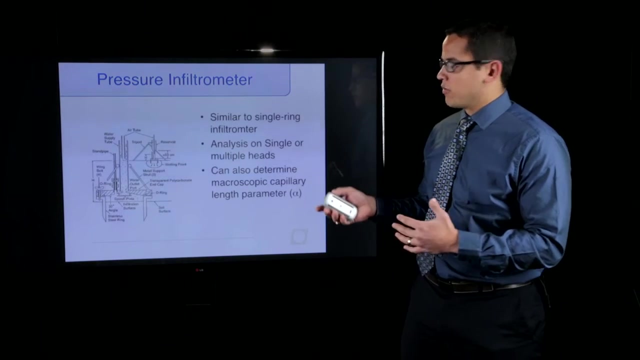 macroscopic capillary length factor that we just talked about earlier, The alpha value, by doing this multiple head analysis which then removes the need to estimate it and again removing another source of error, and and so, with this technique, typically the way it works if you, especially if you're doing, 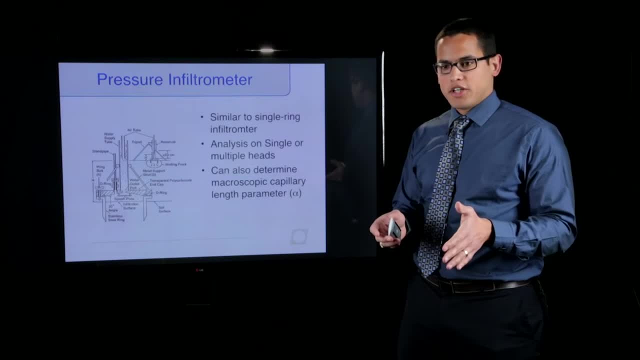 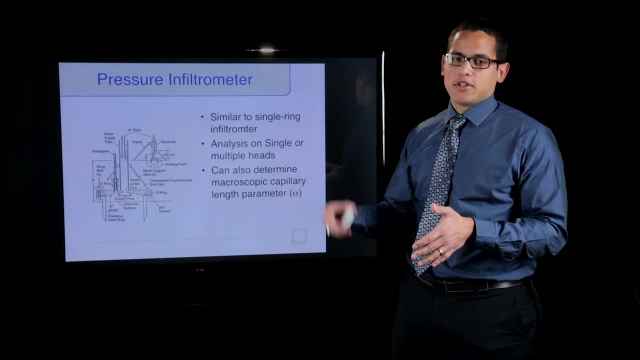 the multiple head analysis. you would start with a single head and apply that constant single head for a certain amount of time, then switch to maybe a higher pressure head and apply that first set interval and then switch back down to the lower pressure head for a set interval and switch back up and the goal is to eventually we reach the quasi. 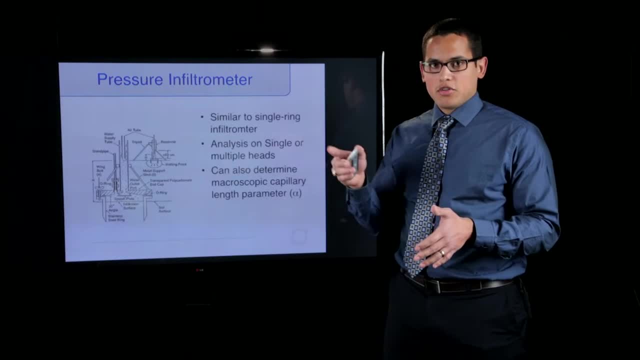 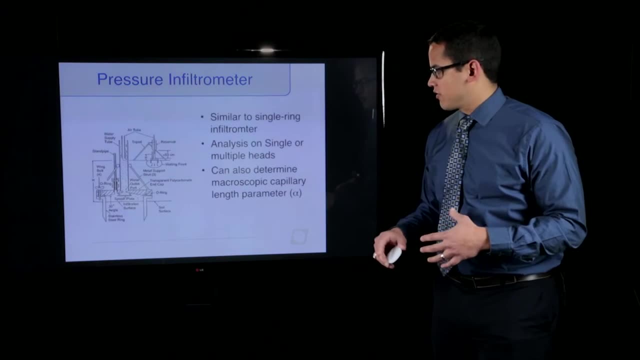 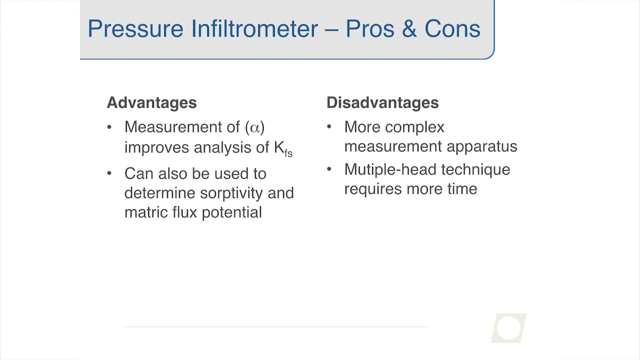 steady state for all, for both pressure heads, and then you can use the, the infiltration rates at the two different pressure heads, to to estimate these values, that such as the, the alpha value, or sorptivity. So with the pressure infiltrometer there are pros and cons, just like with any of the other. 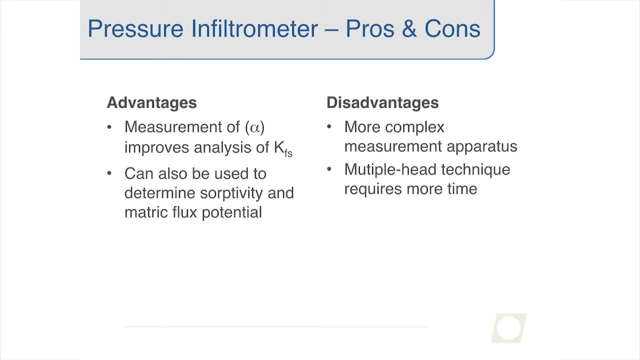 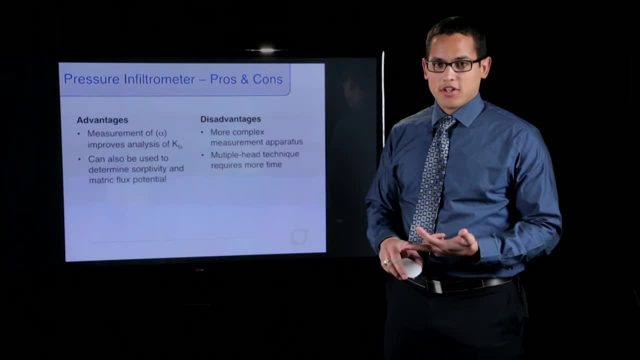 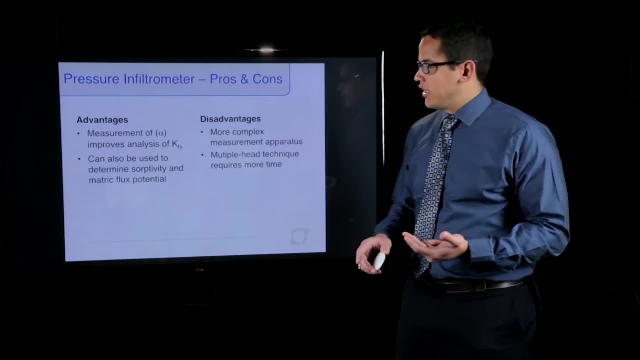 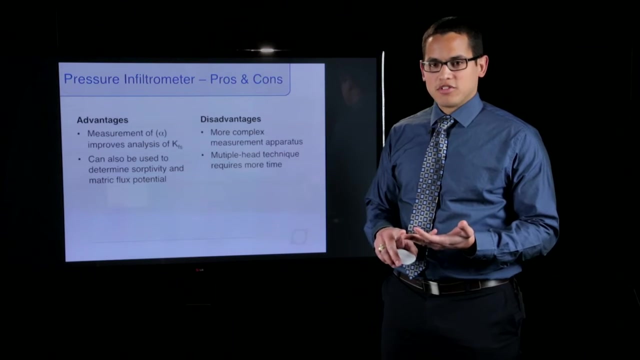 techniques. One of the advantages with this technique- technique again- is the fact that you can measure the alpha parameter, which then improves your analysis for of the field titrated hydraulic conductivity when you're going in correcting for the three-dimensional flow, and you can also determine sorptivity and matrix flux potential, which is it, you know. it's always nice to. 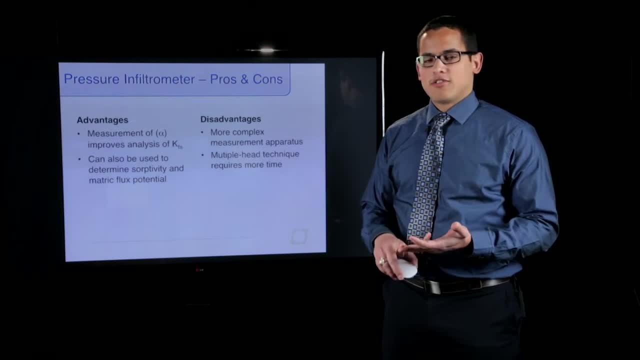 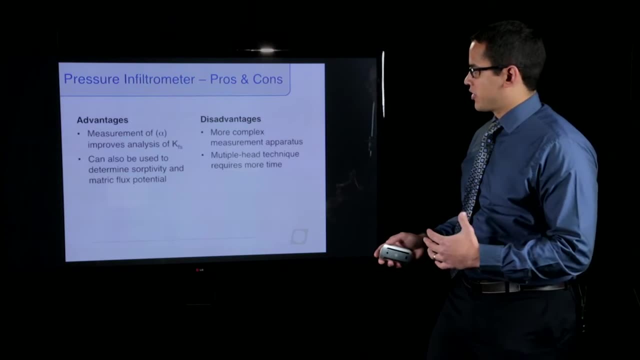 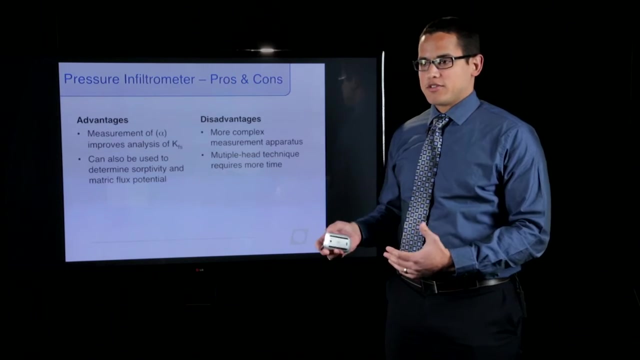 be able to get more hydraulic properties and parameters for your soil in one measurement. One of the disadvantages currently with the pressure infiltrometer is it is a more complex measurement apparatus. If you're trying to automate this, it it. it takes more automation, especially if you're trying to jump to the different. 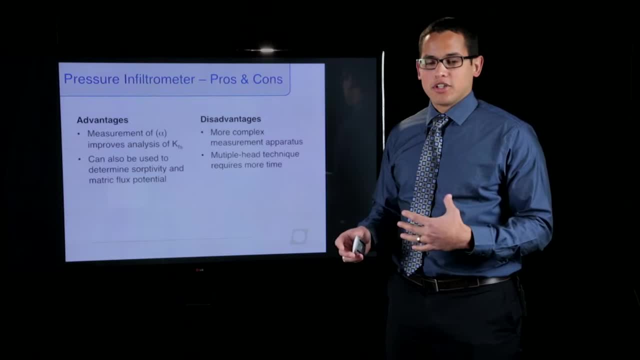 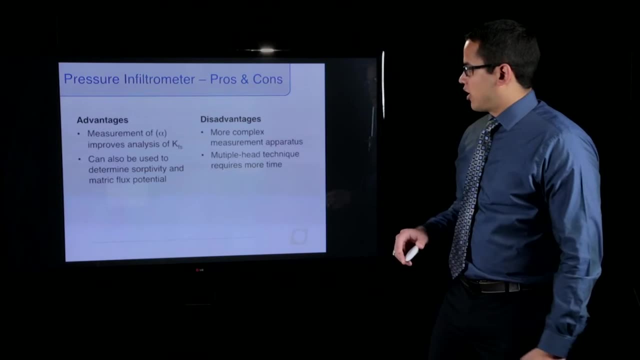 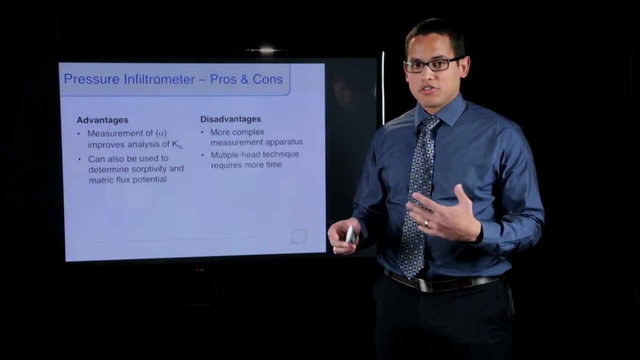 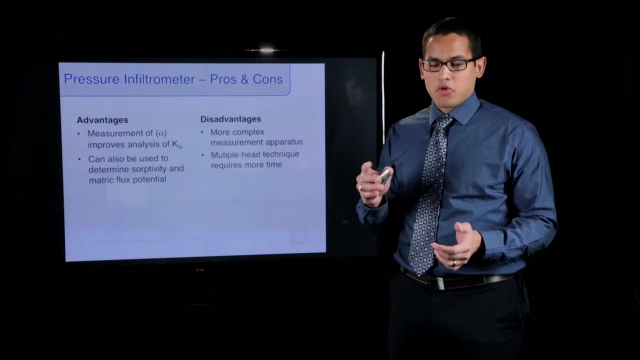 pressure heads There are. there's some work being done to improve this technique and make a simpler automation device simpler automated device When you're doing the multiple head technique or the multiple head analysis. this requires more time and one of the reasons for that is one you have to reach steady state at both pressure. 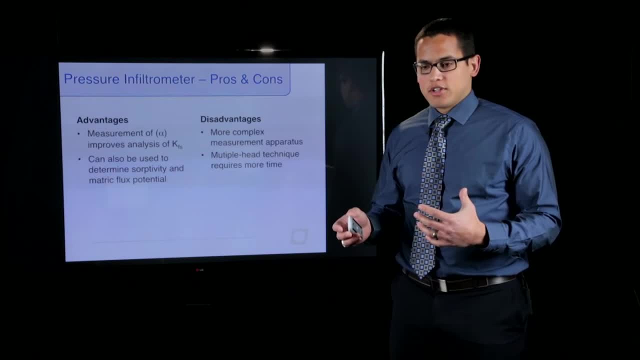 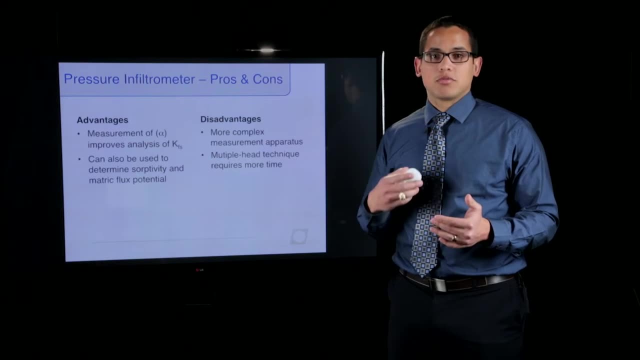 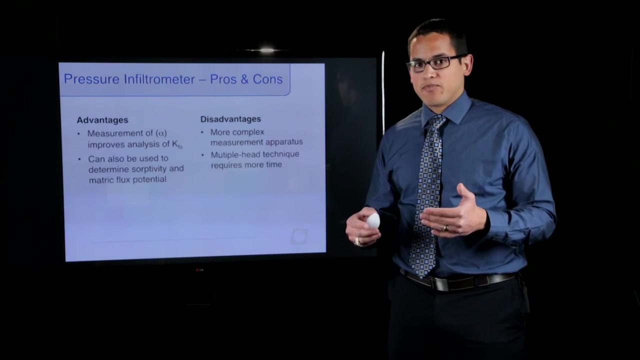 heads. and the other issue is if you're switching from a high pressure head to a low pressure head, and especially if you're doing this with water, then you actually have to wait for the water to go down to the lower pressure head, and if it's a really low conductivity soil, 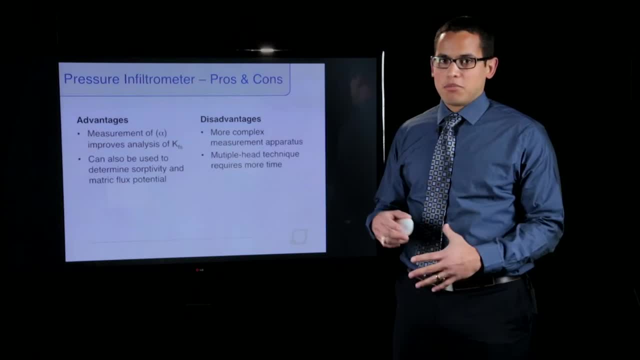 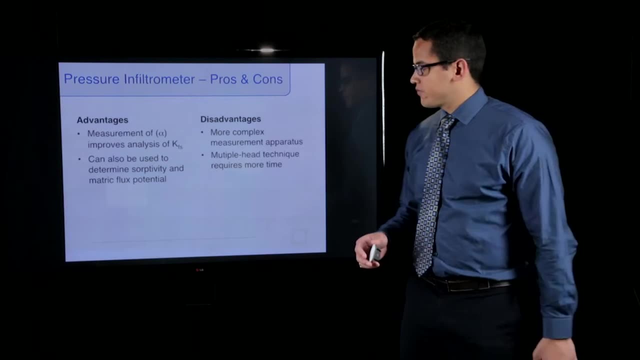 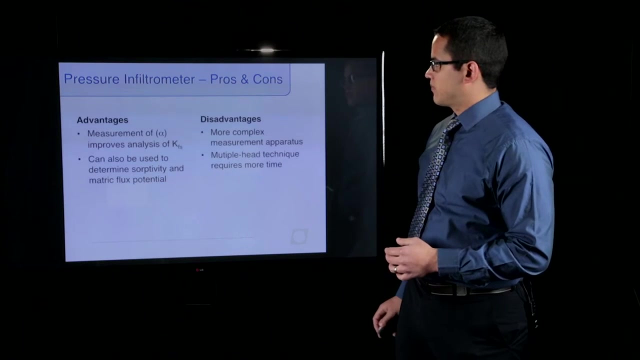 then that could take some time. So this can be a more time-consuming method, depending on how the automation is done and how the pressure heads are are created, but it does have some significant advantages over some of the other ring infiltrometer techniques. The next technique we're going to talk about: 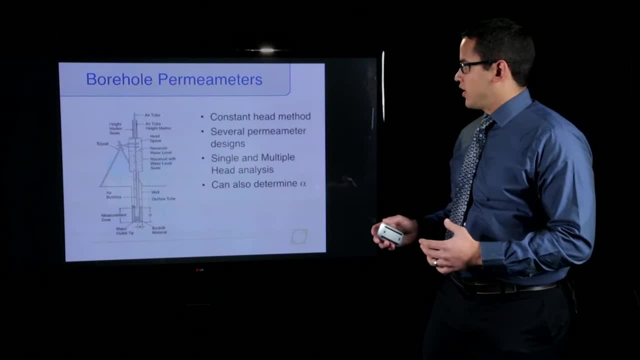 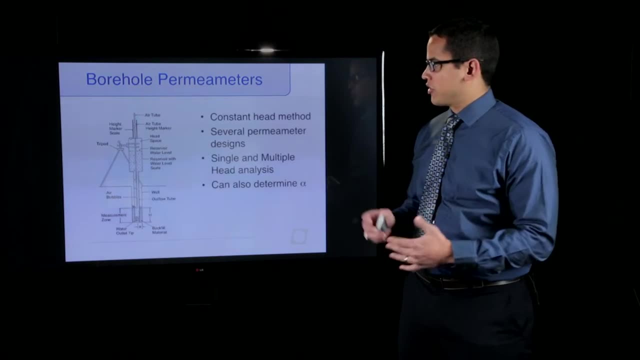 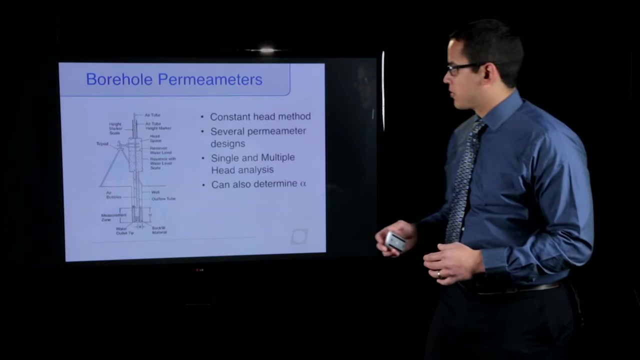 is the borehole permeameters, and here's kind of a diagram of a borehole permeameter. There are several permeameter designs out there. We won't go too in-depth into that, but we will talk about just kind of the, the basics behind the, the borehole permeameter With a borehole. 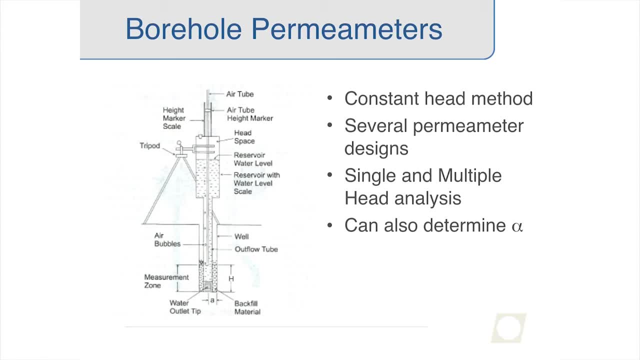 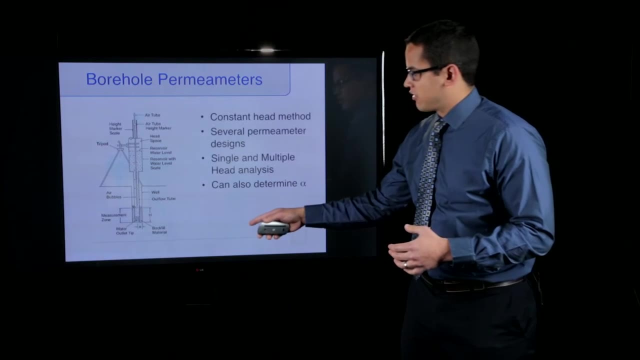 permeameter. you can only do the constant head method. at least only do it. what technique? well, because you're in the borehole, you can actually see what's going on. so the constant head method is is usually a better way to go because you can use, for example, and what they have in this design, they have a Marietta. 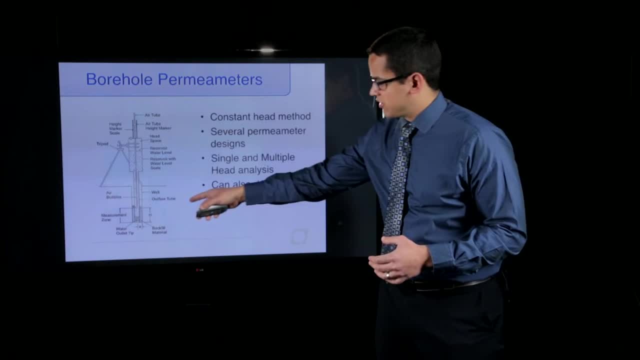 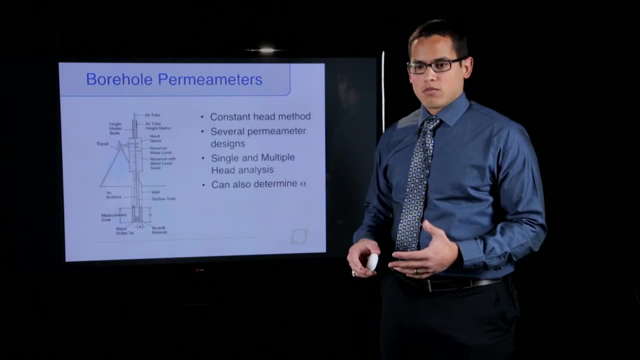 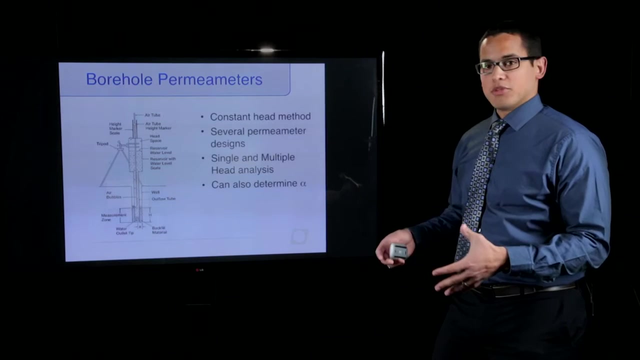 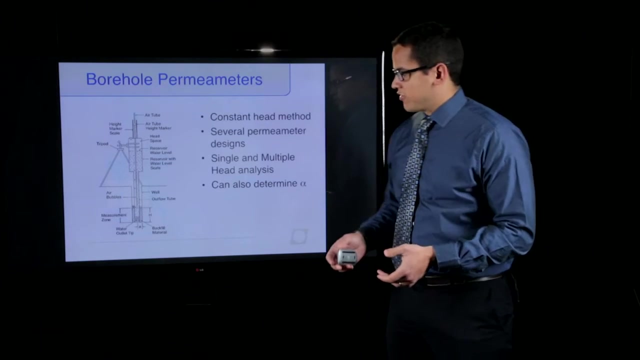 reservoir with a bubbler inside of the, in the, the auger hole, to actually control the, the pressure head, and then you can just measure the flow into the borehole to calculate your flow rates and then to measure and determine when you, when you come to steady state or quasi steady state for, for field methods. 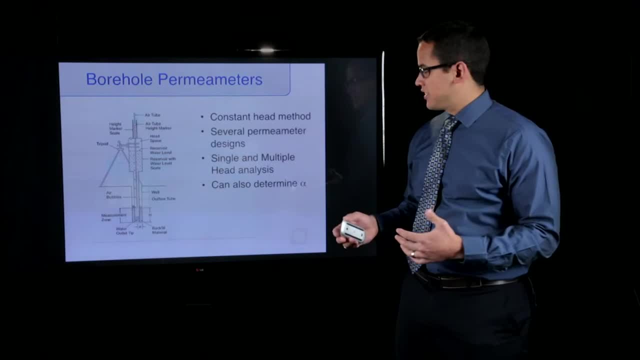 Another nice thing about the borehole permeameter is that it's not just a borehole permeameter. is that it's not just a borehole permeameter? is that it's not just a borehole? technique is just like with the pressure infiltrometer: you can do single and 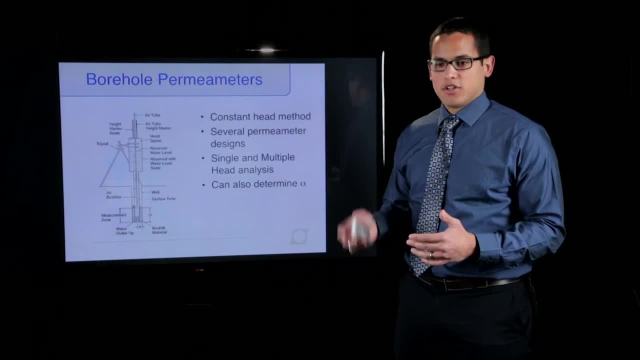 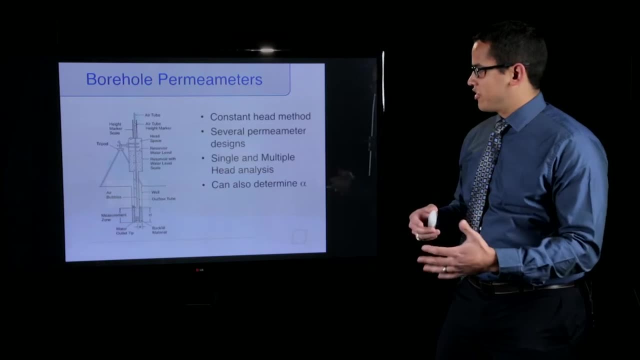 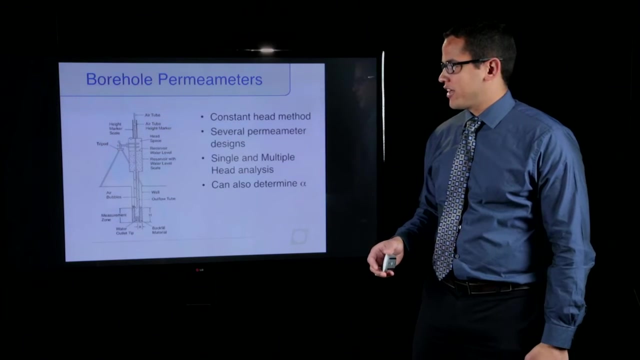 multiple head analysis by: by changing the water levels and the pressure head inside of the augered hole, and with this be just like with the pressure head infiltrometer, you can also determine the alpha values or the soil macroscopic capillary length factor. So just kind of how, how the borehole. 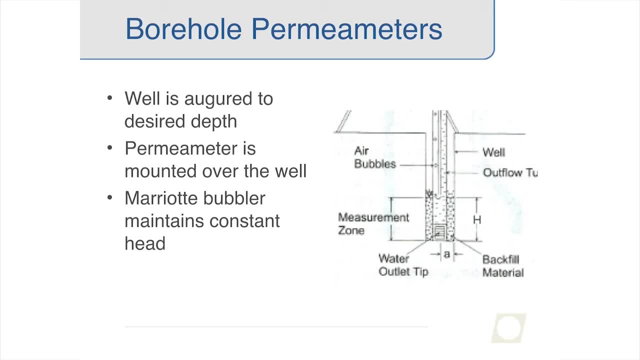 How the borehole permeameters work. you would auger a hole to a desired depth. Say you wanted to make a measurement at 30 centimeters. you would auger a hole down to 30 centimeters. The permeameter is then mounted over the well that you have augered. 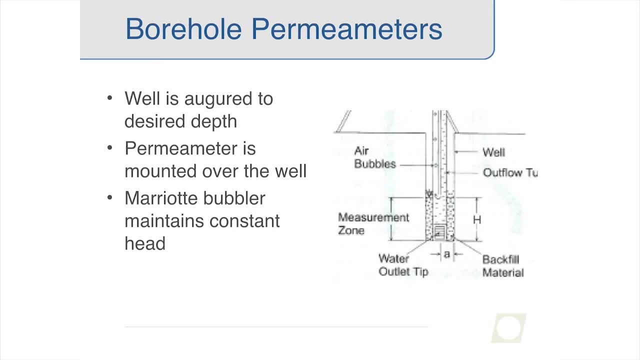 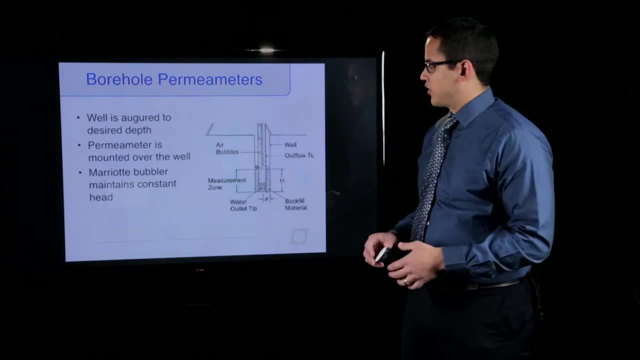 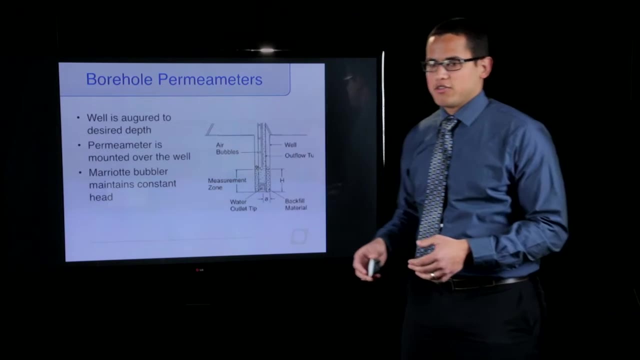 and the Marriott bubbler is inserted and maintains a constant head inside of the augered hole. and then you just calculate the inflow and wait for it to come to steady state and use those steady state values to calculate the hydraulic conductivity. And again, just like with the single ring technique and the pressure infiltrometer technique, 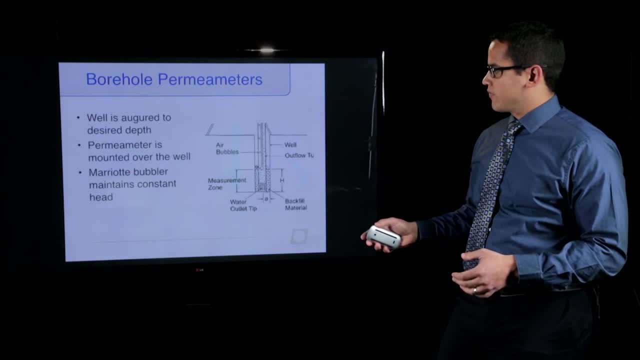 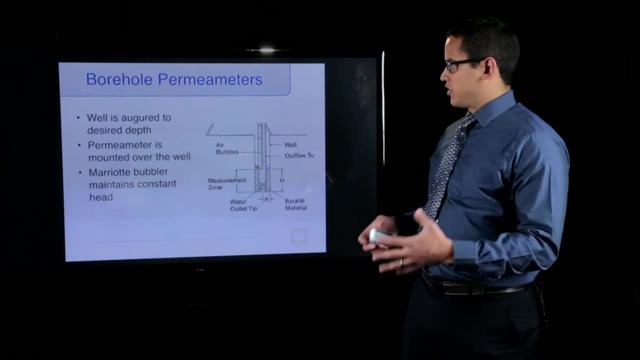 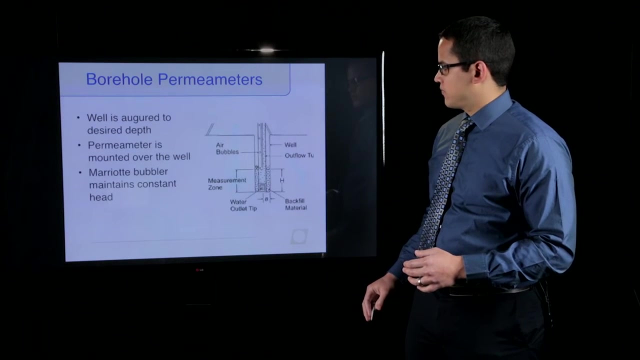 this is a three-dimensional flow technique, so you do have to correct for three-dimensional flow which, using that multiple head analysis to get the alpha value, improves your estimation of hydraulic conductivity. Some of the advantages of the borehole technique again are: 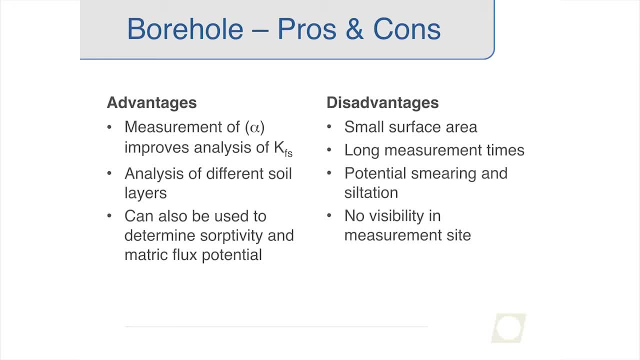 one, you get the measurement of alpha, which improves your analysis of the field-saturated hydraulic conductivity. Another advantage of this technique versus the ring infiltrometers is it's fairly easy to take measurements of different soil layers, because all you're doing is augering a small hole. 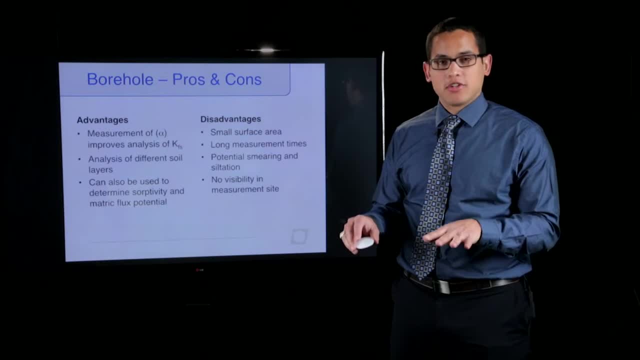 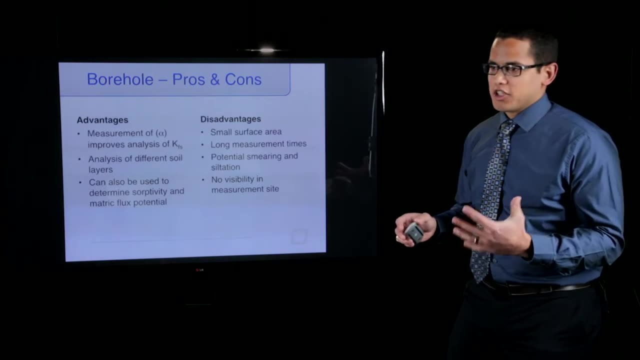 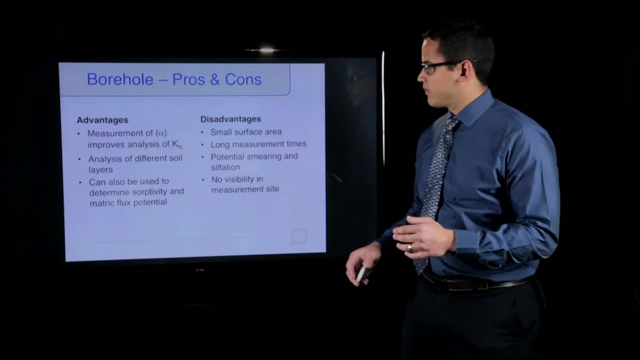 If you're wanting to do that with a ring infiltrometer, you would have to excavate a much larger hole And get down to that layer that you were wanting to measure, which is going to be a little more labor-intensive. So with this borehole technique, you can get actual measurements of different layers fairly easily. 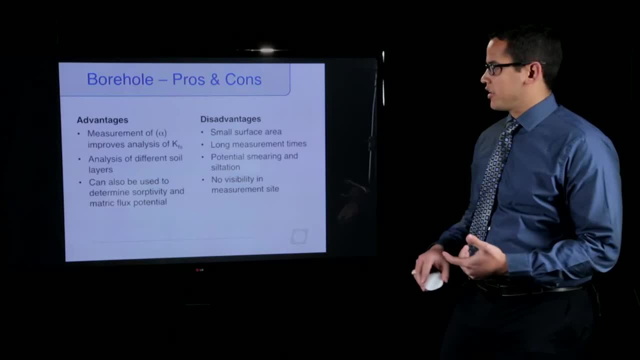 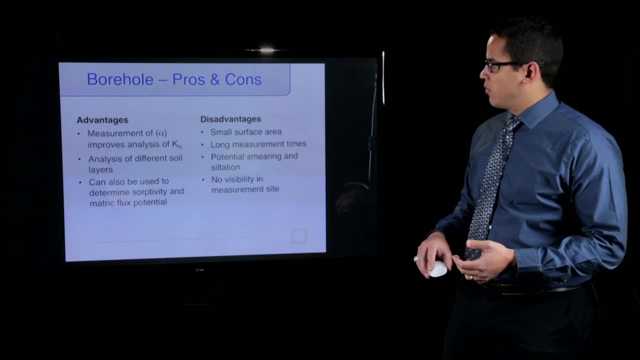 And, just like the pressure infiltrometer technique, it can also be used to determine sorptivity and matrix flux potential. Some of the disadvantages of the borehole technique: it is a small surface area and it's not a large hole. It's just a small surface area that you're measuring. 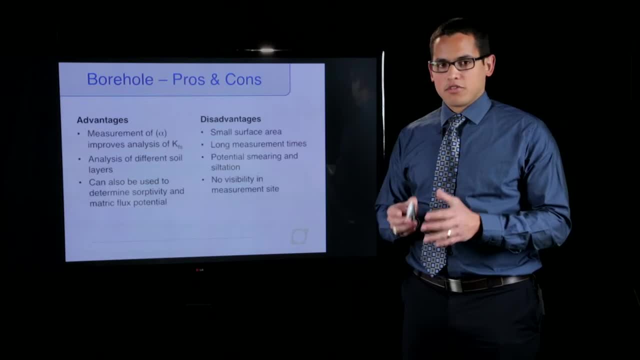 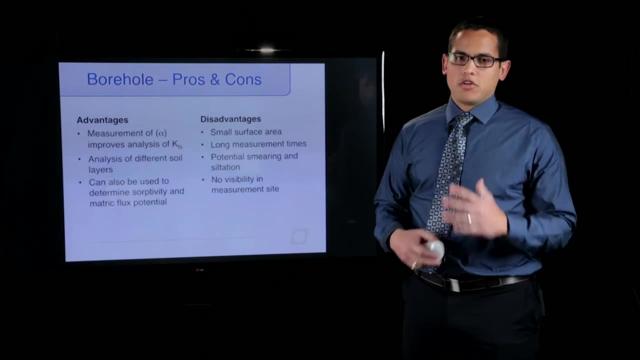 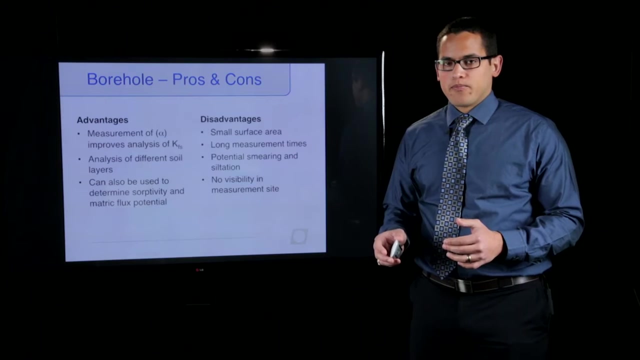 Just like with the small core samples that you would bring back to the lab. you don't completely encompass spatial variability very well, So you typically will want to make more measurements to get a better representation of your field. Just like the other field techniques, there are long measurement times. 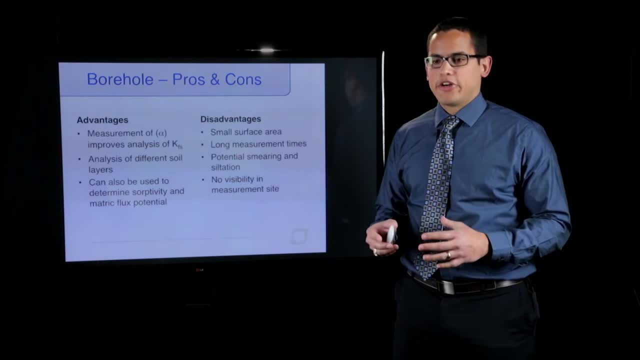 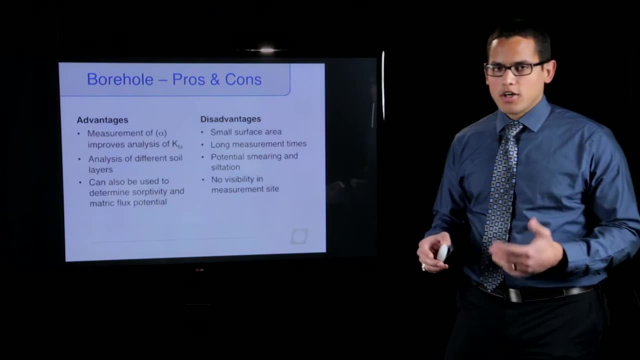 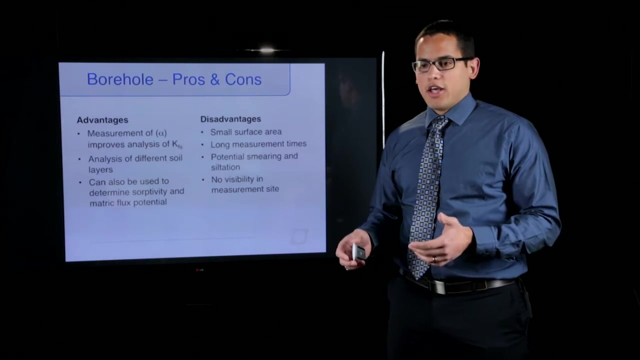 Maybe not as long as a large ring infiltrometer due to the smaller area, But it does take some time, Especially if you're doing the multiple head analysis. One of the other issues with the borehole technique is the potential for smearing or siltation inside of the borehole. 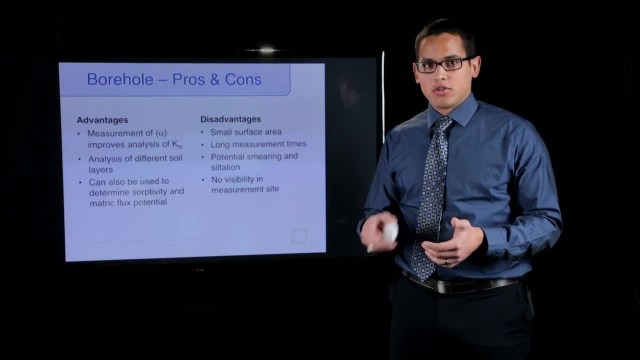 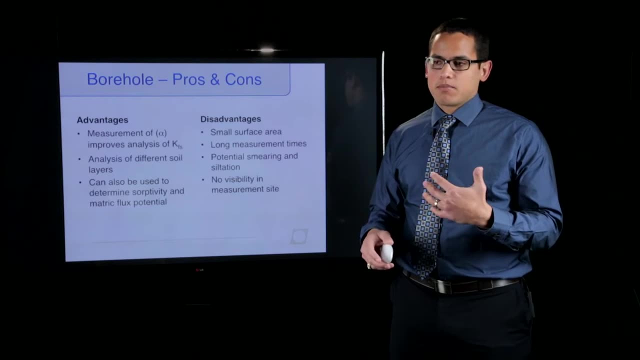 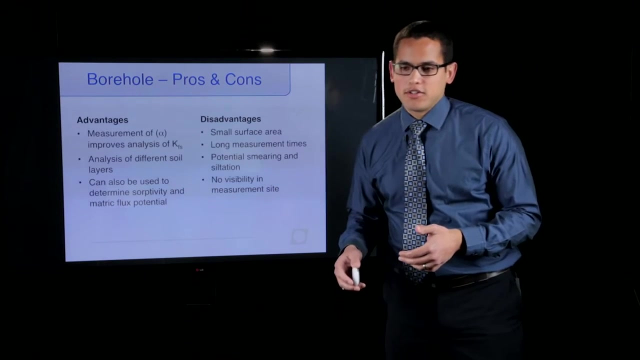 And what I mean by smearing is, as you're augering the hole, you could potentially smear the surface, which would then close off pores, making them unable to conduct water, which then would cause you to underestimate hydraulic conductivity. And one of the other disadvantages of this technique is there's no actual visibility down in the measurement site. 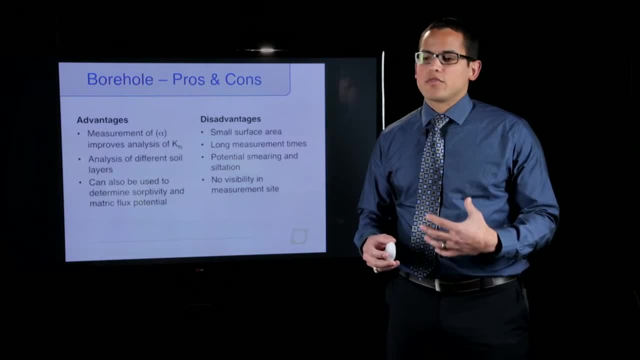 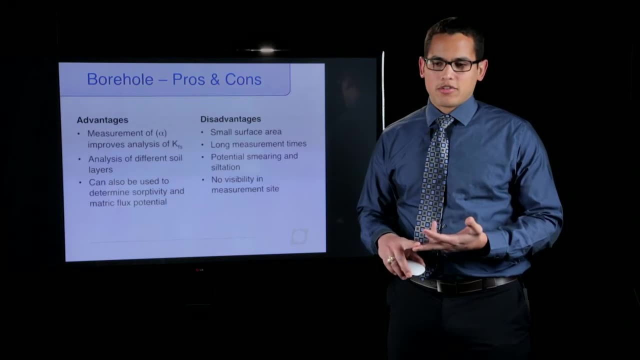 So you can't really see what's going on. So you're just kind of hoping everything that is working right and that you haven't smeared it or you aren't having siltation. There are approaches that you can take to decrease these issues. 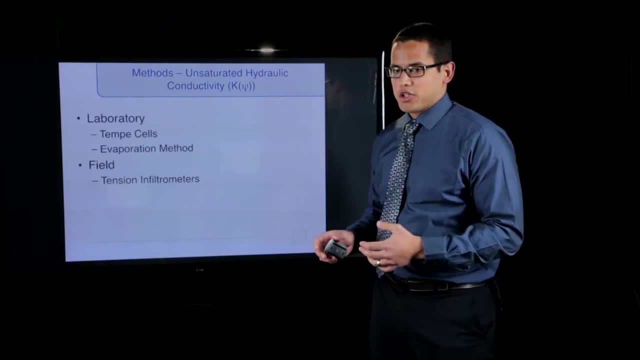 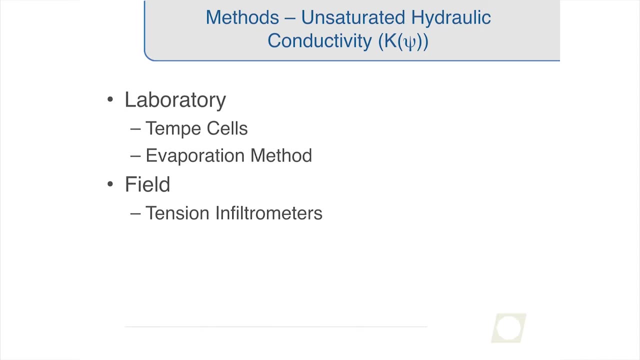 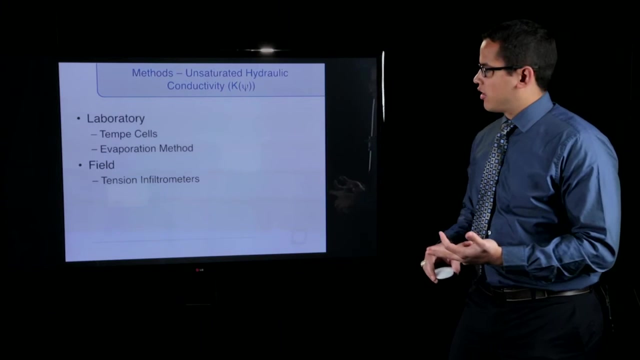 Alright, so that's it for saturated hydraulic conductivity, But now let's focus on unsaturated hydraulic conductivity, Or KSI. We'll focus on laboratory methods using flow cells and the evaporation method, And then we'll focus on the field techniques. 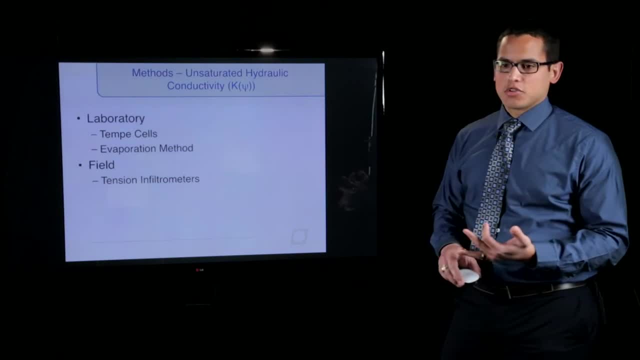 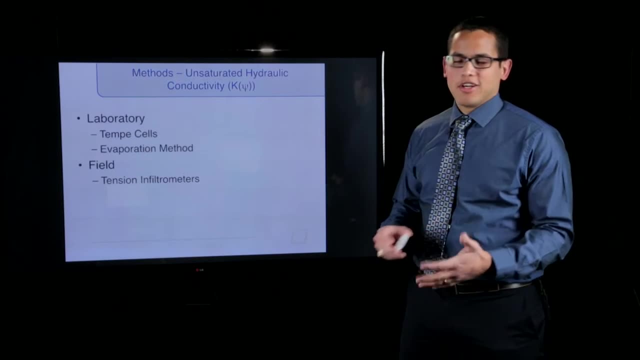 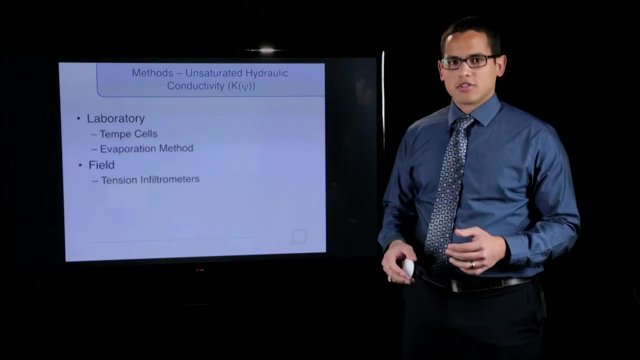 The one that we'll primarily focus on is tension infiltrometers. There are other techniques for unsaturated hydraulic conductivity as well as saturated hydraulic conductivity. We're not going to focus on them in this presentation, just due to time, And these are some of the more popular techniques for measuring hydraulic conductivity. 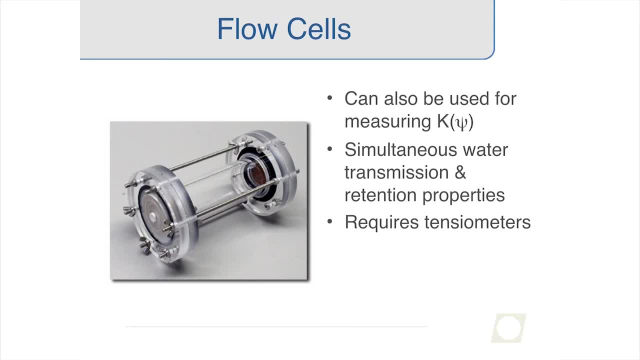 So flow cells can also be used to measure unsaturated hydraulic conductivity as well as saturated hydraulic conductivity. Now, the nice thing about using flow cells to measure unsaturated hydraulic conductivity is due to the approach and the way it's done, is you're getting not only water transmission parameters. 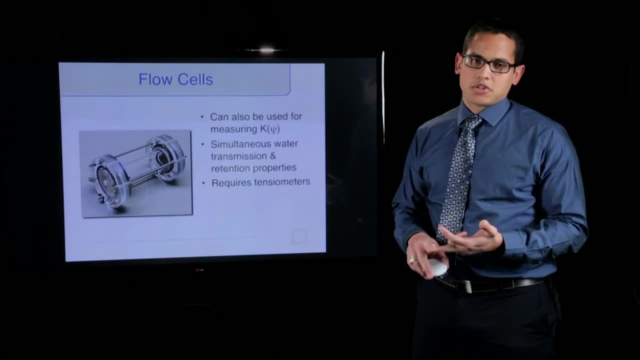 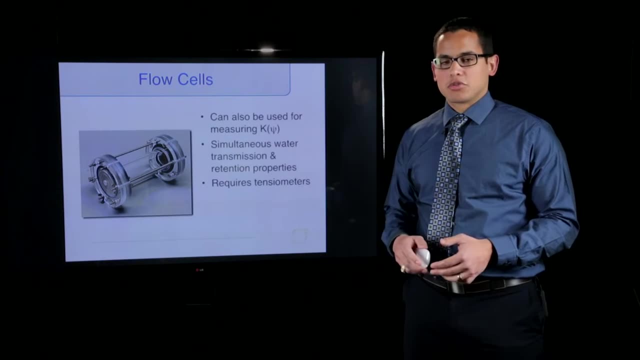 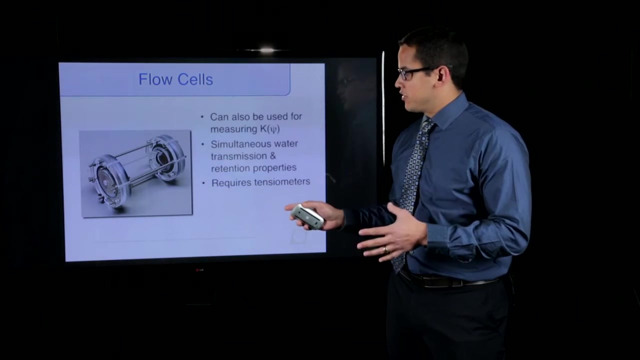 so the unsaturated hydraulic conductivity, you are also getting retention properties at the same time, which can be very useful. Essentially, it would allow you to generate part of the soil moisture release curve. Now, when trying to do unsaturated hydraulic conductivity in flow cells, 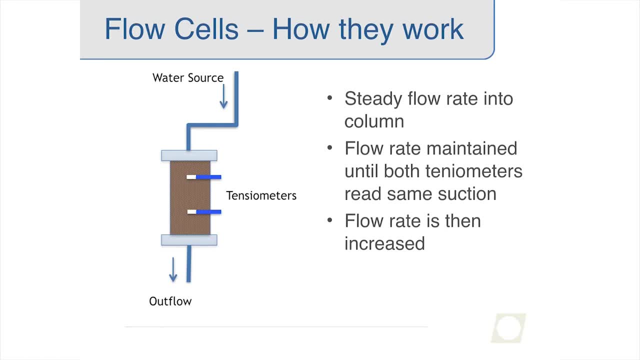 it does require tensiometers. So here's an example of kind of how that would work. So, just like with the, just like with the saturated technique with flow cells, you have a water source coming in, then you have water flowing out of the soil core. 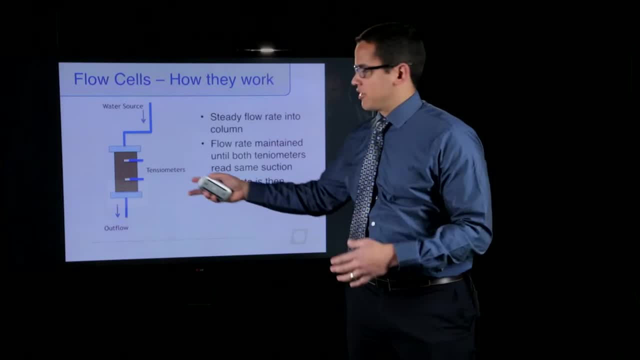 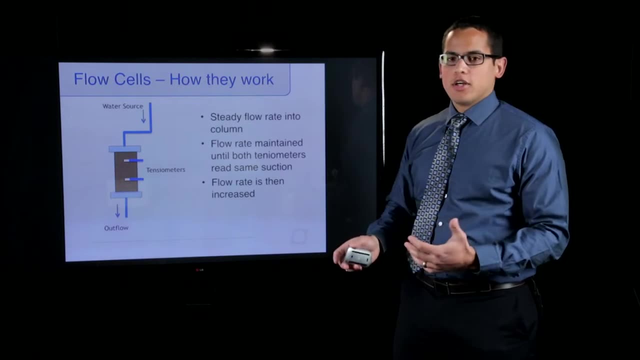 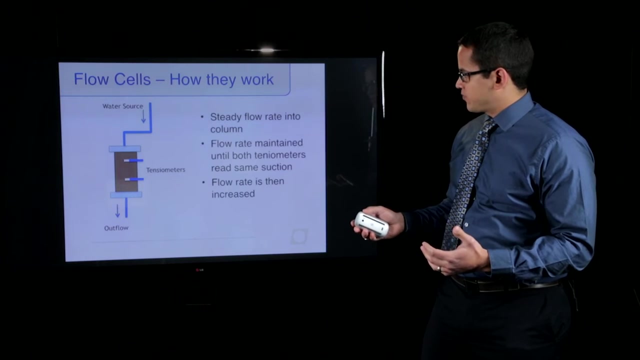 One of the differences is you have, typically, one of the techniques is using two tensiometers at different points in the core. You're monitoring the matrix potential or the water potential at those different points. Now, one of the differences between this technique: 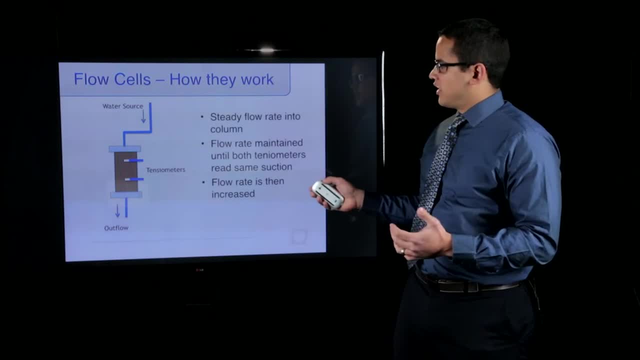 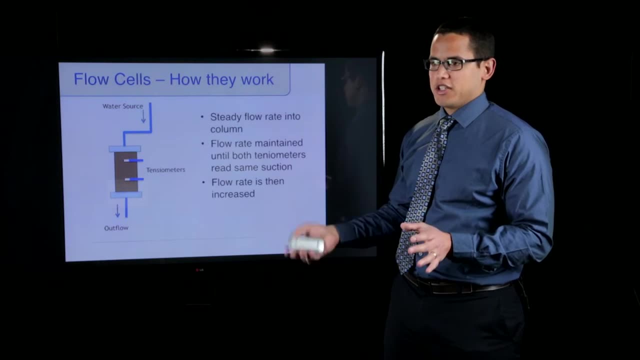 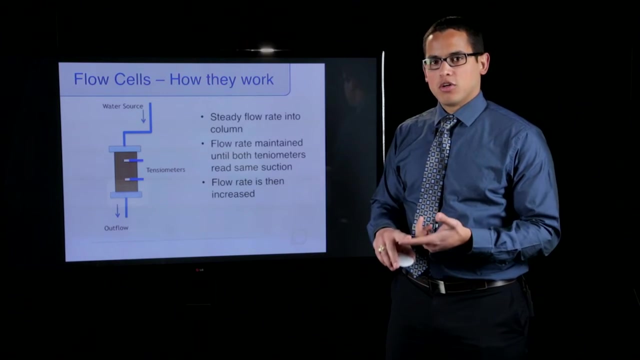 and using flow cells for saturated hydraulic conductivity is. what we want to do now is, instead of having just a constant head or a falling head technique where we just have a lot of water coming in, now we actually want to control the flow rate, So we want to be able to control low to high flow rates inside of the soil core. 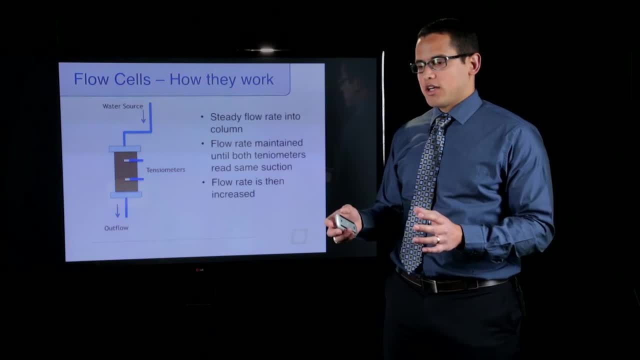 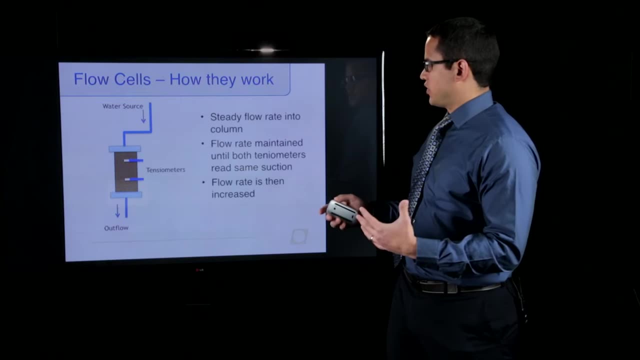 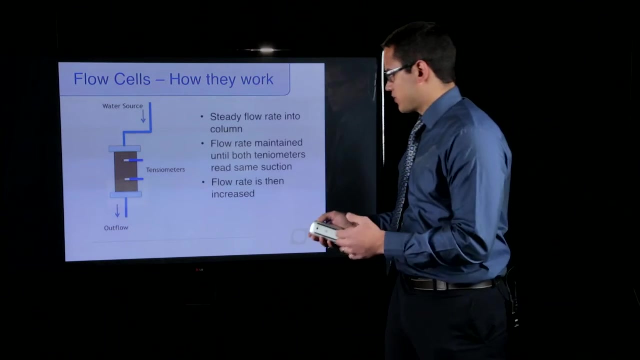 to actually allow the soil to transmit water in unsaturated conditions, And essentially, what you're doing then is you maintain a certain flow rate until both tensiometers are reading the same suction or the same matrix potential, And once this point has been reached, 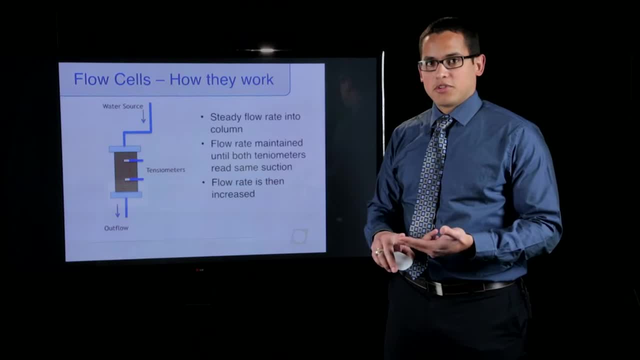 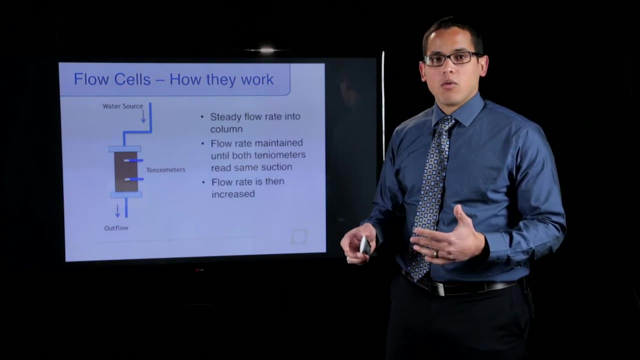 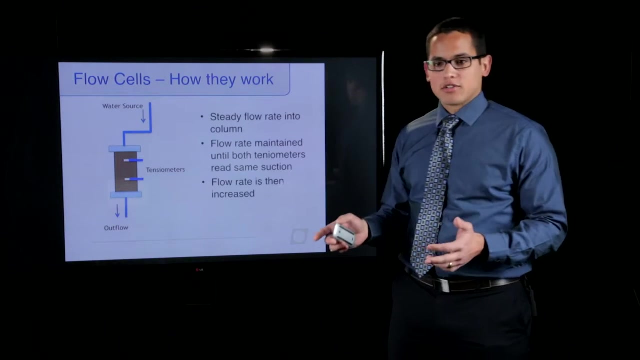 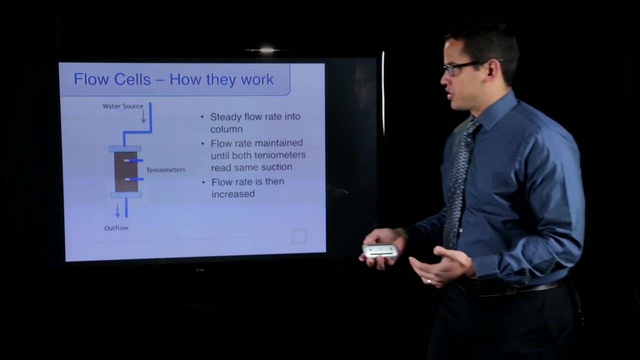 then you can measure, then you can use those simultaneous suction measurements or matrix potential and the actual flow rate coming in, to determine what the unsaturated hydraulic conductivity was at that specific potential. And then, if you were wanting to get the retention properties, you would also want to measure water content as well of that soil core. 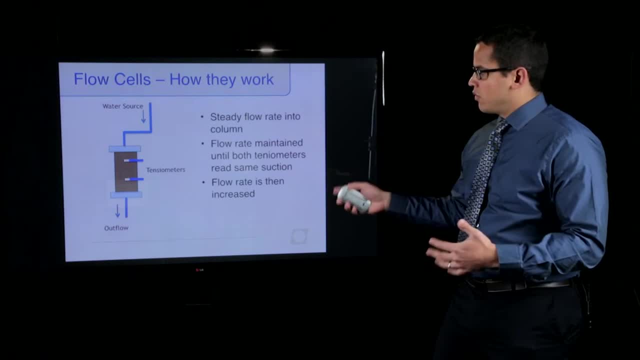 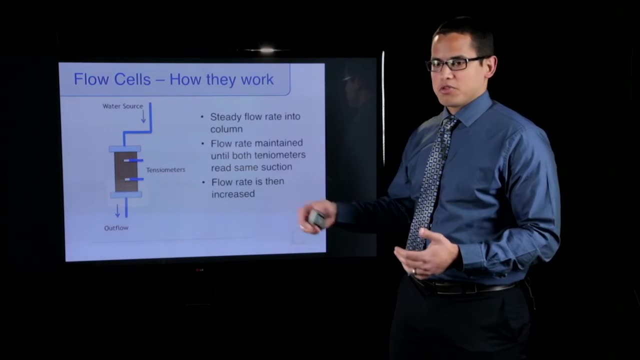 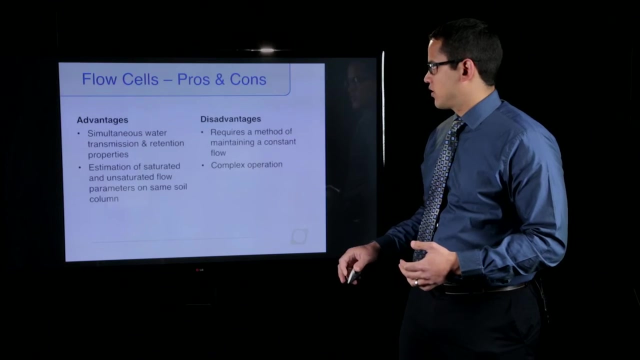 Once you reach the equilibrium between those two tensiometers, at that point you'll then increase the flow rate to get the next point and you'll have to do this multiple steps to get different points along the unsaturated hydraulic conductivity curve. So some of the advantages of using flow cells to measure. 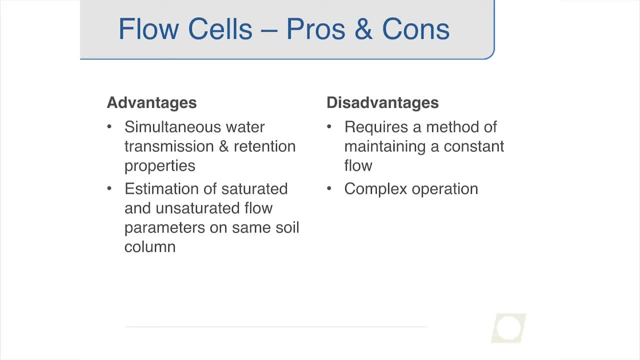 hydraulic conductivity or unsaturated hydraulic conductivity is, again. you get simultaneous water transmission and retention properties, depending on how you set this up, which can be very useful, especially when you're trying to get a full characterization of hydraulic properties of soil, Along that with flow cells. 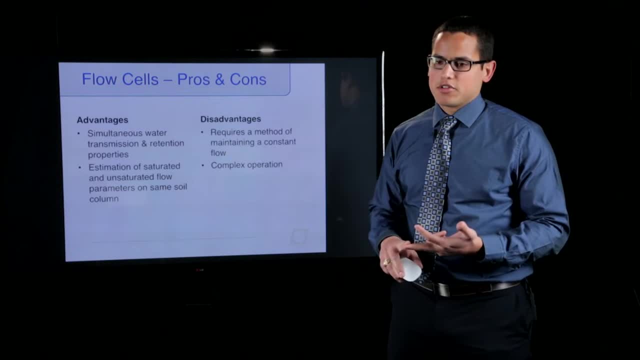 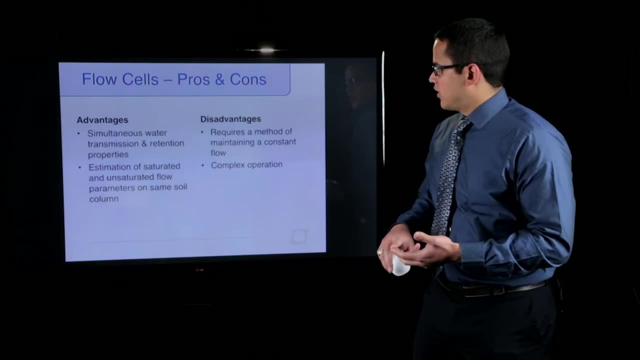 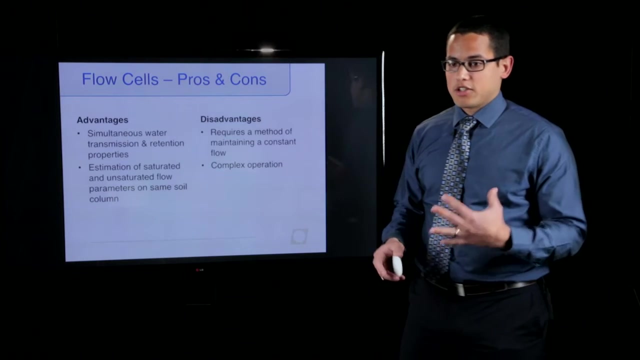 you can estimate both saturated and unsaturated flow parameters on the same soil column, So that's a nice approach to be able to take. Some of the disadvantages with this technique is it does require a method of maintaining a constant flow, and so you have to have some type of pump. 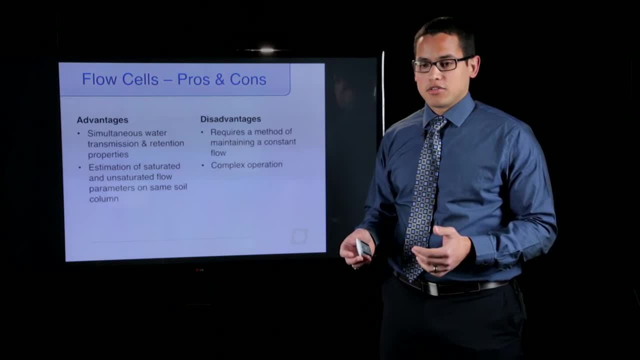 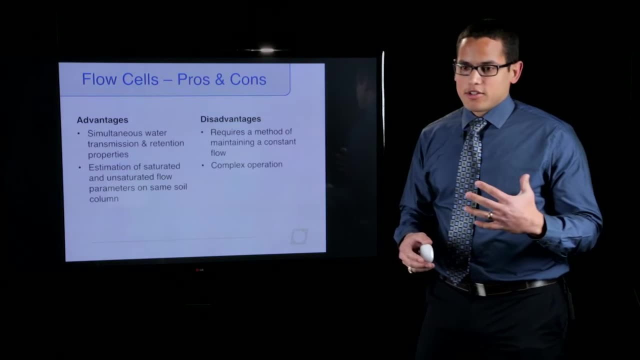 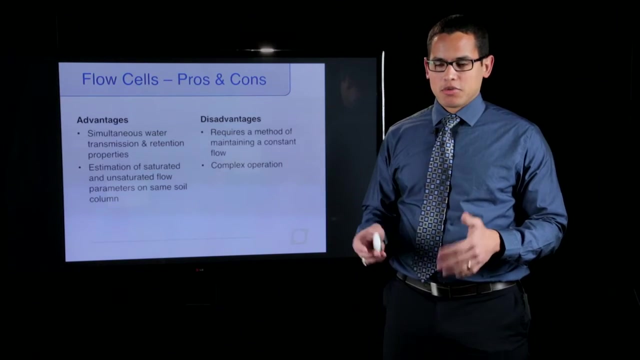 that's controlling the flow into the soil core, and be able to actually change those different flow rates. So again, just like with the saturated technique, this is also going to take up some space in the lab and for automation it requires some fairly complex instrumentation. 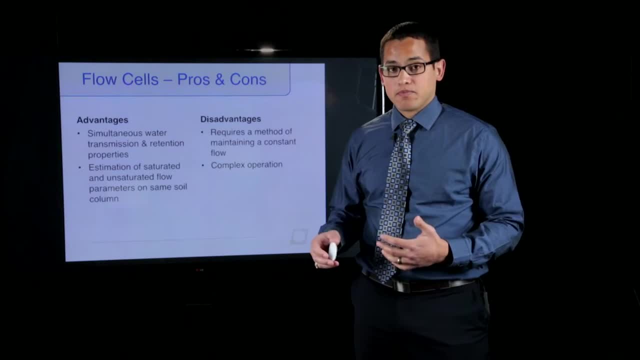 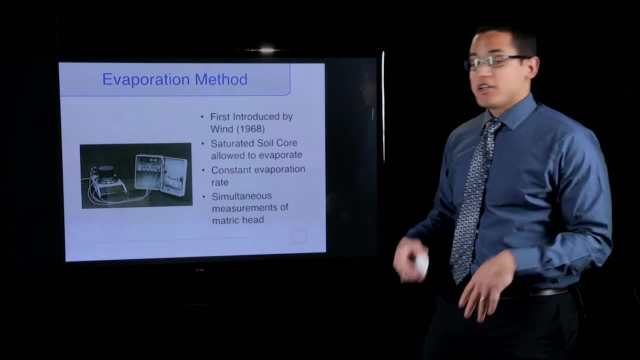 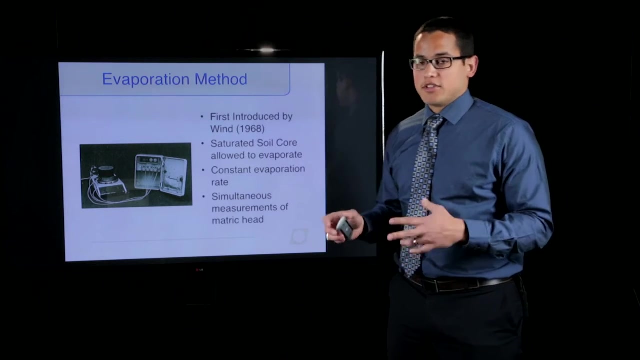 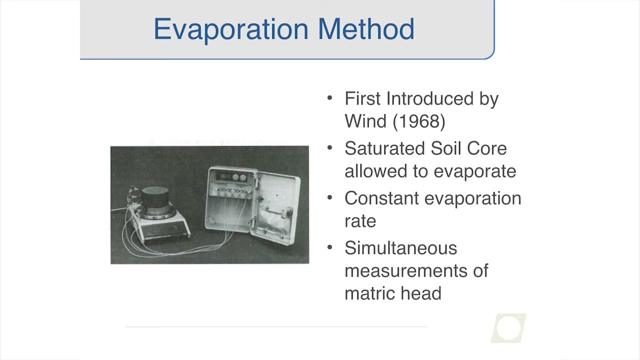 and it is a little more complex operation than doing saturated hydraulic conductivity Now. one of the other techniques for measuring unsaturated hydraulic conductivity is the evaporation method. This was first introduced by WEND in 1968, and here's an example of one of the earlier systems. 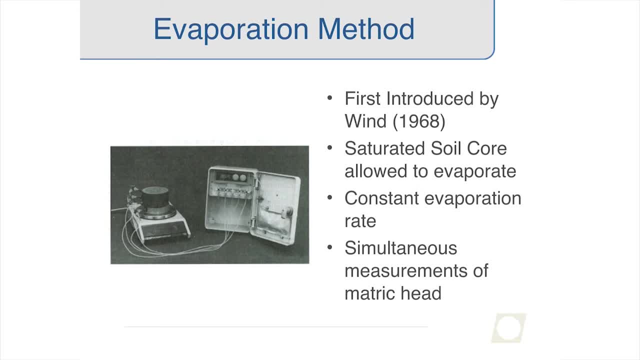 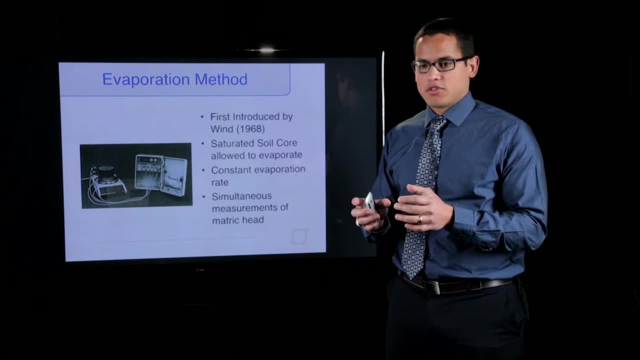 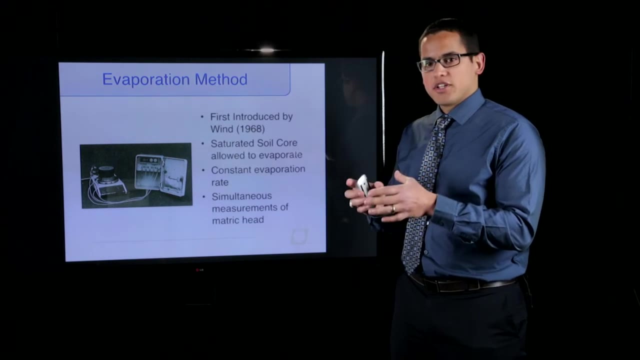 designed for measuring unsaturated hydraulic conductivity based on the evaporation method. Essentially, what you have is a soil core with tensiometers inserted into it at different depths. The core starts off initially saturated, and it is open at the surface and closed at the bottom. 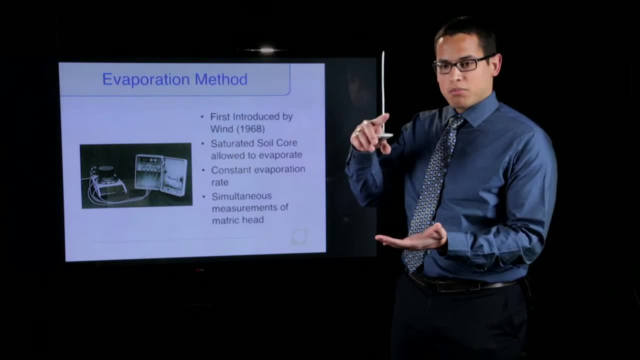 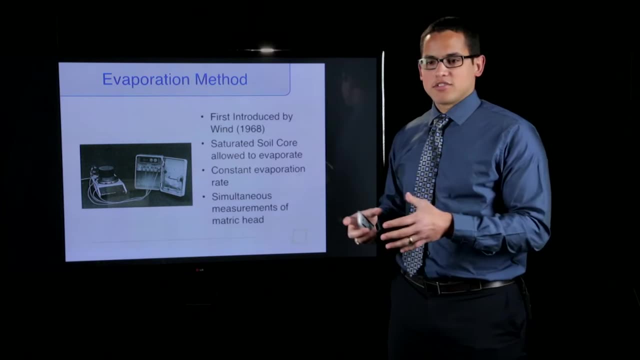 So the water can only evaporate from the surface and what happens is you get a gradient in the mature potential in the core and if you're measuring the mass of the soil core as it evaporates over time, and you get the gradient, 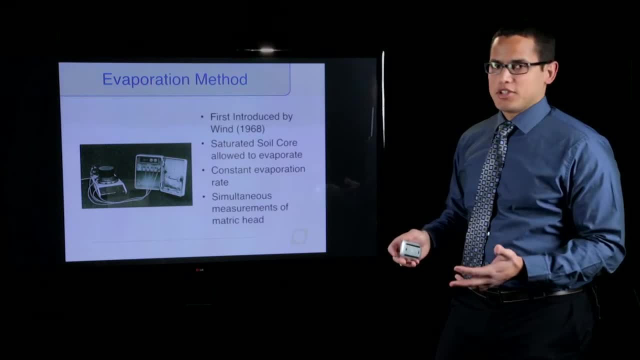 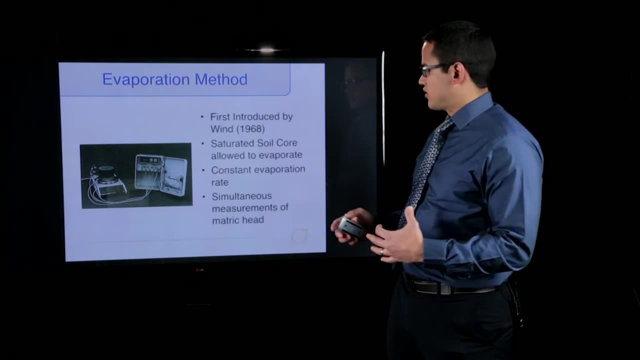 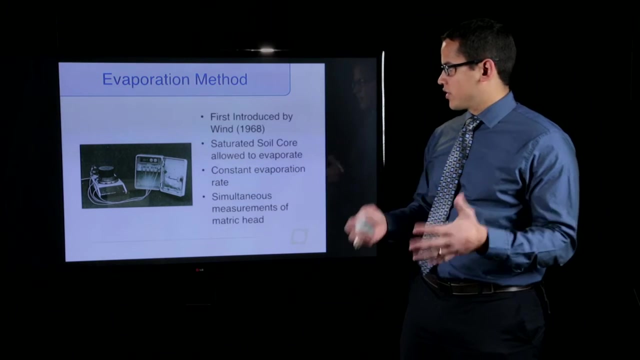 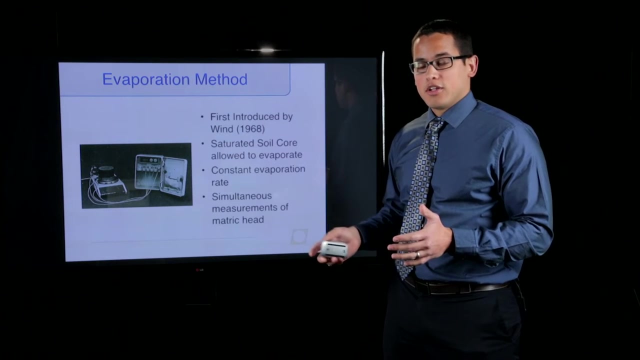 then you can calculate the mature flux potential or the unsaturated hydraulic conductivity. This technique does require a constant evaporation rate and along with that, because we're getting simultaneous measurements of matric head and water content, we can also do the retention properties. 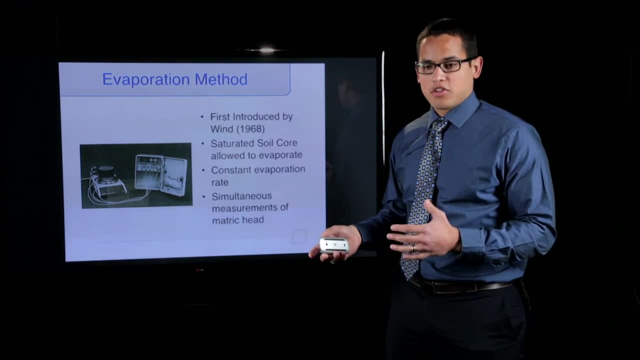 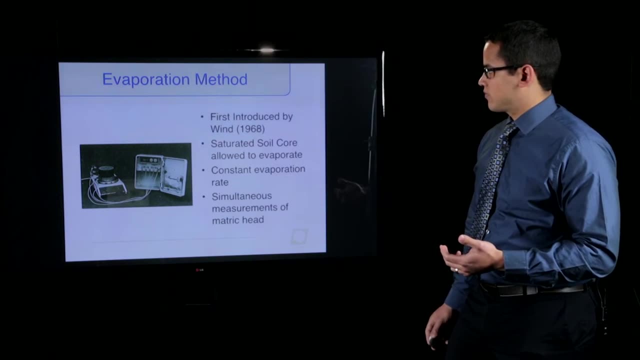 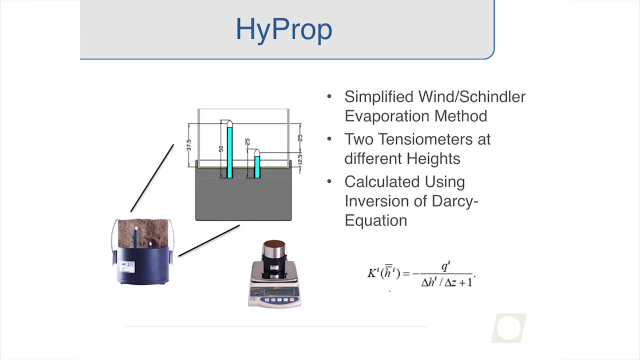 of the same soil core. So, just like with the flow cell technique, we can do unsaturated hydraulic conductivity and generate the soil moisture release curve. So here's a device that was developed based on that technique, except it was simplified. so it's based on the simplified. 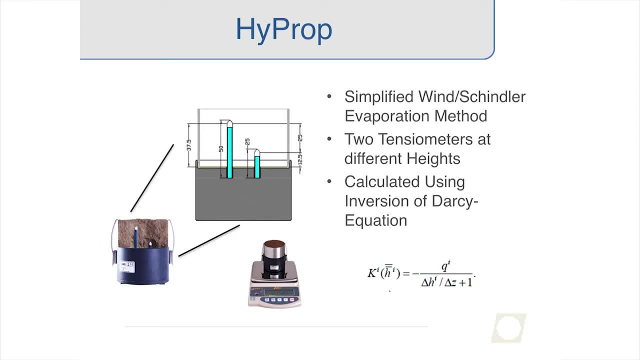 Winn-Schindler evaporation method and this device is the HyProp, And with this instrument you have two tensiometers at different heights inside of a soil core and, just like we talked about earlier, it's only open at the surface. 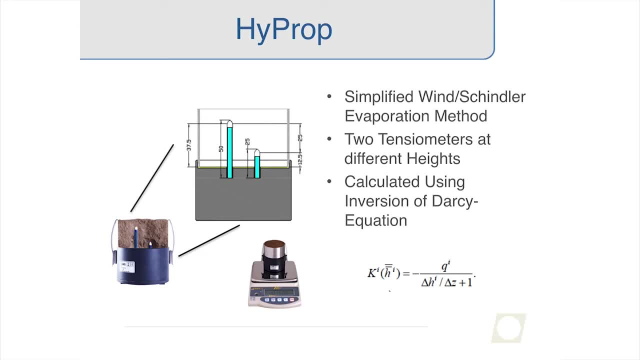 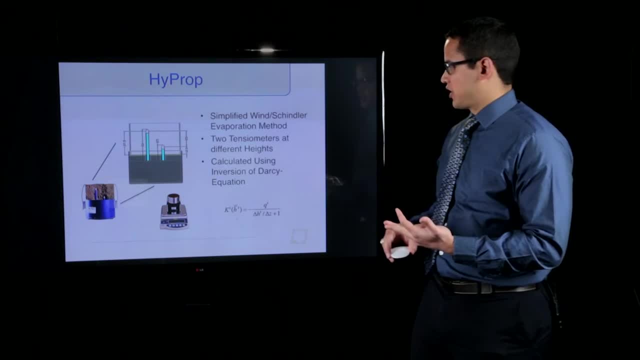 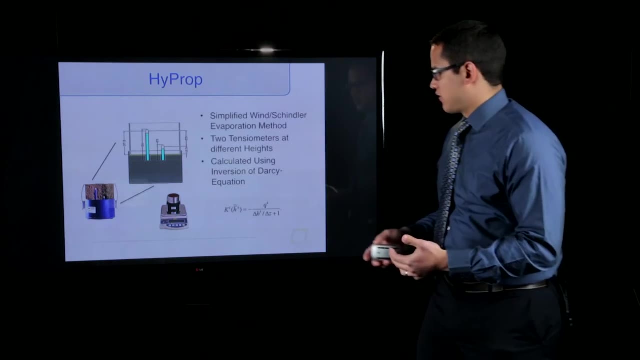 and the HyProp sits on a scale over time and measures as the soil core evaporates and generates both the retention properties and the unsaturated hydraulic conductivity. And the unsaturated hydraulic conductivity is calculated using the inversion of the Darcy equation and you can see an example of that here. 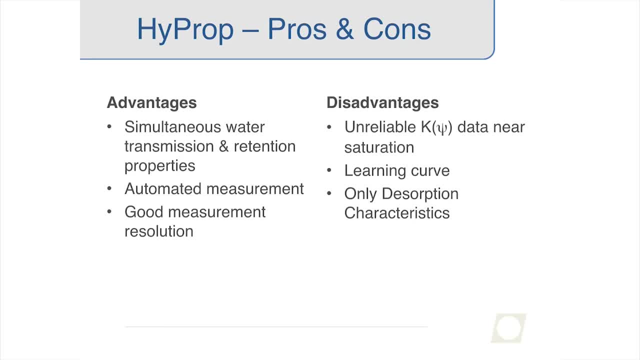 So some of the advantages of the HyProp: you do get simultaneous water transmission and retention properties, just like we said. One of the other main advantages of the HyProp versus, say, the flow cell technique is this is a completely automated measurement. 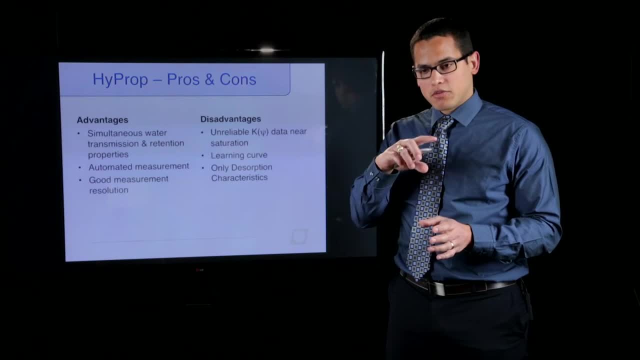 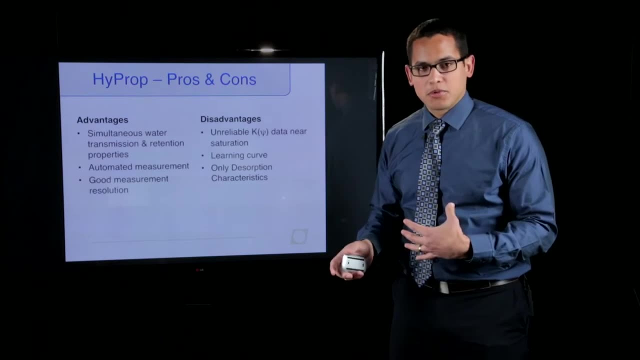 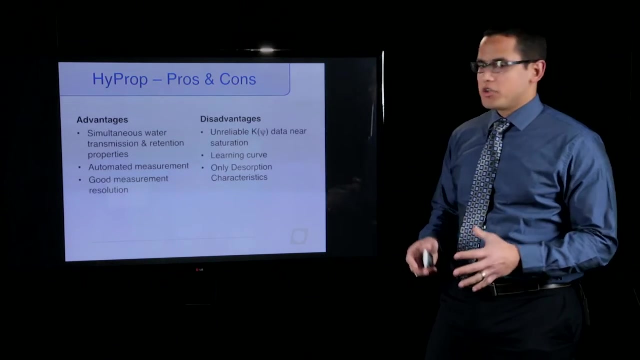 throughout the full range, and so we actually generate the curve for unsaturated hydraulic conductivity by doing this, which is just kind of a more simple technique and more automated and requires less intervention than some of the other techniques, And you do get good measurement resolution. 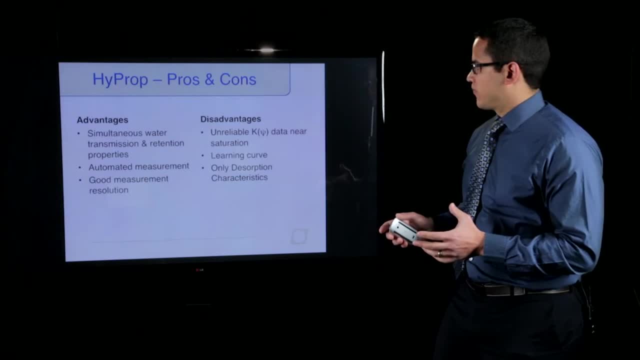 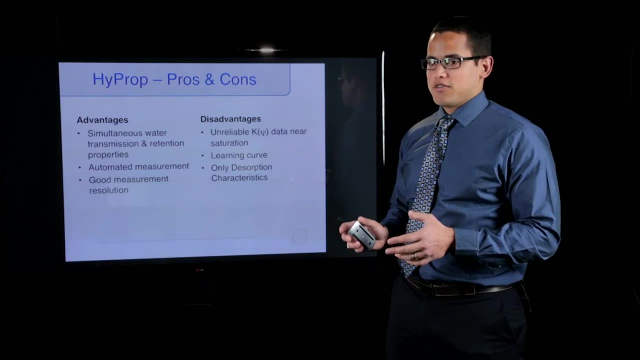 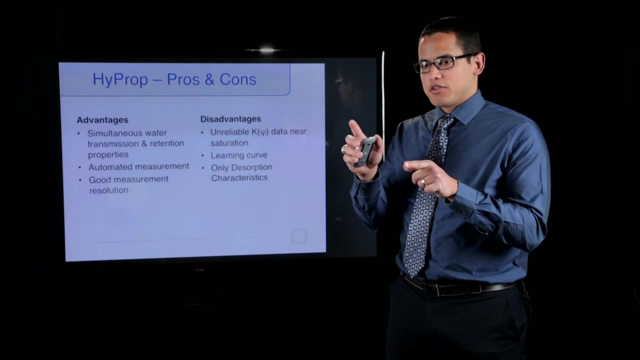 except for near saturation, And so one of the disadvantages of this technique is you do have unreliable, unsaturated hydraulic conductivity data near saturation, And the reason for that is typically near saturation. you have very little differences between the drying gradient and the top and the bottom tensiometer. until you reach a certain point, And this varies for different soil types. Typically, for finer textured soils we can actually get better measurements of unsaturated hydraulic conductivity, closer to saturation, than with coarser textured soils. The HyProp does have a little bit of learning curve. 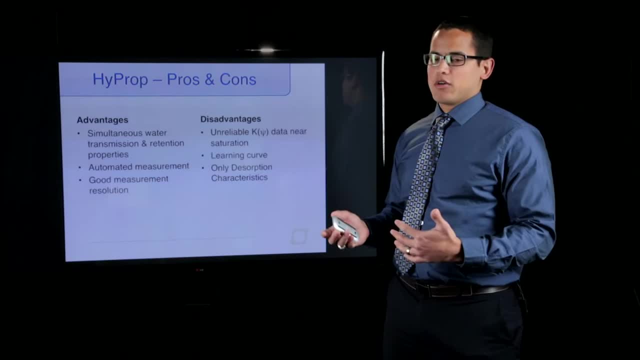 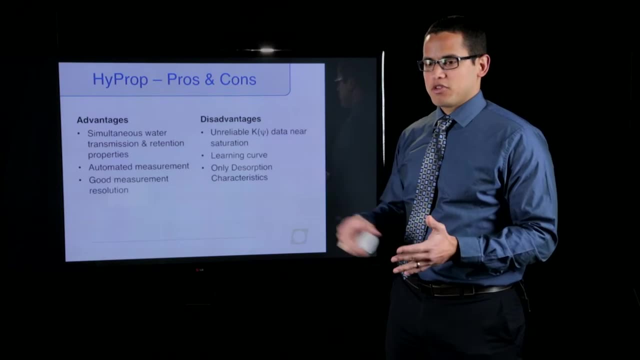 because you do have to learn how to fill tensiometers and how to work with this type of instrument, But once you do figure that out, it is a very easy setup and once it's set up it's completely automated. One of the other disadvantages of this is: 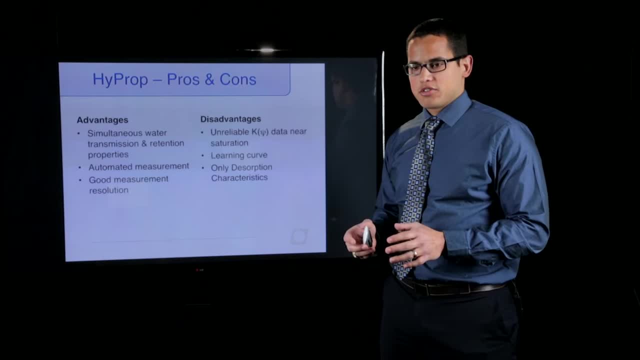 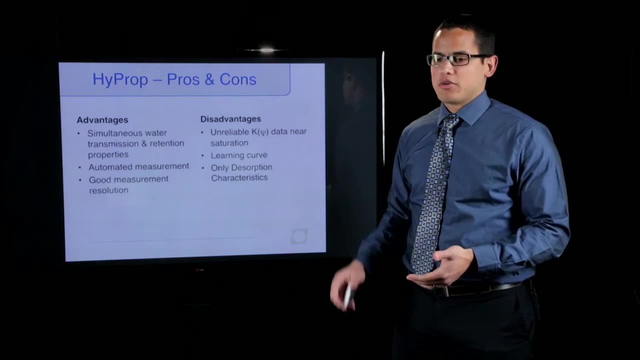 you're only doing desorption characteristics, So you can have some differences from adsorption characteristics, where you're adding water, whereas in this case you're actually evaporating water and losing water, So you might have some slight differences there. Okay, now we'll focus on the field techniques. 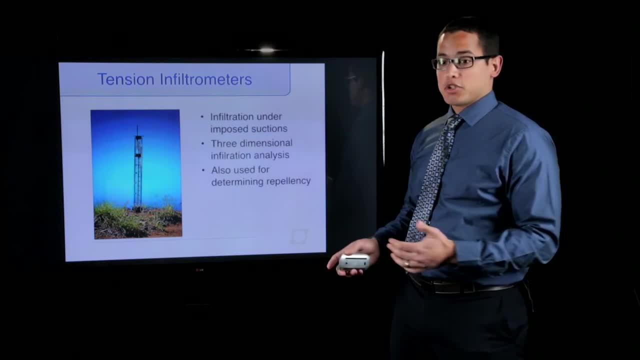 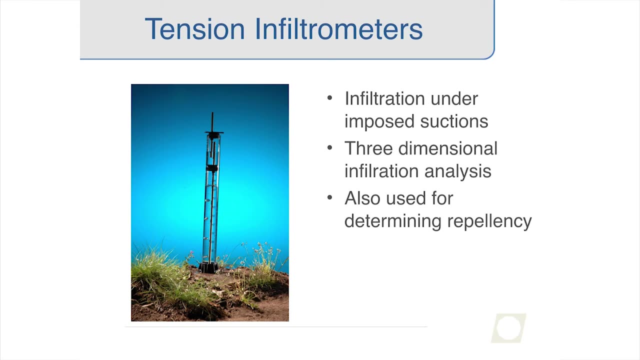 And the one field technique that we were going to talk about is tension infiltrometers. So essentially, what a tension infiltrometer does is it infiltrates water into the soil under imposed suctions, And so you can actually change the suction and measure the infiltration rates. 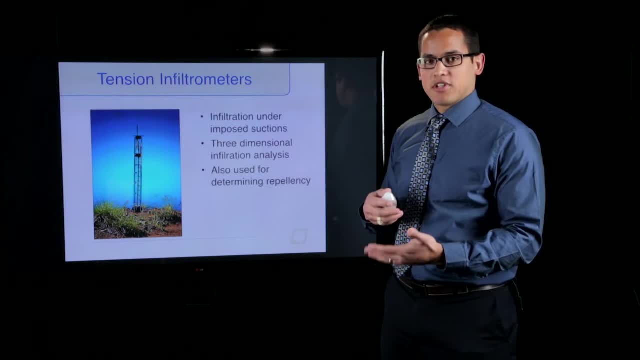 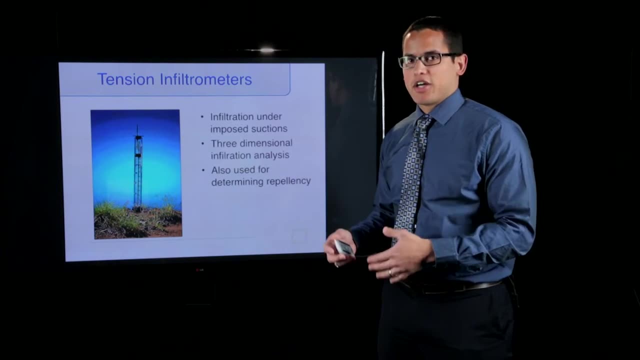 at different negative suctions to segregate different pore sizes. So the higher the suction, the smaller the pores have to be to actually pull water out of this infiltrometer. And so one of the things to make sure people understand is with tension infiltrometers. 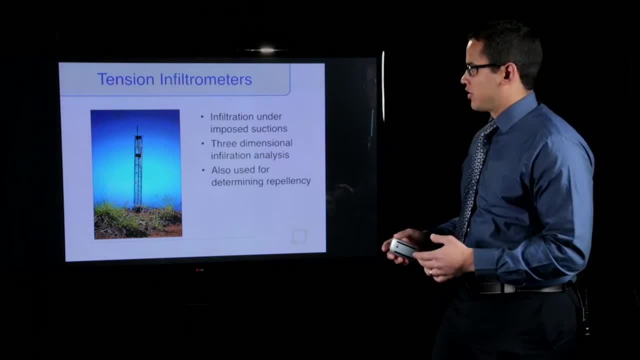 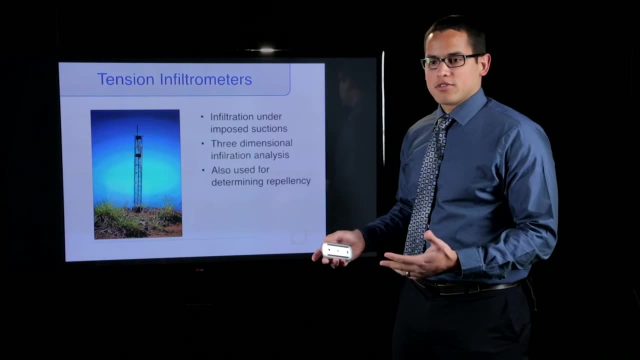 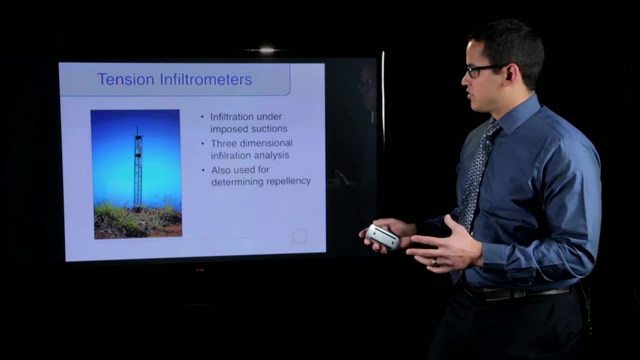 you cannot measure saturated hydraulic conductivity. You can only measure unsaturated hydraulic conductivity. This is a three-dimensional infiltration technique, so it requires three-dimensional analysis of flow, And one of the nice things about tension infiltrometers is they can also be used to determine repellency. 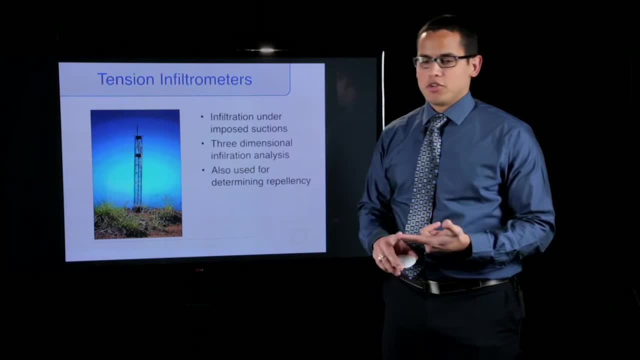 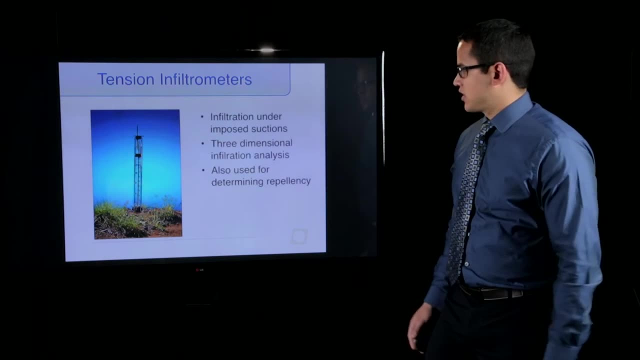 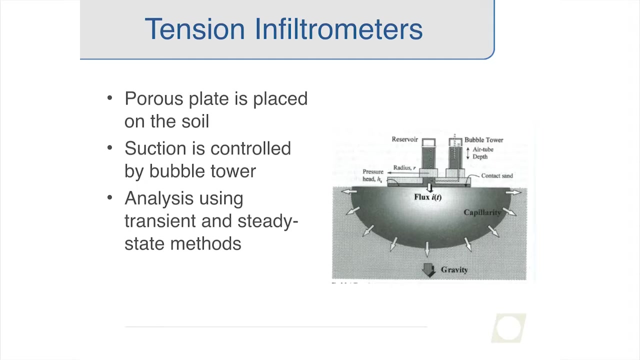 And this is really useful for people that are doing hydrophobicity studies, especially in post-forest fire situations, And this is a common application of tools like this. So, essentially, how a tension infiltrometer works is you have a porous plate. 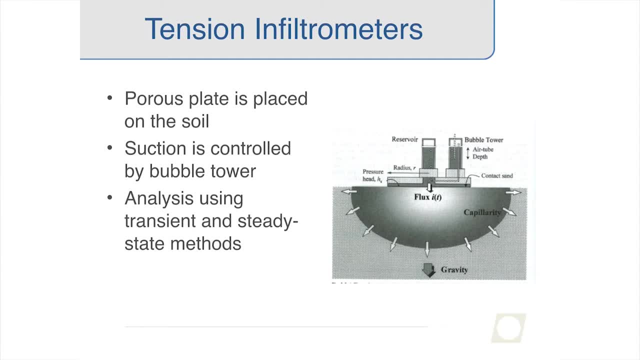 that's placed on the soil. You can see an example of that here. The water is pulled out of the soil and in three dimensions it's going to be higher flow down just due to gravity. The suction is controlled by a bubble tower. 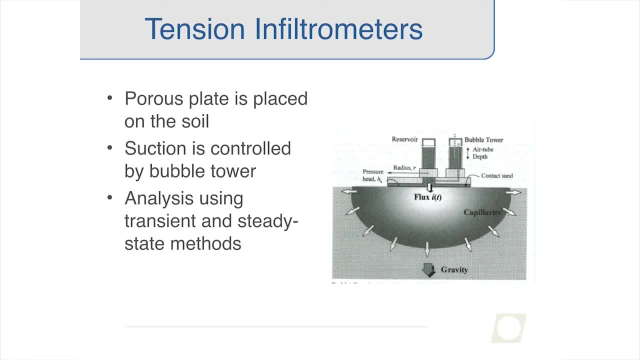 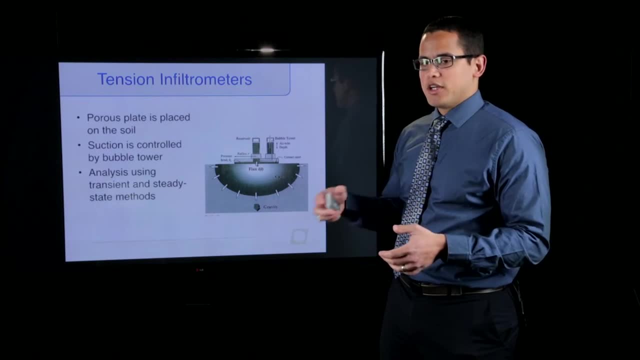 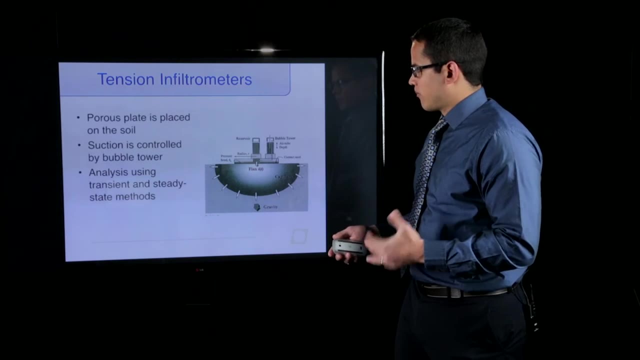 which has essentially a Marriott bubbler in it as well, And it actually, then, is controlling negative suction, And you control this typically by inserting the bubble tube deeper into the water to raise the suction that's required to pull water through the device With the tension infiltrometer. 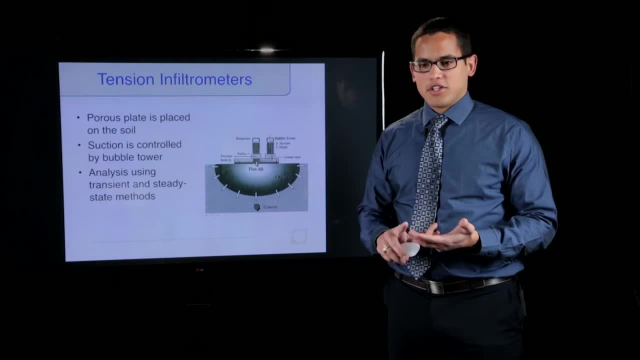 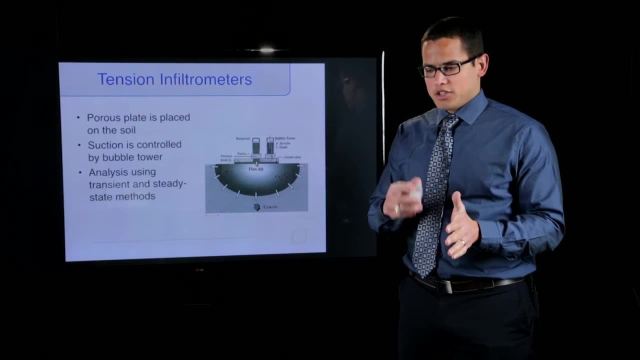 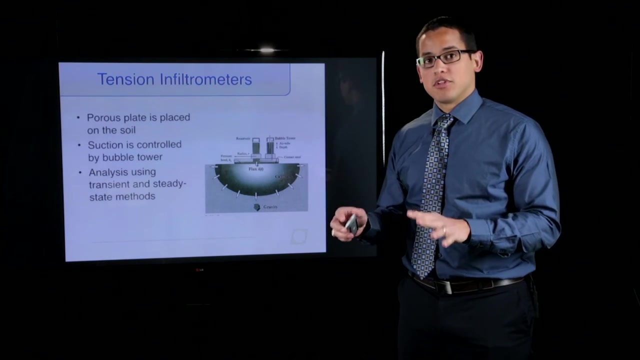 you can have analysis using transient and steady state methods, And essentially what that means. what a transient method is is you start taking your measurement and continuously measure the infiltration rate as it changes over time, And you don't have to reach steady state with this technique. 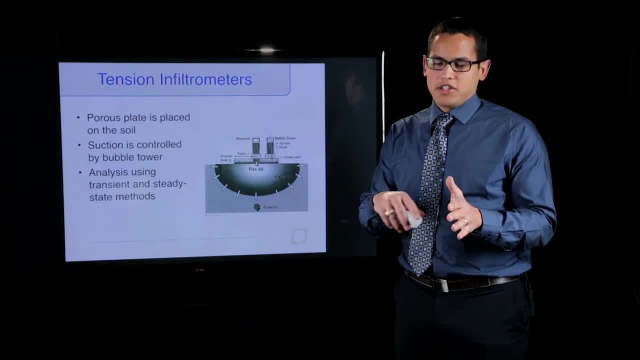 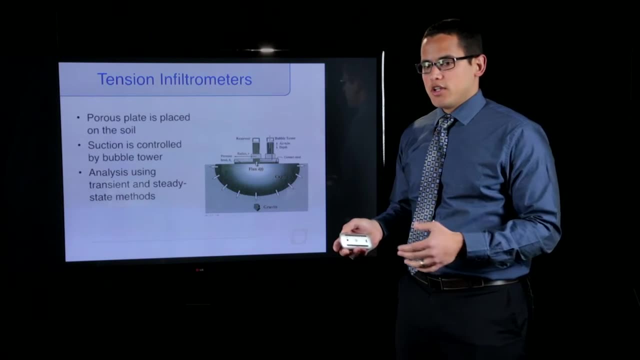 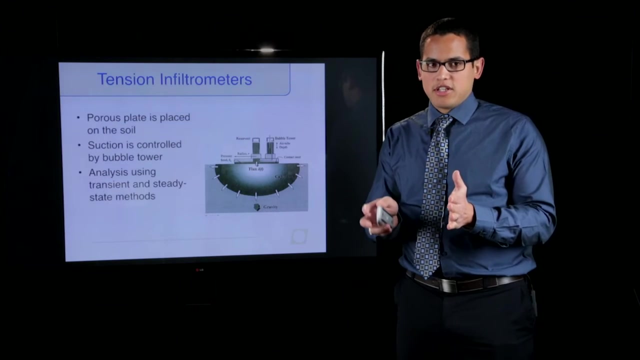 And there are analysis techniques to essentially extrapolate the data and get an estimation of the unsaturated hydraulic conductivity for that imposed suction. The other is the steady state method, where you actually do this for a set amount of time until you actually reach steady state infiltration rates. 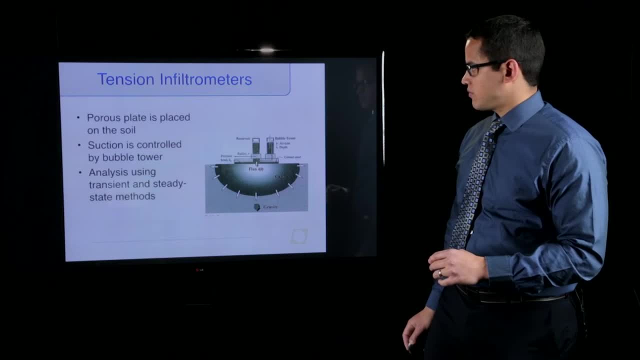 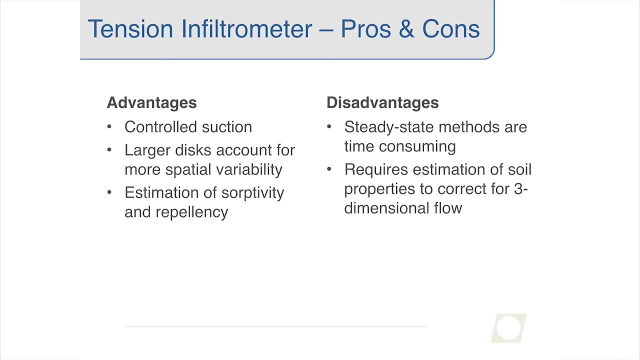 This technique, of course, is going to take more time. So some of the advantages and disadvantages of tension infiltrometers. One of the advantages with the tension infiltrometer is it is a controlled suction So you can set. okay, I want to get unsaturated hydraulic conductivity. 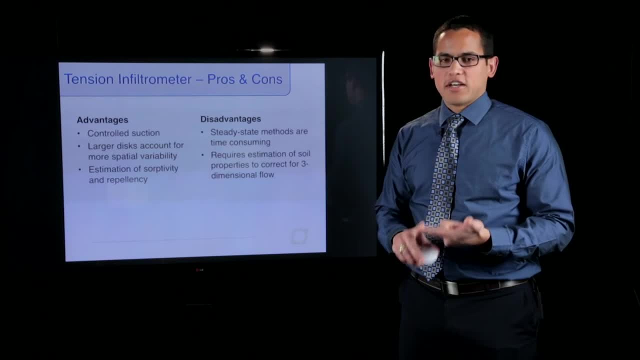 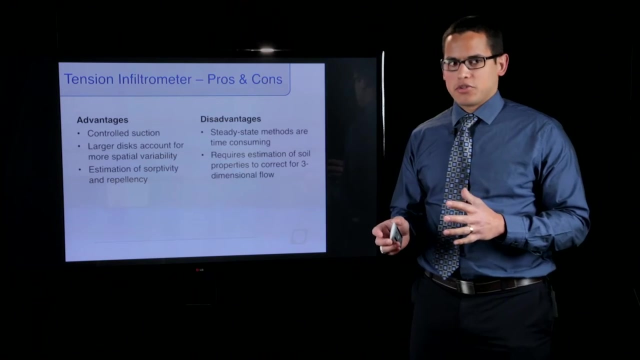 at this major potential. So I'll set it to say five centimeters of suction. Larger disks can account for more spatial variability- Now one of the things to kind of point out on that as you get further away from saturation. you actually get less of an effect on macropores or less of an effect of macropores on hydraulic conductivity, And that actually removes a lot of the sources for spatial variability. Research has shown that there is less spatial variability associated with unsaturated hydraulic conductivity. 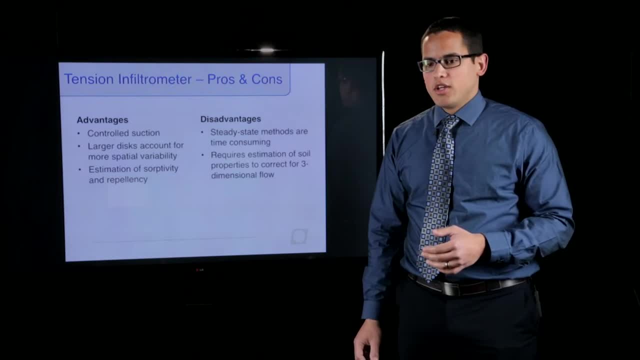 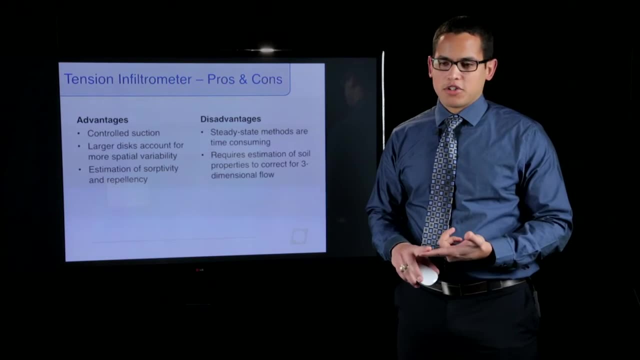 Not that it's not there, but there is a little less associated with this measurement, And you can also get an estimation of sorptivity and repellency with this technique, which is useful when doing hydrophobicity studies and post-force-fire studies. 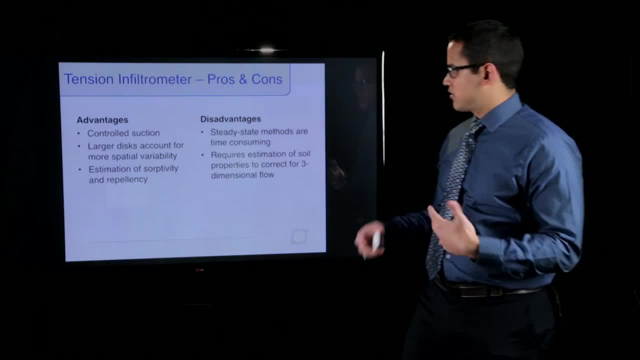 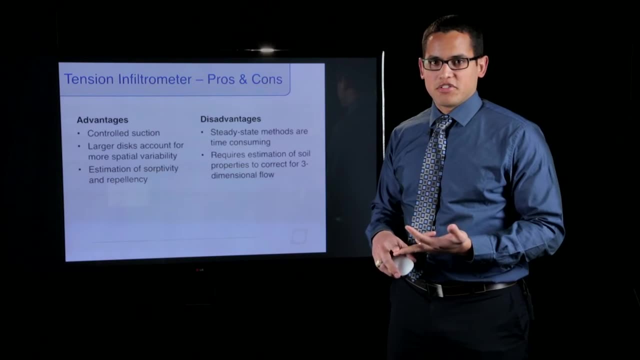 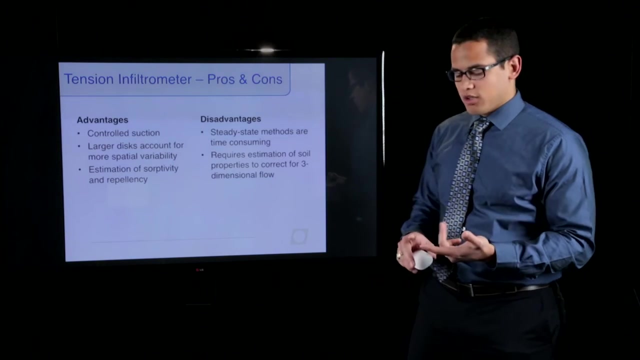 Some of the disadvantages with this technique is the steady state methods are time-consuming, just like they are when trying to reach steady state in a ring infiltrometer or a borehole permeometer. It does take time. When doing the transient technique, there is a possible for some inaccuracies. 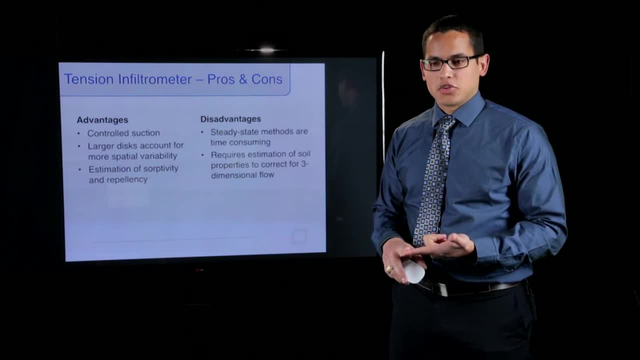 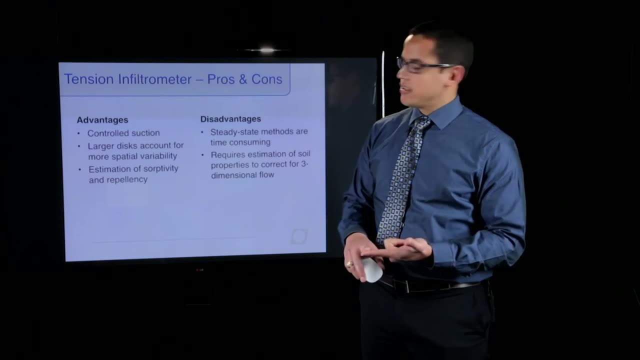 especially if you start with a very dry soil because you have a higher initial infiltration rate. So sometimes it's a good idea to make multiple measurements. if you do it using the transient technique And just like with a single ring infiltrometer, this requires an estimation of soil properties. 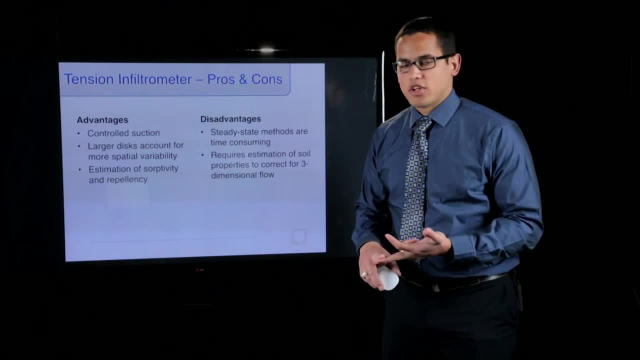 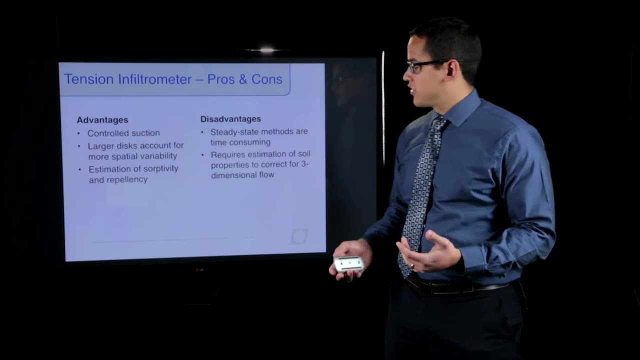 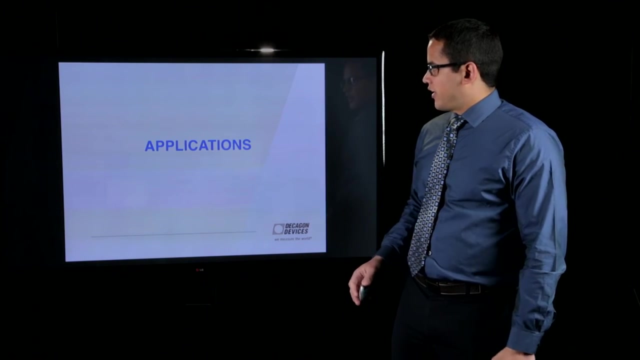 to correct for three-dimensional flow. So that's another disadvantage, another potential source for error. but this is a good technique for measuring unsaturated hydraulic conductivity in the field. All right, so now we're going to go on to just a couple applications of hydraulic conductivity. 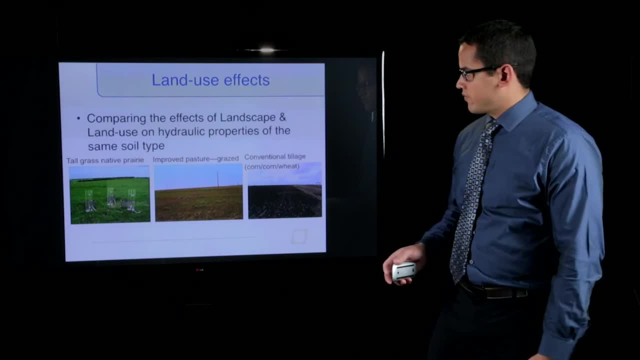 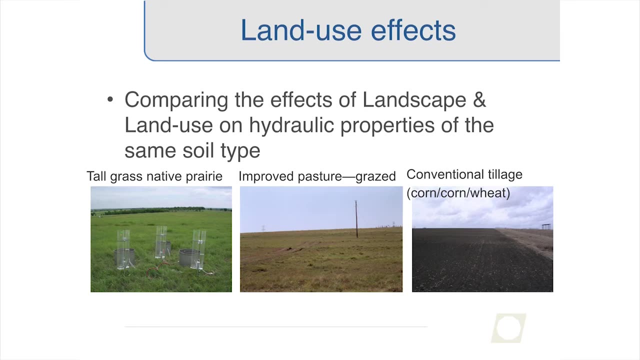 and where it's been useful. One of the reasons we commonly use hydraulic conductivity measurements is to compare land-use effects on hydraulic properties of soils, And this is something that's typical. that a lot of hydropedologists are doing is looking at either land-use effects 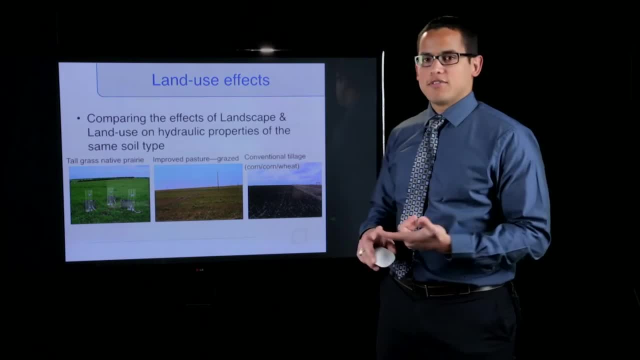 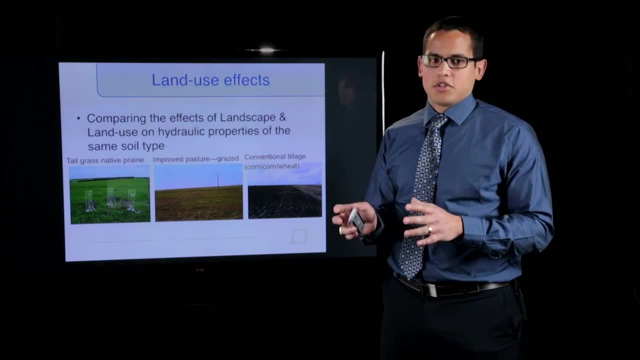 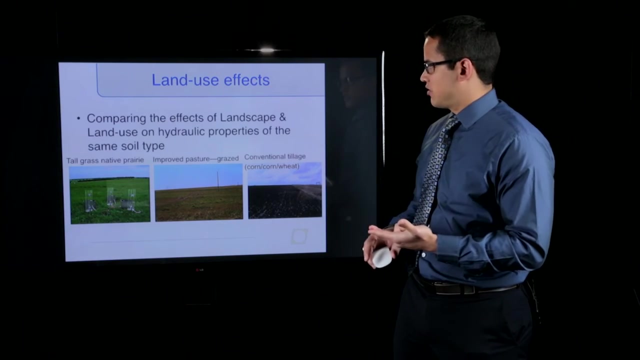 or landscape effects on hydraulic conductivity in that same soil type, Because it's often assumed: okay, I have this soil type, then I can use this hydraulic conductivity value. But it's often the case that the case is not true, especially when under different land uses. 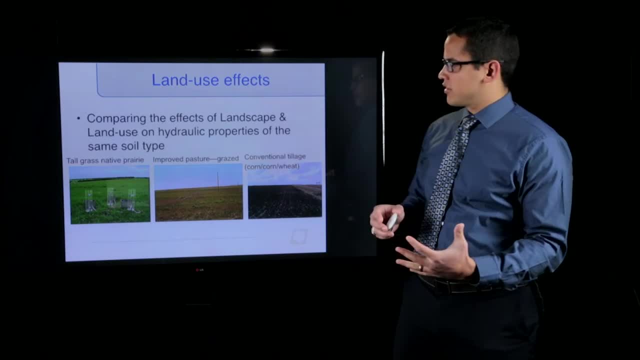 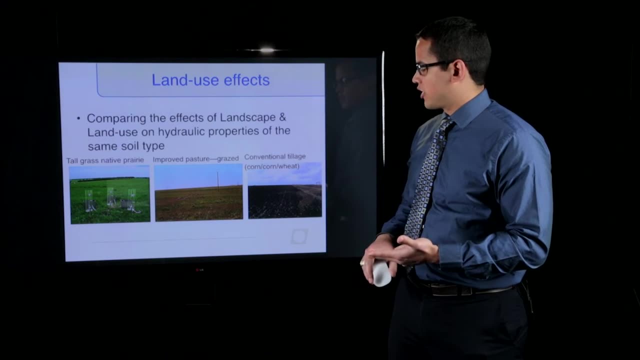 and landscape positions. And so here's an example, Some research that I've done in the past looking at hydraulic property changes in the black lands of Texas, looking at the vertisols, And this was actually a site where we had tall grass, native prairie site. 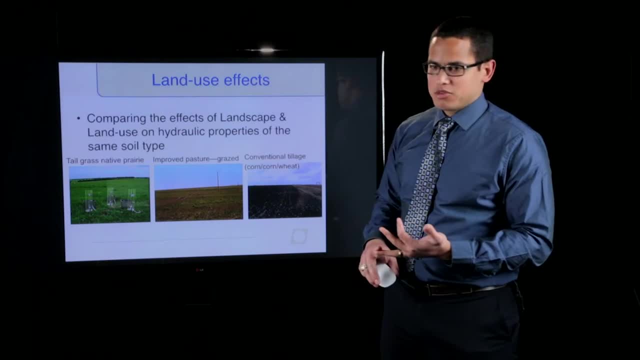 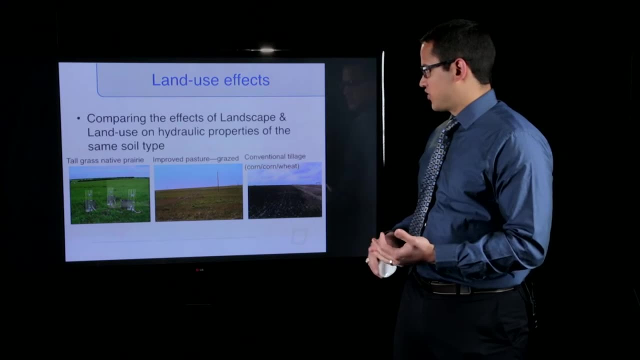 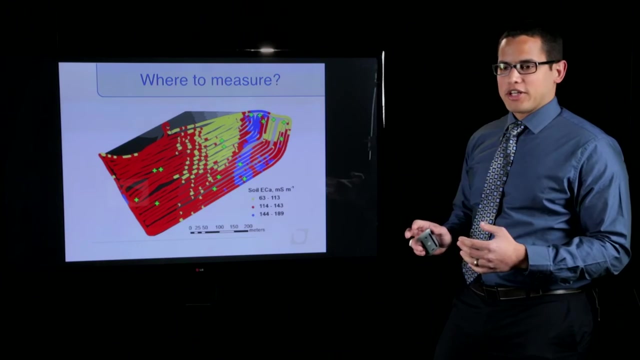 an improved pasture and a conventional tillage that looked just the same soil type, And we also had a strong change in landscape position across all three fields. And so another really interesting thing that I kind of want to point out is one of the common questions that we get is: 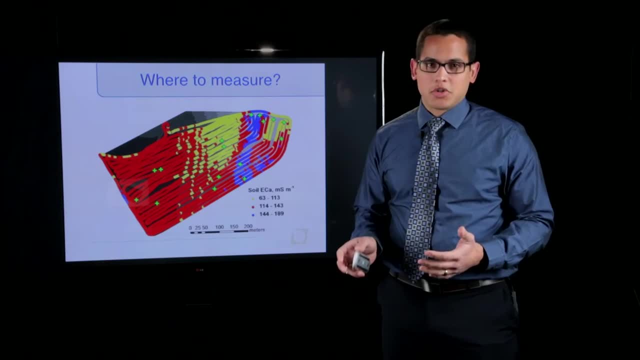 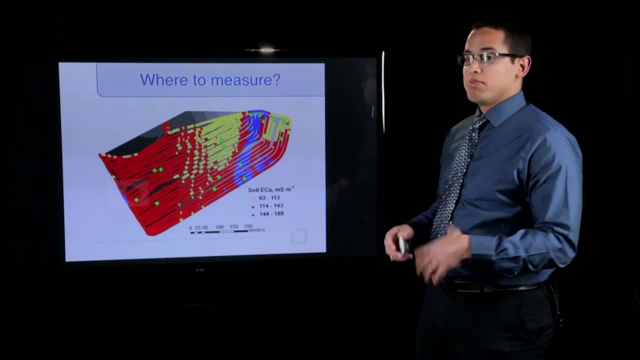 where do I need to make my measurement or how many measurements do I need to make and those types of things. And one of the tools that we've actually used in the past is a measurement of bulky sea across a field to try and get an estimation of the actual variability. 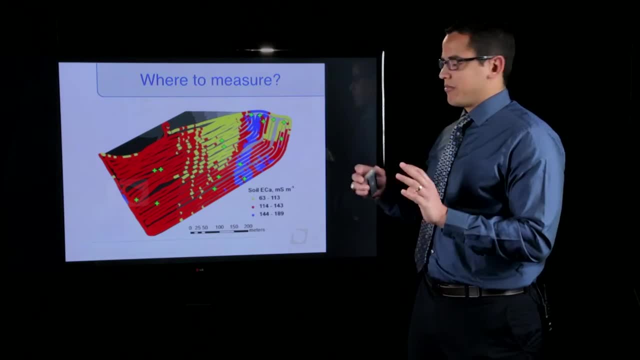 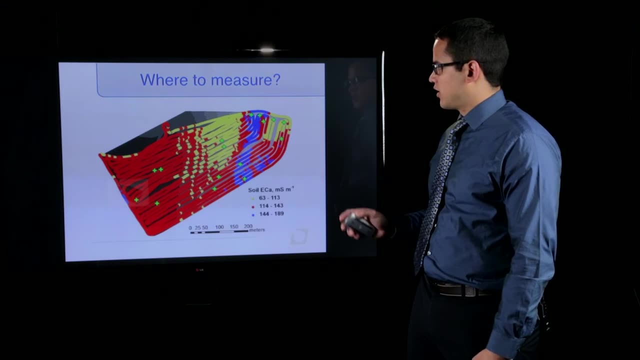 that's in the field, to then make decisions on where to make measurements and how many measurements we actually want to make to encompass the spatial variability of the field. And this is an example from one of the fields that we made these measurements on down in Texas. 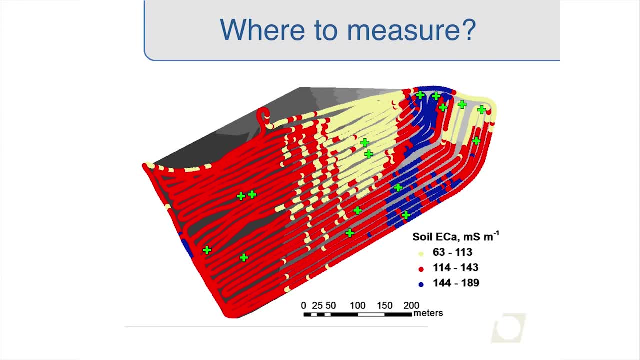 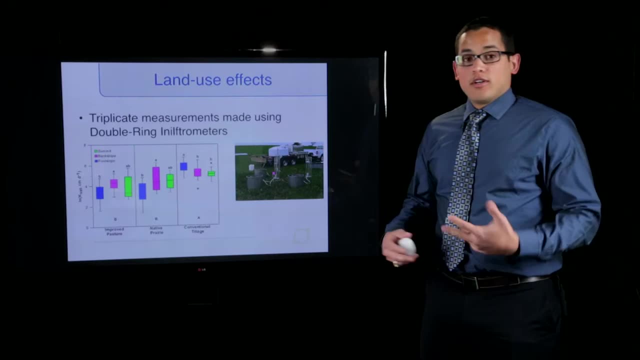 And these EC maps were generated using an EM38 device to measure the bulky sea, And then we were able to separate it into different sections and then decide where we wanted to make our measurements and how many measurements we actually wanted to make. So what we did with this project was again: 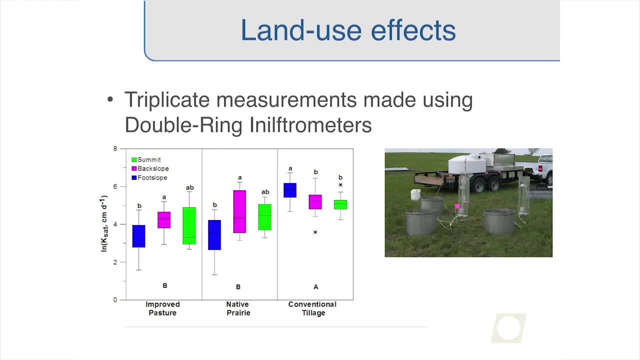 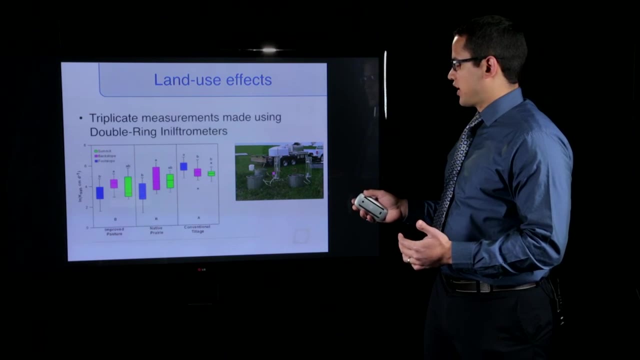 we were looking at land use effects And we made triplicate measurements of field saturated hydraulic conductivity using double ring infiltrometers at each of the points that we had selected, And so if we had, say, 10 points selected, we made 30 measurements in this field. 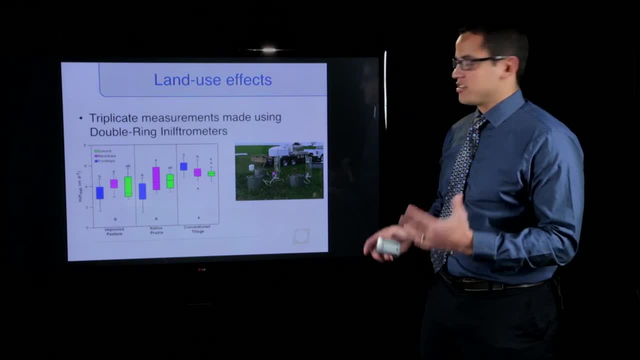 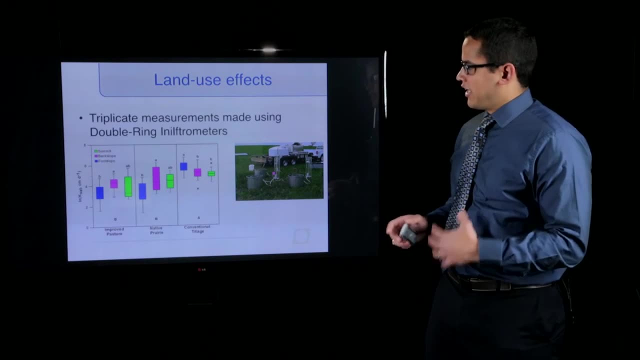 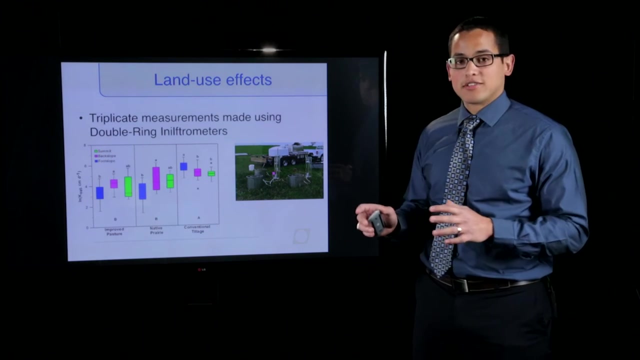 So what we did was compare the measurements across the different land uses and across the different landscape positions within each of these fields, And one of the really interesting things that came out of this is what we found when looking at the differences in landscape positions across the improved pasture. 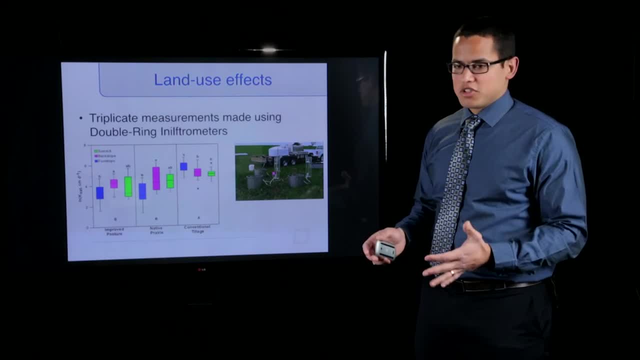 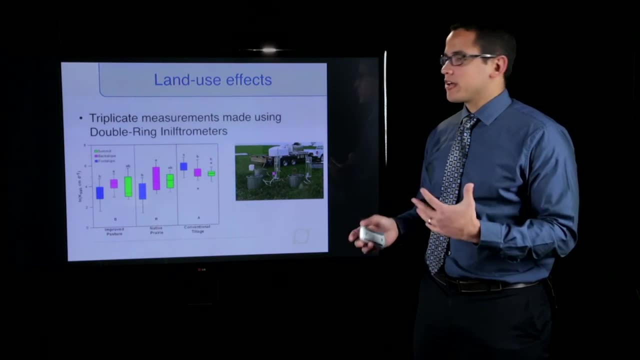 and the native prairie site, which are undisturbed soils because they're not tilled. Obviously, the improved pasture is grazed, so it is imposed a higher compaction and higher bulk densities than the native prairie. And then there are some vegetation differences. 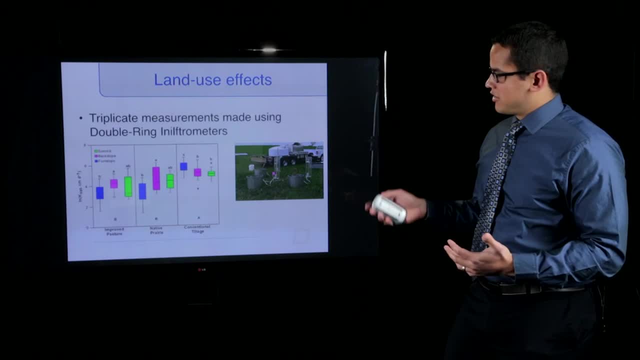 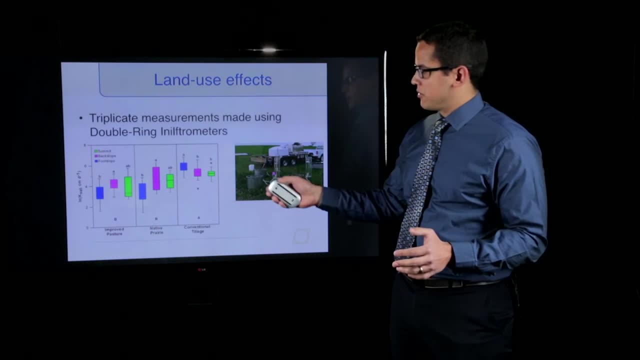 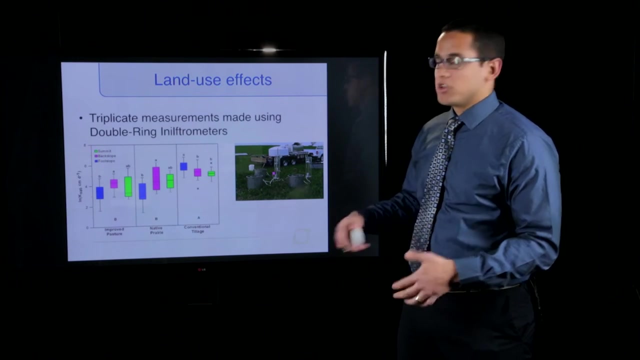 between the two, But what was really interesting is in both fields- and these fields are separated- we found the same trends across the summit: the backslope and the footslope, where typically we had higher hydraulic conductivity values in the backslope and then the lowest hydraulic conductivity. 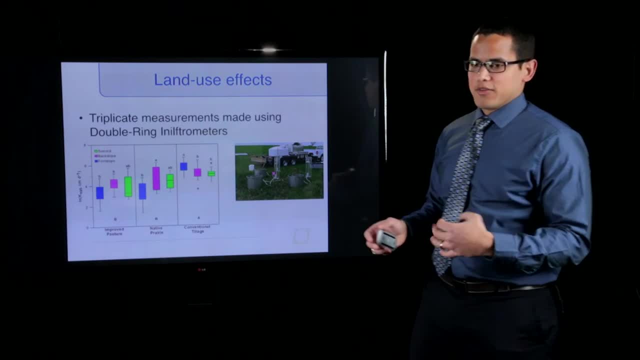 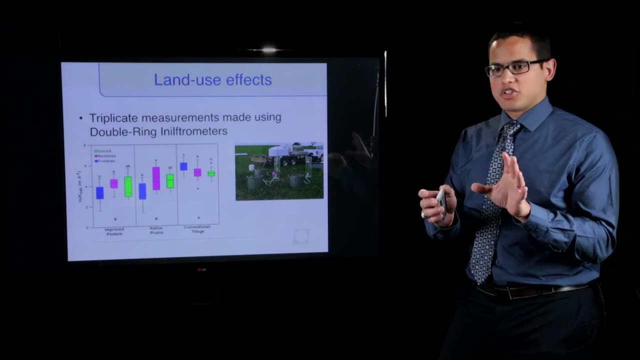 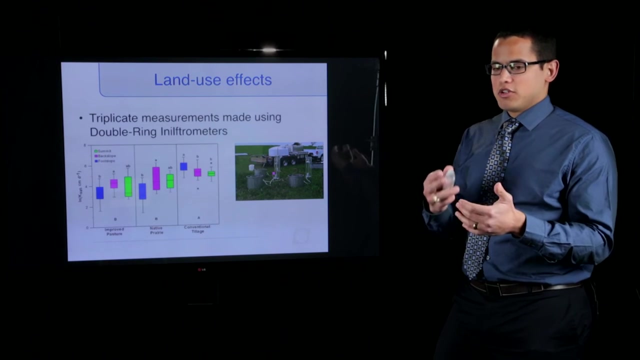 values in the footslope of each of these positions, And this is partially due to the Katina effect, where you have different changes in the hydraulic properties and the actual kind of chemical makeup of the soil due to solute leaching from the summit and precipitation of solutes in the footslope. 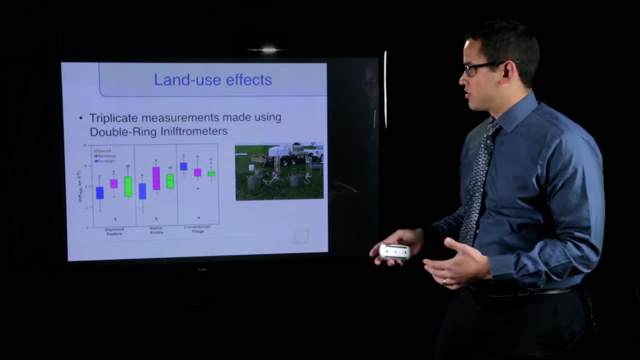 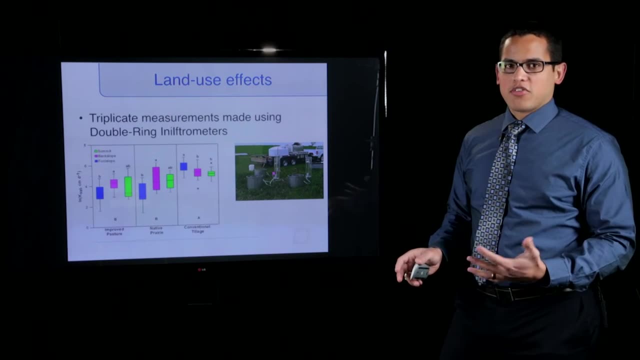 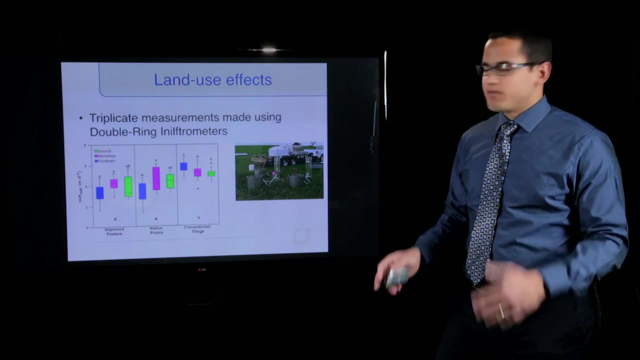 which then does cause some changes in the properties of the soil. And what was interesting is that this trend was not evident in the conventional tillage site, likely due to the fact that this site is being disturbed and tilled very regularly. And so just kind of an interesting use. 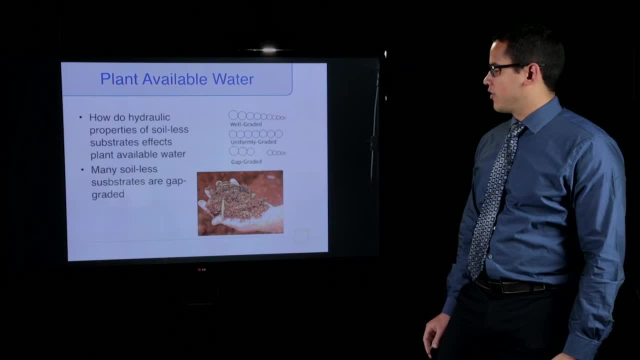 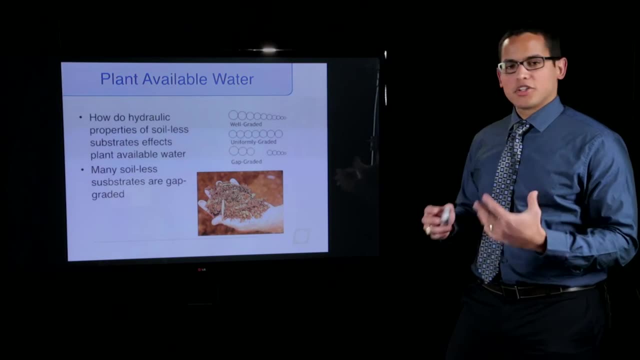 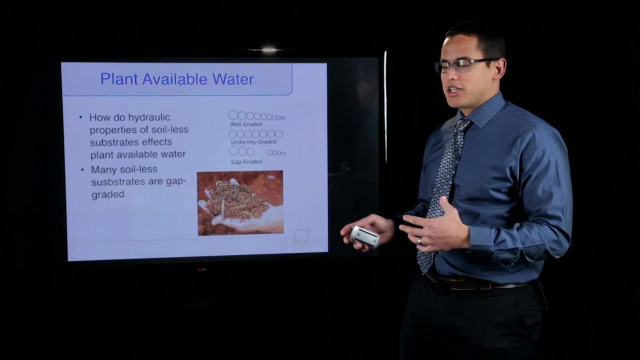 of hydraulic conductivity. Now, one of the more interesting ones for me that we've been recently looking at is: can hydraulic conductivity affect plant-available water? And what's going on right now is there are a lot of researchers looking at how do hydraulic properties of soil-less substrates 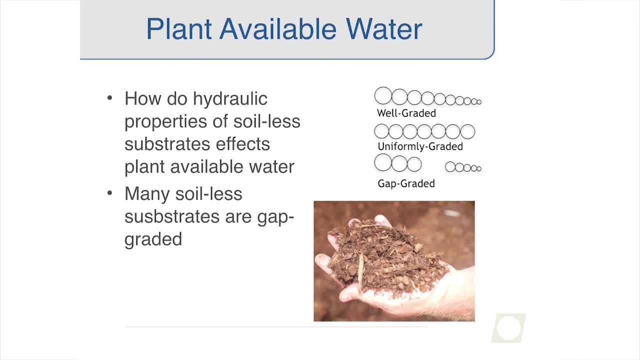 affect plant-available water. Typically, what most people look at is the soil-water retention curve and then they use that to determine what the actual plant-available water is in that range. But one of the things to consider is a lot of soil-less substrates are gap-graded. 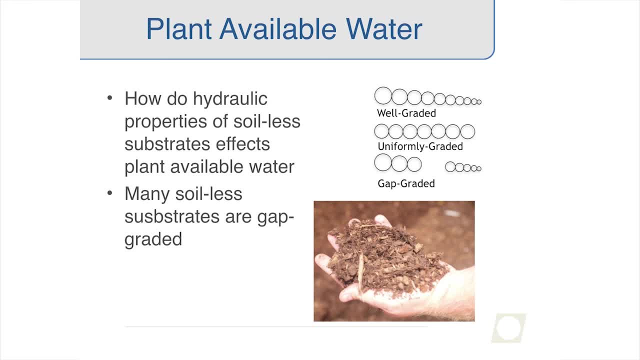 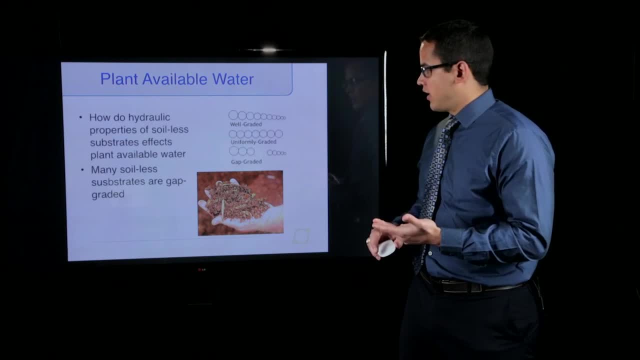 so we have substrates based from bark and substrates based from crushed brick that are used in green roofs and those types of things, And so what happens is we get very small pores inside of the materials themselves, like, for example, inside of the bark. 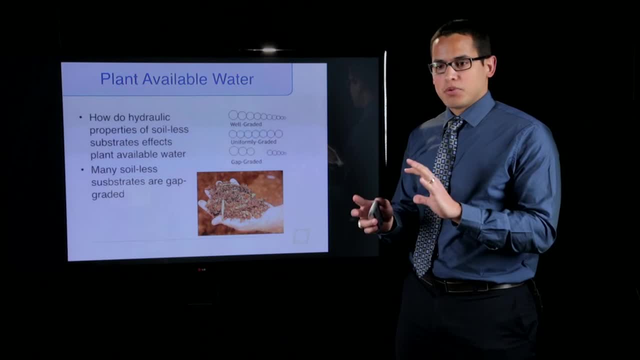 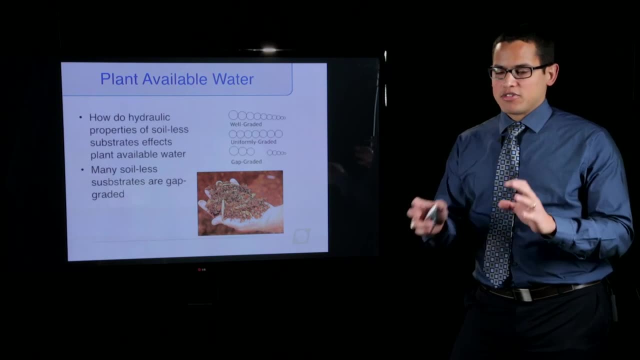 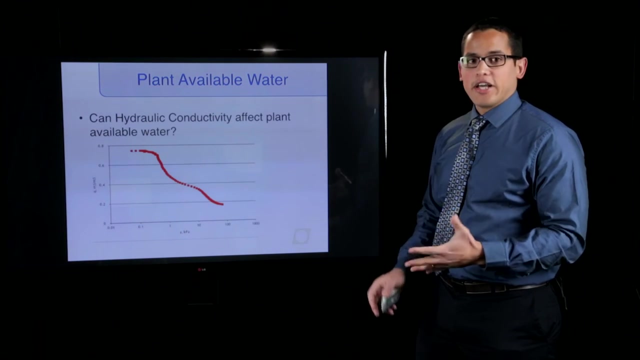 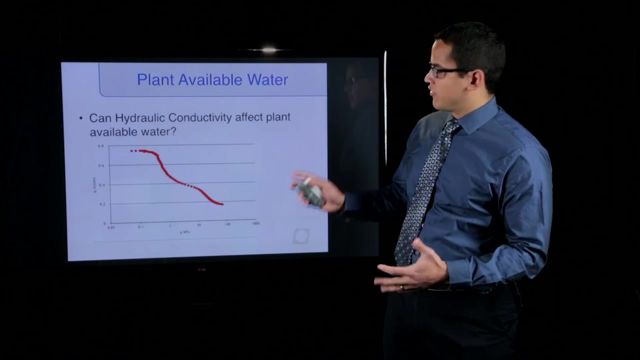 or inside of the crushed brick, and then we get larger pores around that, but we don't have these intermediate pores that help establish contact between the range of the pores, And so that's very evident when looking at the soil moisture release curve of these different soil-less substrates. 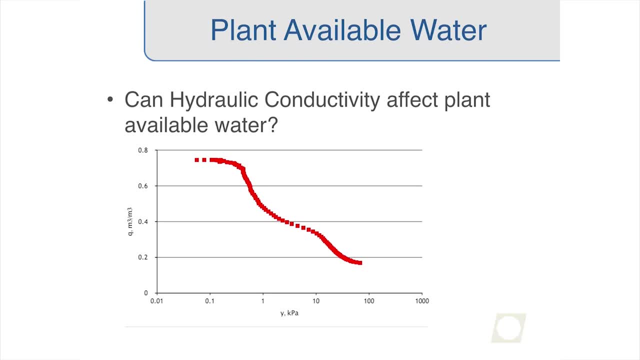 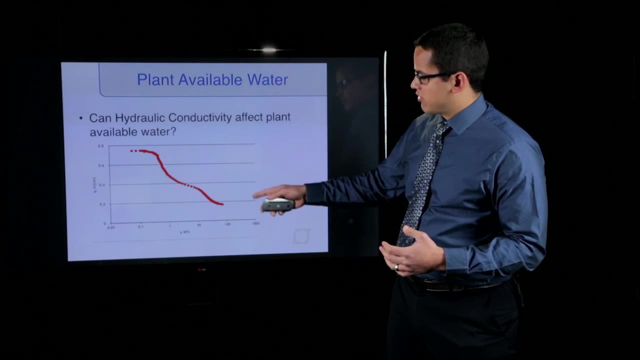 So here is a retention curve for what we call the McCorkle sample. This is actually a bark-based, soil-less substrate, And what happens is we get this bimodal release curve, and that's typical with gap-graded substrates. And so, because we have this gap-graded situation,